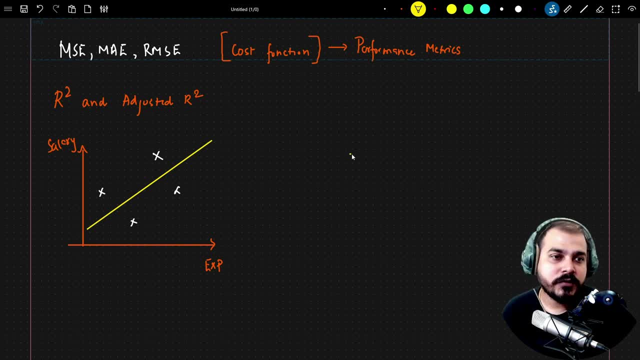 you know, in the linear regression I have also intuitively explained you about a concept of gradient descent And this gradient descent, the main aim is- and this was my cost function- theta zero comma, theta one, And this was my theta zero coefficients. in short. 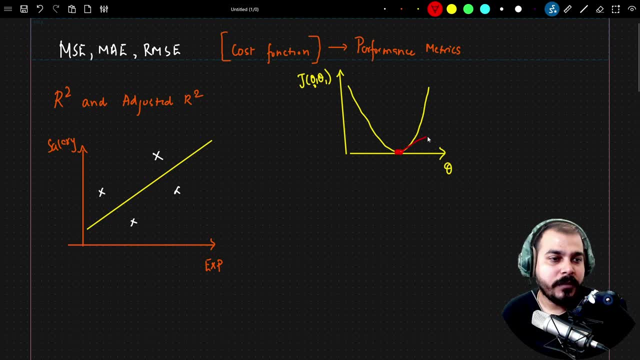 Our main aim was to basically come to this particular global minima. So this is basically where my global minima and I have to come over here right And how I'm going to come. I have to continuously change this theta value, find out the derivative and try to come. 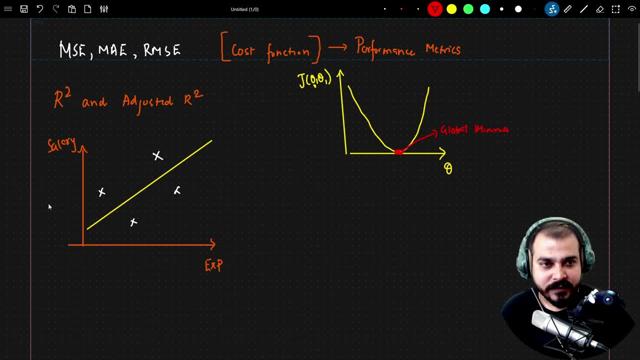 over here right Now. let's go ahead and see that if I have this specific use case over here, you know that. let's say: this is my data set- experience and salary. right, I will obviously be having some values right now over here. Now, this salary is nothing but my y variable. 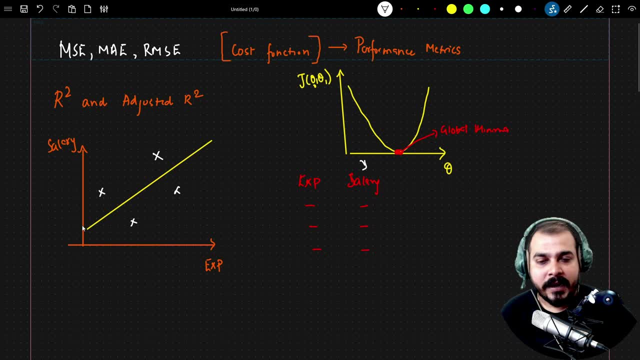 that is my truth variable, which is denoted by this white column, And this best fit line, which is basically created, actually help us to find out the predicted data points, right? So here, with respect to this particular data point, this is my predicted data point. with respect to this, this is my 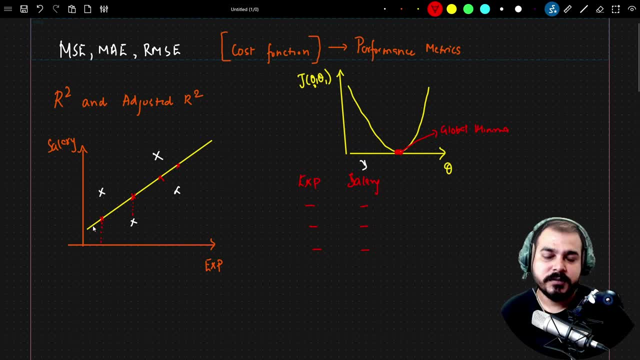 predicted data point. it is: this is my predicted data point and this is my predicted data point. So what we do? we basically calculate the error like this, And our main aim is to reduce the specific error. And in order to reduce the specific error, we use different, different. 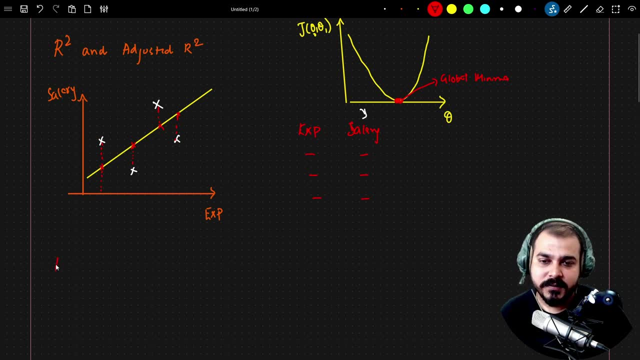 cost function. the first cost function that we used is basically called as mean squared error. now let me go ahead and write this formula: mean squared error is nothing but summation of i is equal to 1 to n. y minus y hat. y hat is the predicted output, whole square divided by n. 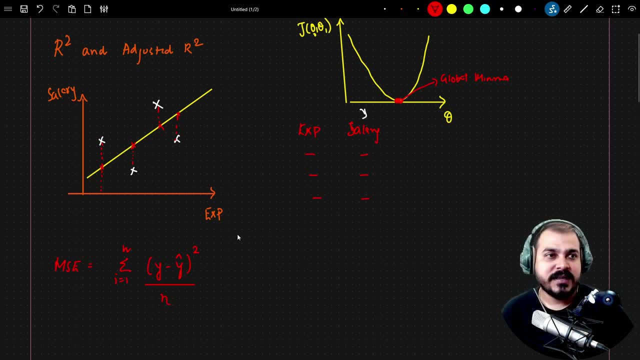 right. n is the total number of data points and this is the same cost function that we used to basically create this gradient descent. now, what is so important about this cost function? and our main aim is to reduce this cost function, because this is specifically talking about the error and 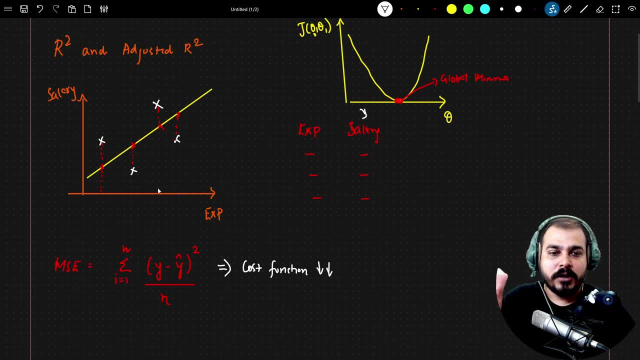 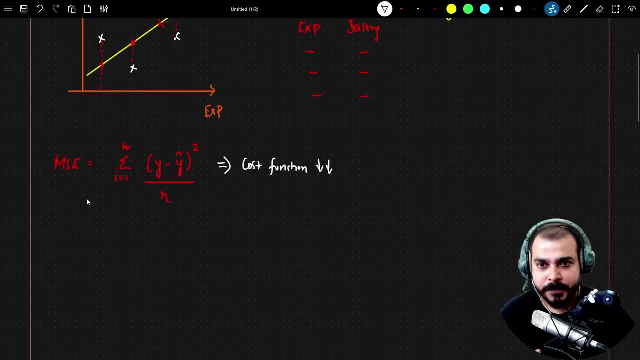 our best fit line should be created in such a way that our cost function should keep on reducing. okay, so we can also use this as a parameter to check how our model is basically performing. okay, now, in mean squared error here. we are just trying to calculate the error, right. so y y minus y hat. 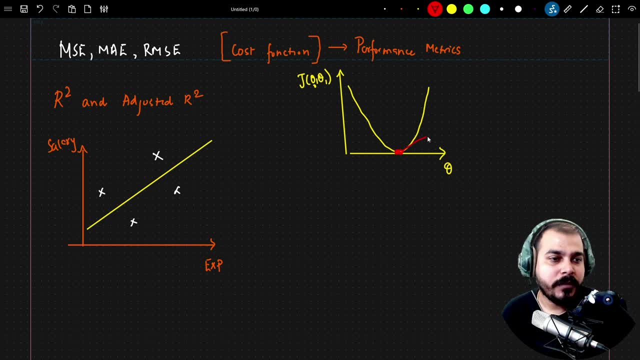 Our main aim was to basically come to this particular global minima. So this is basically where my global minima and I have to come over here right And how I'm going to come. I have to continuously change this theta value, find out the derivative and try to come. 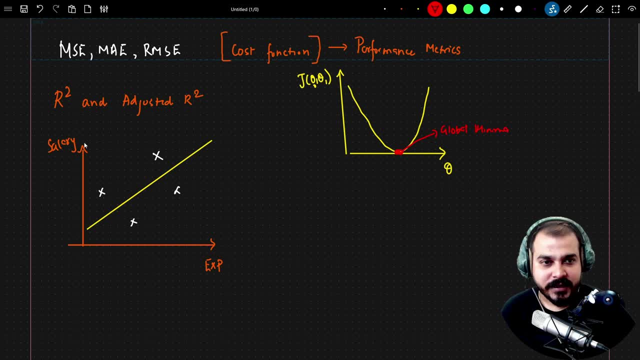 over here right Now. let's go ahead and see that if I have this specific use case over here, you know that. let's say: this is my data set: experience and salary. right, I will obviously be having some values right now over here. Now, this salary is nothing but my y variable. That is my truth. 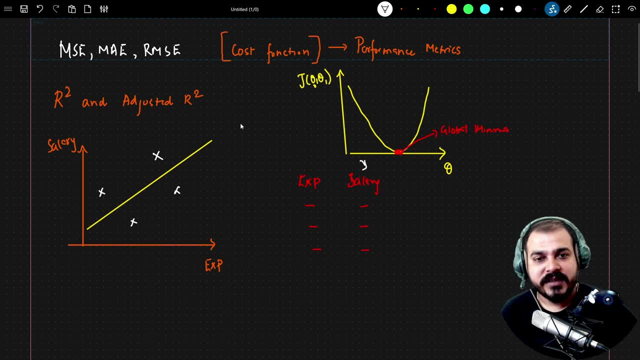 variable, which is denoted by this white color And this best fit line, which is basically created, which will actually help us to find out the predicted data points, right? So here, with respect to this particular data point, this is my predicted data point With respect to this. 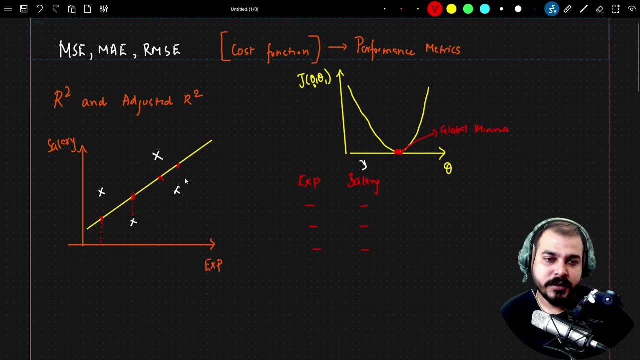 this is my predicted data point. It is: this is my predicted data point and this is my predicted data point. So what we do? we basically calculate the error like this, And our main aim is to reduce the specific error. And in order to reduce the specific error, we use different, different cost. 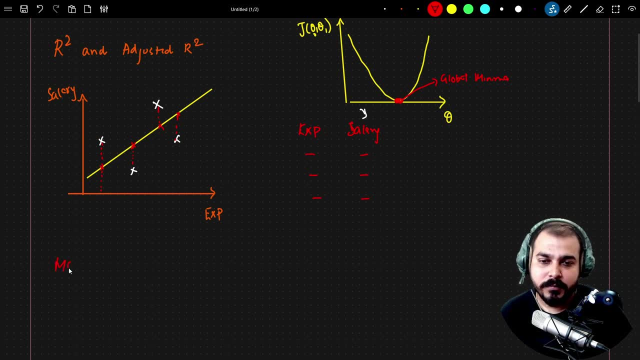 function, The first cost function that we used, is basically called as mean squared error. Now let me go ahead and write this formula: Mean squared error is nothing but summation of r is equal to one to n y minus y hat. Y hat is the predicted output, whole square divided by n. 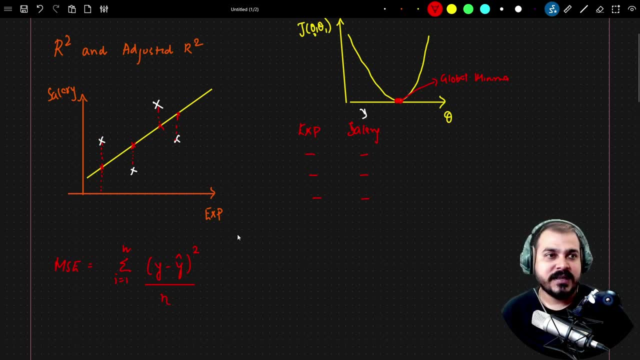 Right. N is the total number of data points, And this is the same cost function that we used to basically create this gradient descent. Now, what is so important about this cost function? And our main aim is to reduce this cost function, because this is specifically talking about the 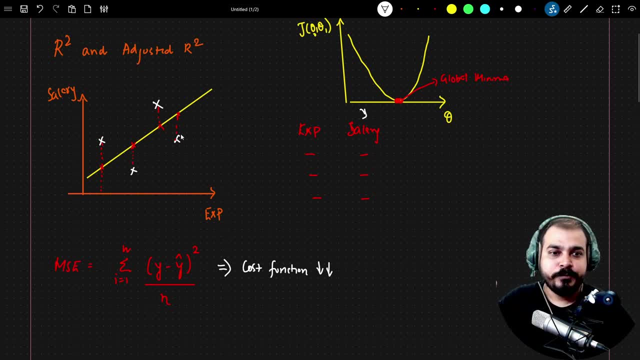 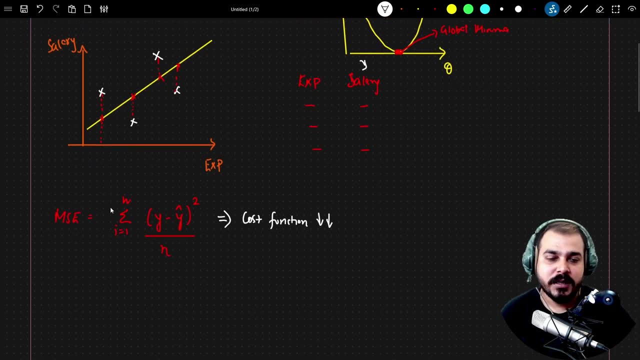 error- and this is specifically talking about the error- and our best fit line should be created in such a way that our cost function should keep on reducing. okay, so we can also use this as a parameter to check how our model is basically performing. okay, now, in mean squared error here. 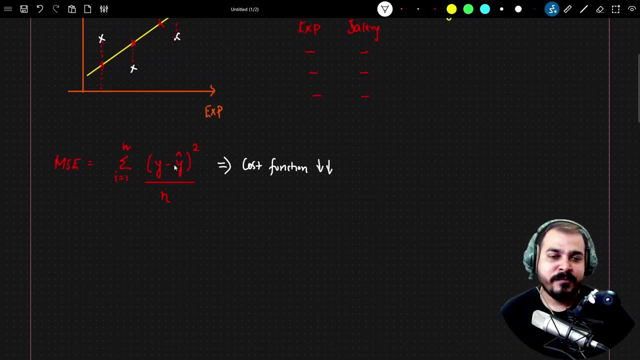 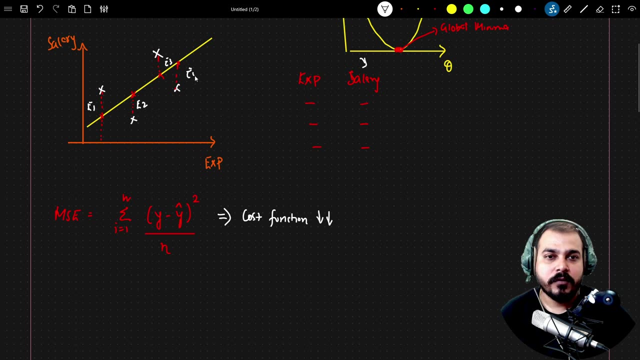 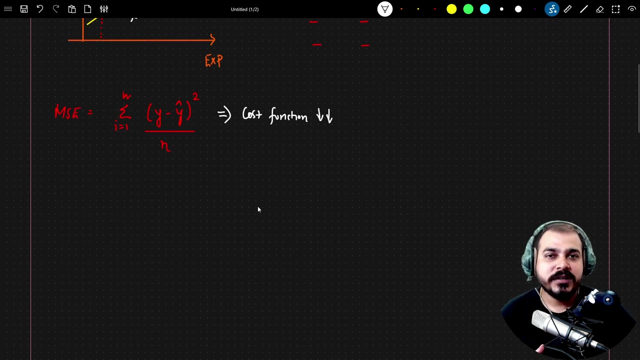 we are just trying to calculate the error, right? so y y y minus y hat. so we are going to add up this particular error. let's say i'm mentioning it as e1, e2, e3, e4, right, i'll add up all this particular error. now let's talk about the advantages of using msc and disadvantages of. 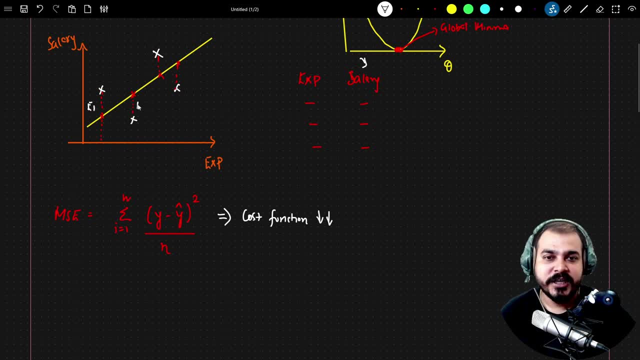 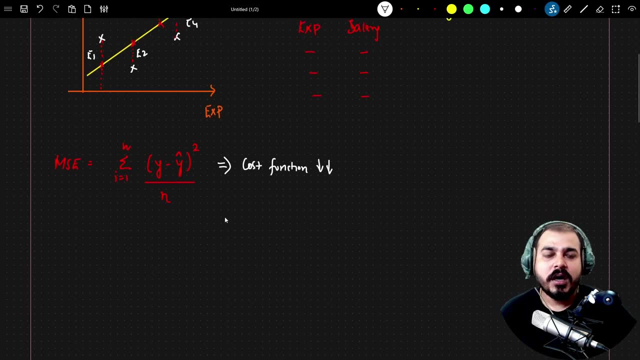 so we are going to add up this particular error. let's say, i'm mentioning it as e1, e2, e3, e4, right, i'll add up all this particular error. now let's talk about the advantages of using msc and disadvantages of using msc. now, first of all, from our previous intuition, we have already seen that 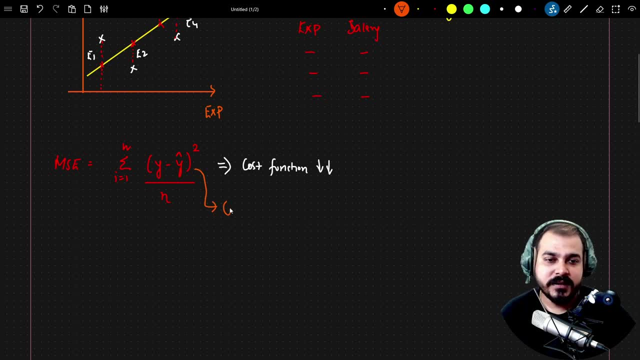 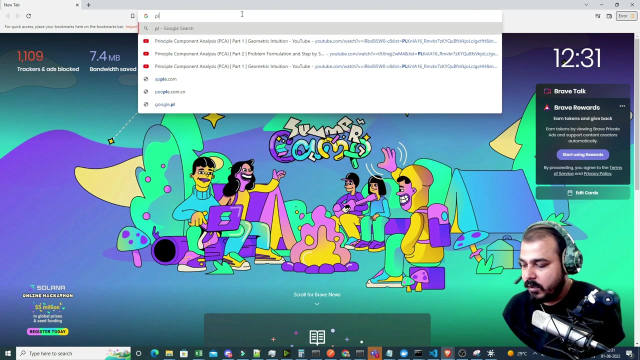 this: y minus y hat whole square. it is basically a quadratic equation. so if you don't know what is a quadratic equation, i would suggest just open a browser. let me just show you a quadratic equation how it looks like. so let's say, over here i'm just writing it out: plot. 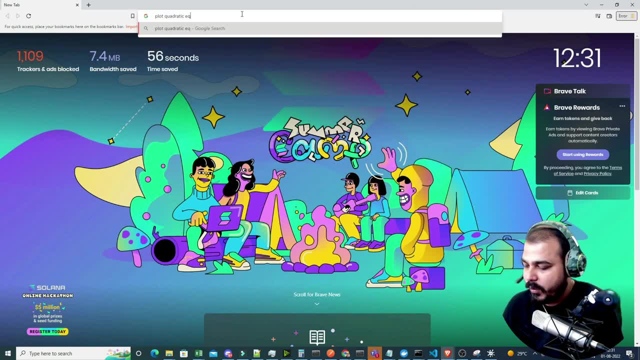 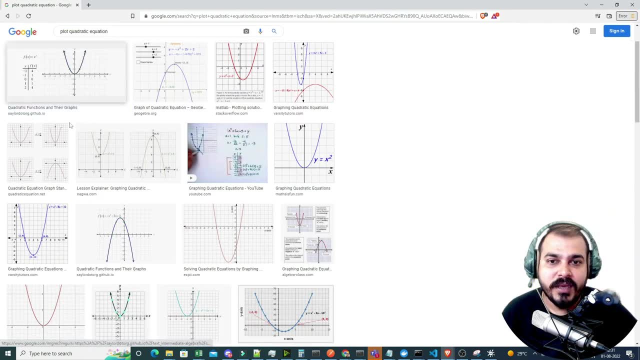 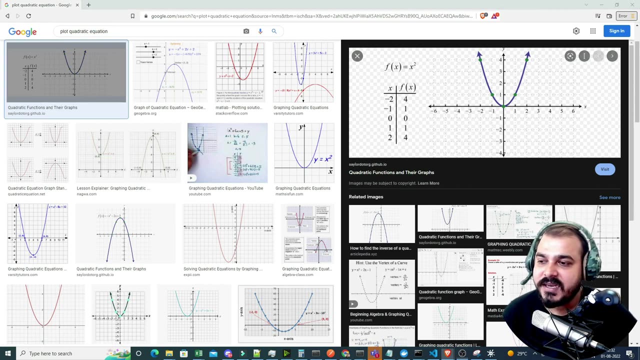 quadratic equation. okay, so when i plot this quadratic equation, if i probably go and see the images here, you'll be able to see we will be getting this kind of image right. and if you are getting this kind of image, you obviously know that this is basically a gradient descent, that 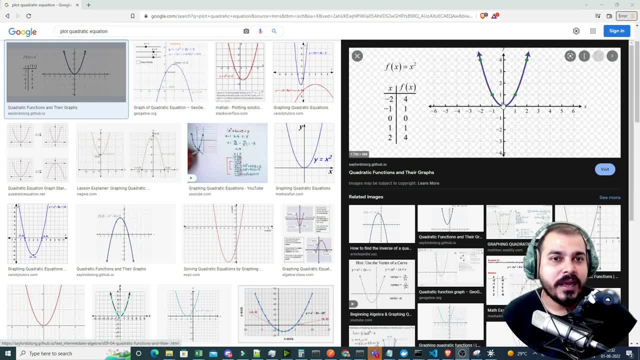 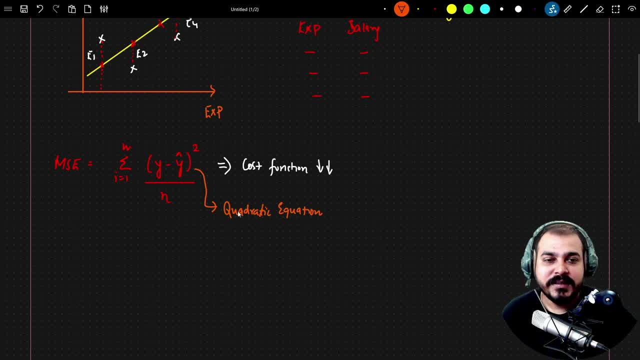 basically means we will be able to reach our global minima with the help of this quadratic equation. now why i say uh? now why i say this as a quadratic equation? because, understand, this is in the format of ax plus by plus c. right, because if i take this and if i write a minus b, whole square, it is nothing. 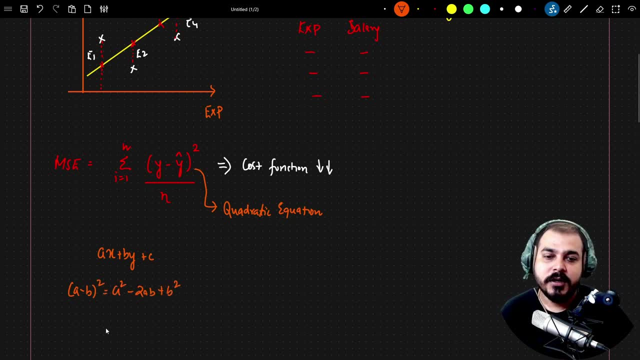 but a square minus 2ab plus b square right. so here it is basically a quadratic equation. and whenever you have a quadratic equation and if you plot this quadratic equation, in short, you will be getting a gradient descent. and remember one important point in gradient descent that you will be: 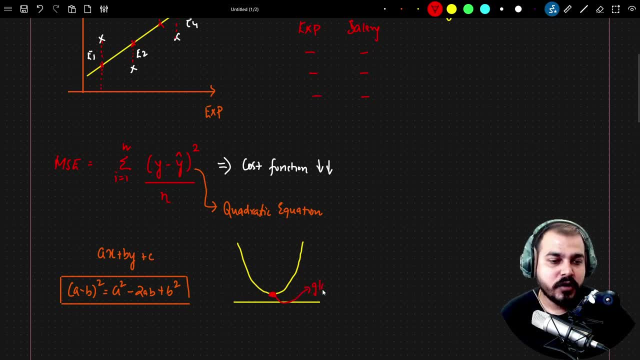 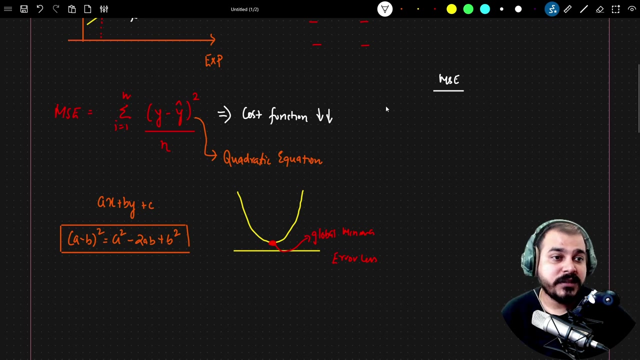 having a global minima, and our aim is basically to come to this global minima, or near to this global minima, because here the error will be less right. so this is the major, major advantage. so let me go ahead and write the advantages of using RMSE. sorry, mean squared error. so first, 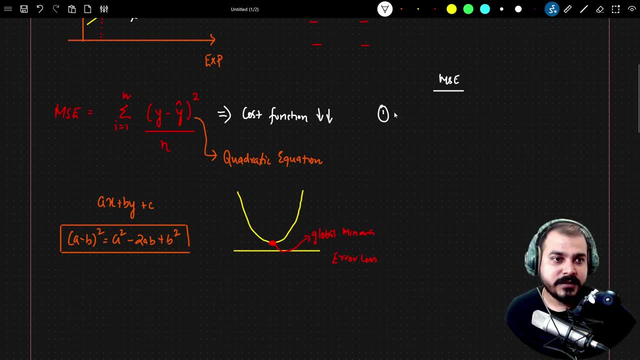 advantage is that, if I probably write this as advantage, let me go ahead. so, advantage and disadvantage, the first and the foremost advantage is that, and whenever we have this kind of gradient descent, one thing you need to know that it is differentiable at all point, and we also saw this right. it is. 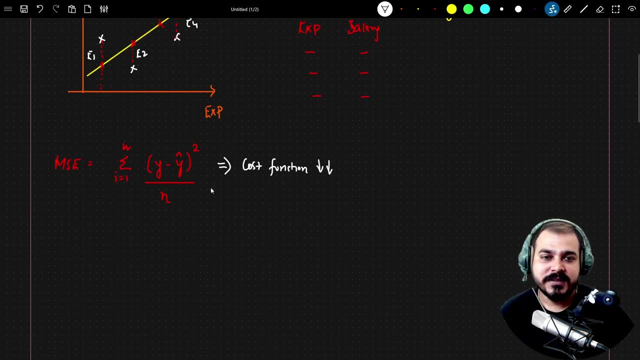 using msc now. first of all, from our previous intuition, we have already seen that this y minus y hat whole square. it is basically a quadratic equation. so if you don't know what is a quadratic equation, i would suggest just open a browser. let me just show you a quadratic. 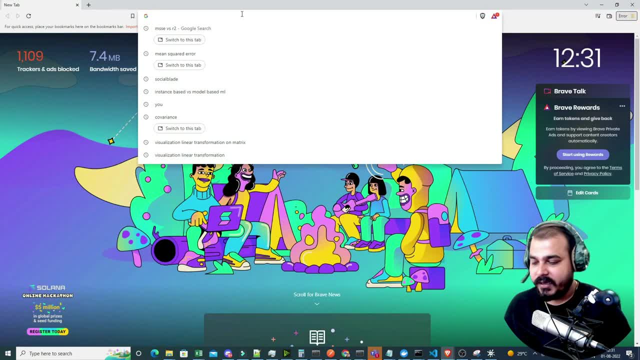 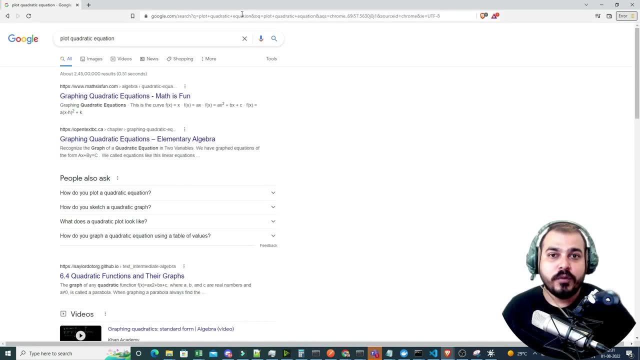 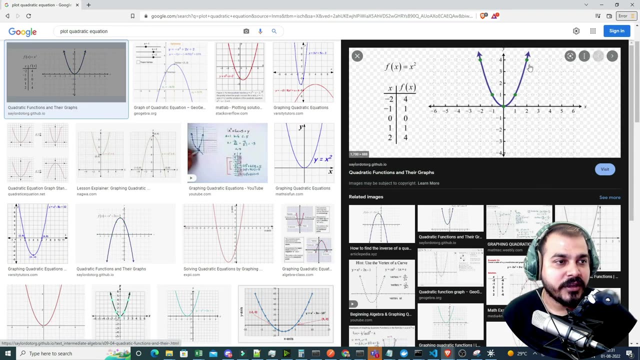 equation how it looks like. so let's say, over here i'm just writing it out, plot, plot, quadratic equation. okay, so when i plot this quadratic equation, if i probably go and see the images here, you'll be able to see we will be getting this kind of image right. and if we 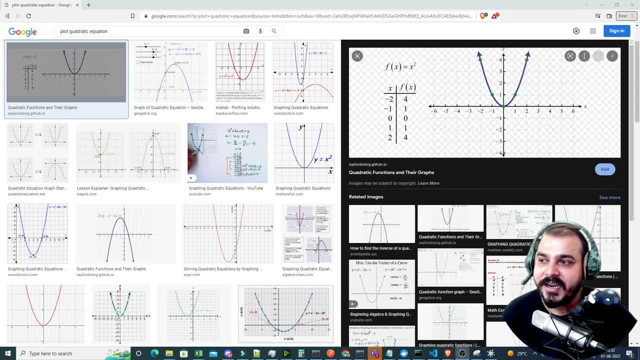 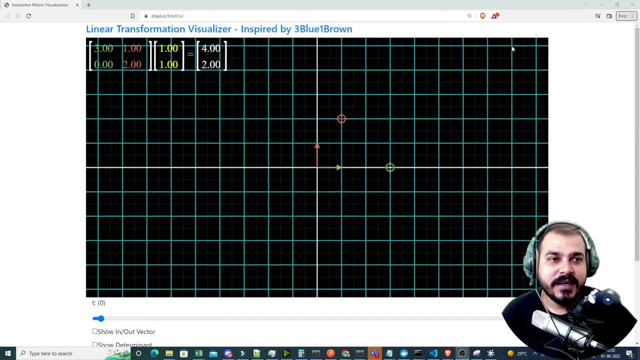 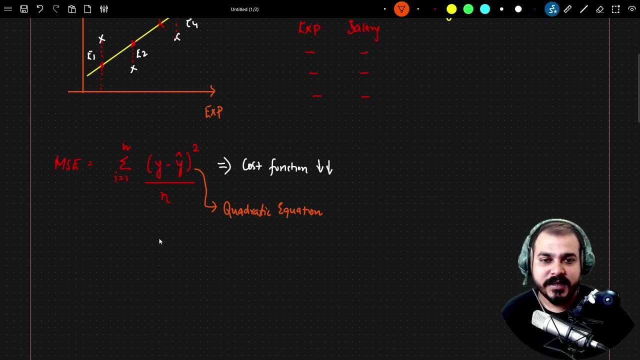 are getting this kind of image. you obviously know that this is basically a gradient descent. that basically means we will be able to reach our global minima with the help of this quadratic. now why i say uh? now why i say this as a quadratic equation? because, understand, this is in the format of ax plus by plus c. right, because if i take this and 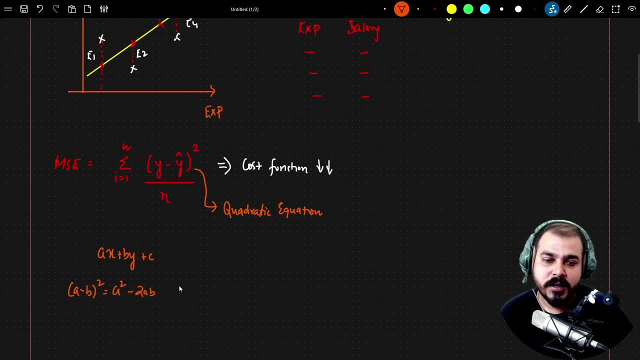 if i write a minus b, whole square, it is nothing but a square minus 2ab plus b square, right. so here it is basically a quadratic equation. and whenever you have a quadratic equation and if you plot this quadratic equation in short, you will be getting a gradient descent. and remember one important point: 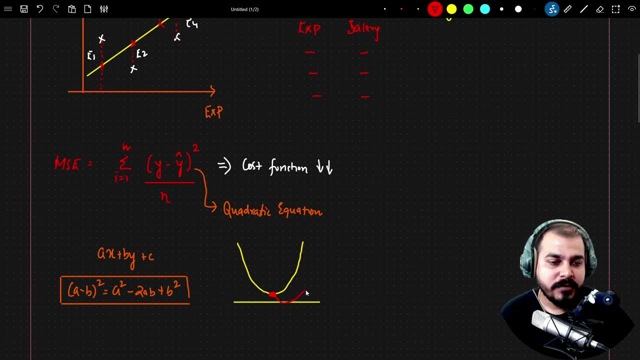 in gradient descent, that you will be having a global minima, and our aim is basically to come to this global minima, or near to this global minima, because here the error will be less right. so this is the major, major advantage. so let me go ahead and write the advantages of using rmse. 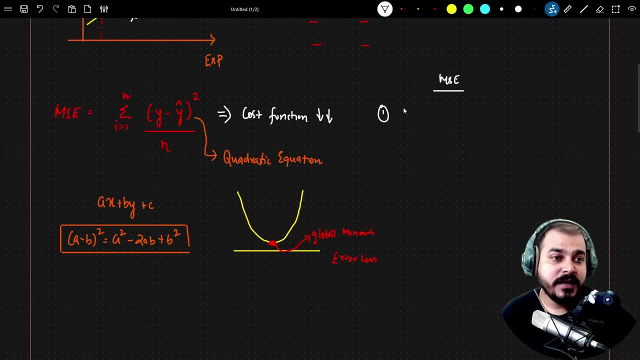 sorry, mean squared error. so first advantage is that. uh, if i probably write this as advantage, let me go ahead. so, advantage and disadvantage. the first and the foremost advantage is that, and whenever we have a global minima, we have a global minima, have this kind of gradient descent. one thing you need to know, that it is. 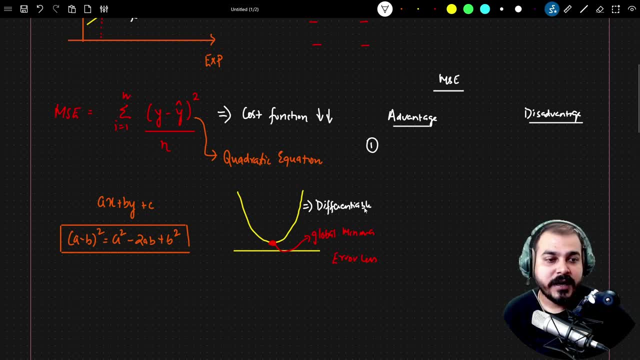 differentiable at all point, and we also saw this right. it is differentiable at all point. so first advantage is that it is differentiable. why it is differentiable? because it forms this kind of gradient descent curve, so at every point we will be able to calculate the slope and based on that we can 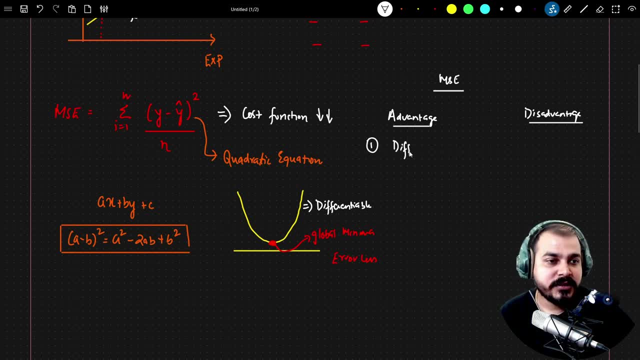 differentiable at all point. so first advantage is that it is differentiable. why it is differentiable? because it forms this kind of gradient, decent curve, so at every point we will be able to calculate the slope and based on that we can reduce the, we can reduce the coefficient and probably reach the global minima. 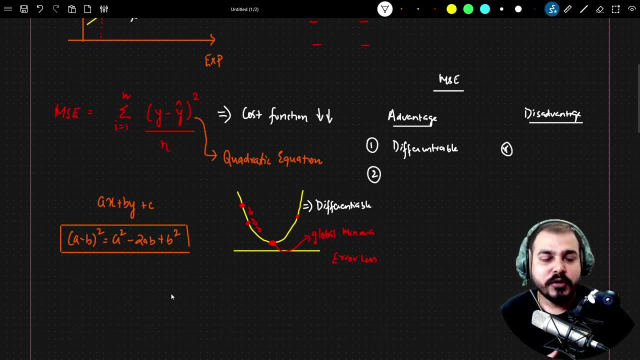 so most. a major advantage is that it is differentiable. coming to the next advantage is that over here, this kind of curve, it has one local and one global minima. this is super important point which everybody needs to focus on. right, let's say this particular gradient descent, that 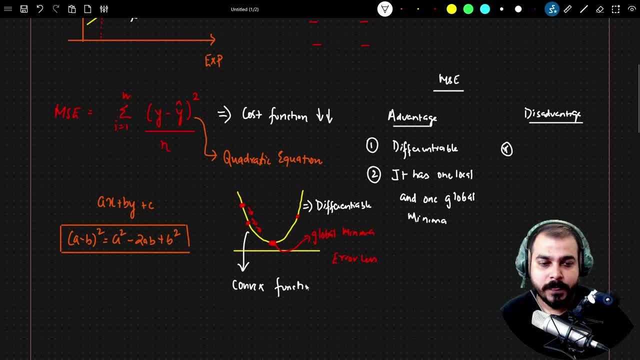 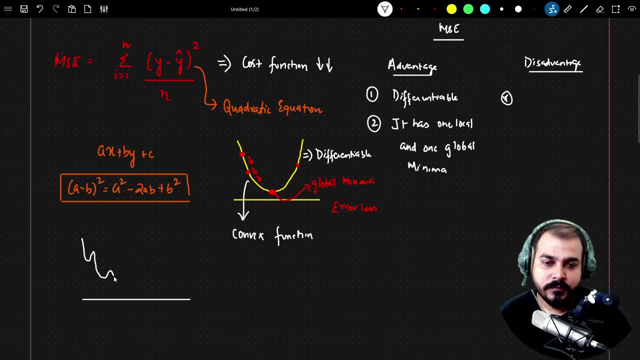 i see is basically a convex function. okay, if you see some of the curves, let's say that i have one curve like this and this gradient descent curve looks something like this. okay, now over here you can see that this is not a convex function. obviously, here you have one global minima and 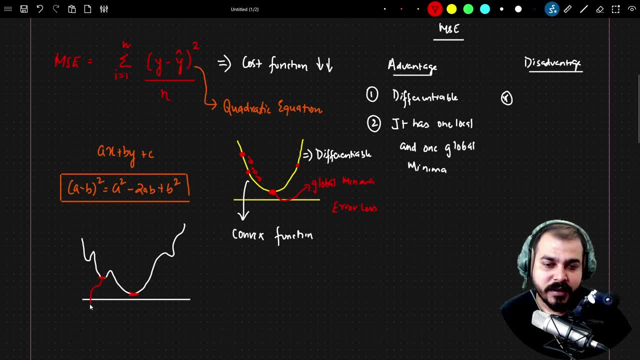 you'll also be seeing that you'll be having some more minimas, and this minima is basically called as local minima. if we use different types of equation, in those equation you'll be seeing that you'll be able to get- or if you plot these equations, you'll 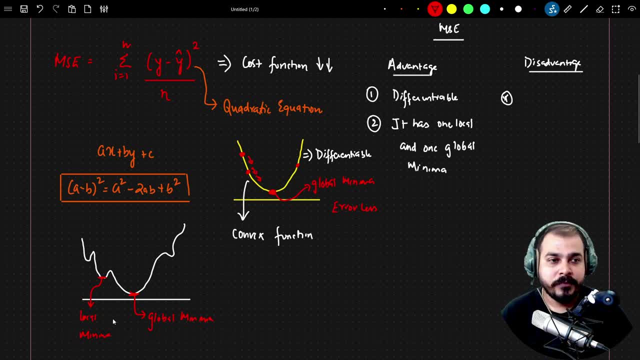 be. there'll be chances that you'll be getting both global minima and local minima, but since you're using this quadratic equation, you're plotting it, you will just be having one local or one global minima right, not multiple, because what will happen if you have some local minima, then your convergence? 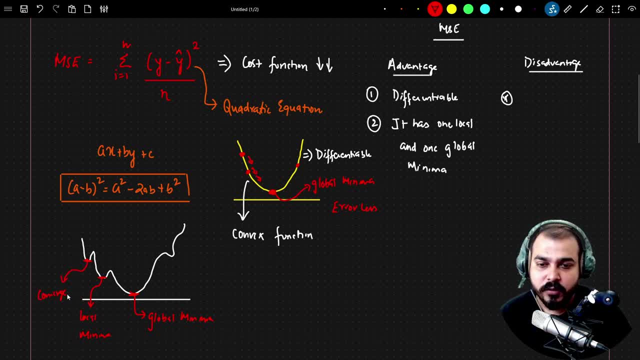 will get stuck over here. right, your convergence will get stuck over here because why? here the slope is actually equal to zero. this is a super important point to understand. what is the references between local minima and global minima? okay, if you have a local minima, that basically. 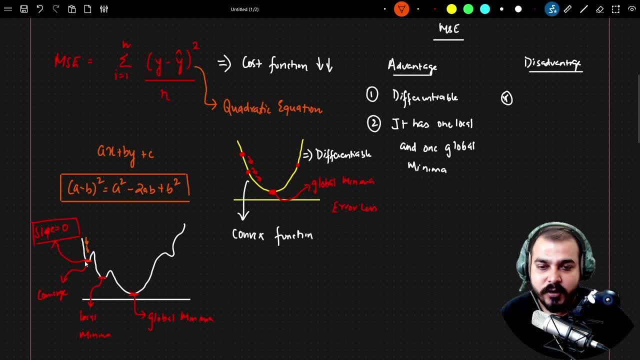 means your convergence. let's say your convergence is happening like this. it will go ahead and it will stop over here, because here your slope is zero, right, but in the real you really need to reach to the global minima, right. so if you use any different kind of equation, specifically not 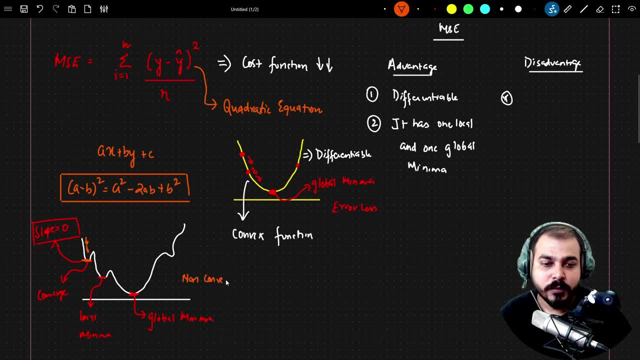 quadratic equation. there are also some equation which is basically called as non-convex equation or non-convex functions. in this particular case, you will be seeing that they will be having both local minima and global minima, but currently we are using this quadratic equation, that is y minus. 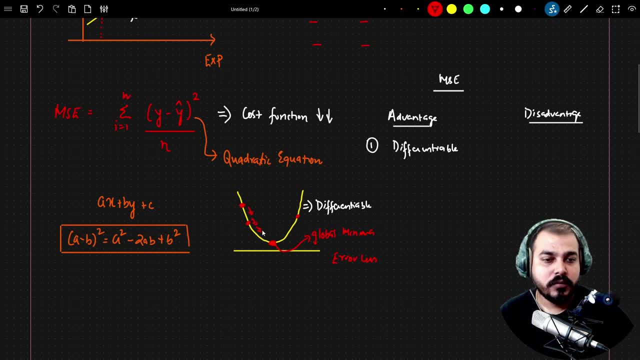 reduce the, we can reduce the coefficient and probably reach the global minima. so most a major advantage is that it is differentiable. coming to the next advantage is that over here, this kind of curve, it has one local and one global minima. this is super important point which everybody needs to focus on, right. 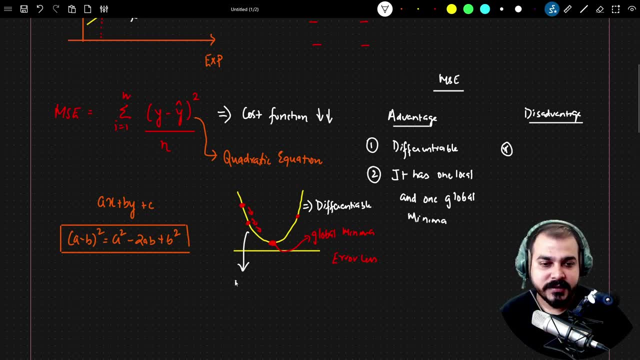 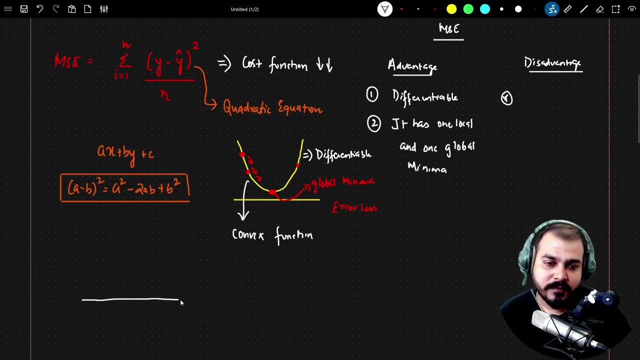 let's say, this particular gradient descent that I see is basically a convex function. okay, if you see some of the curves, let's say that I have one curve like this and this gradient descent curve looks something like this. okay, now, over here you can see that this is not a convex function, obviously here. 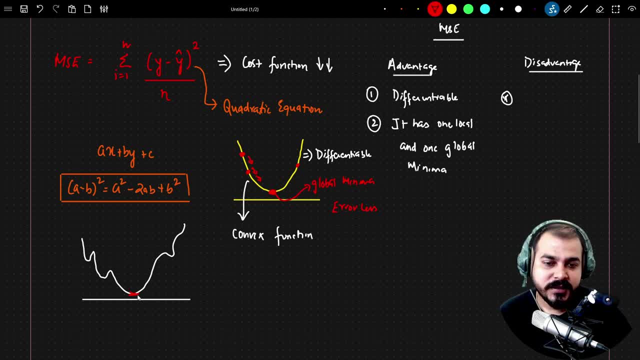 you have one global minima and you'll also be seeing that you'll be having some more minima and this minima is basically called as local minima. if we use different types of equation, in those equation, you'll be seeing that you'll be able to get, or if you plot this equations, you will be, there'll be. 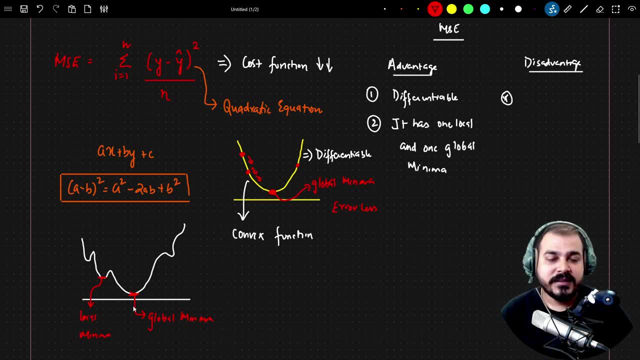 chances that you will be getting both global minima and local minima. but since you're using this quadratic equation- you are plotting it- you will just be having one local or one global minima. right, not multiple, because what will happen? if you have some local minima, then your? 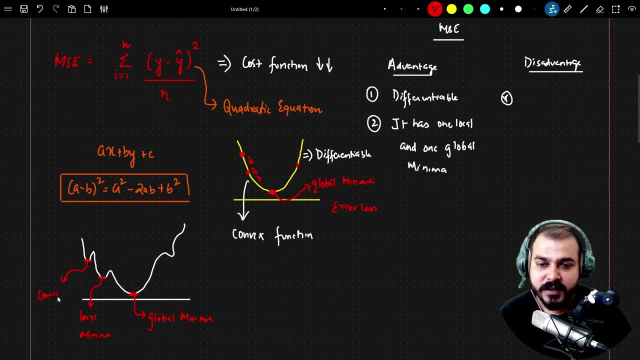 convergence will get stuck over here. right, your convergence will get stuck over here because why here the slope is actually equal to zero is a super important point to understand. what is the differences between local minima and global minima? okay, if you have a local minima, that basically means your convergence. let's say your convergence is: 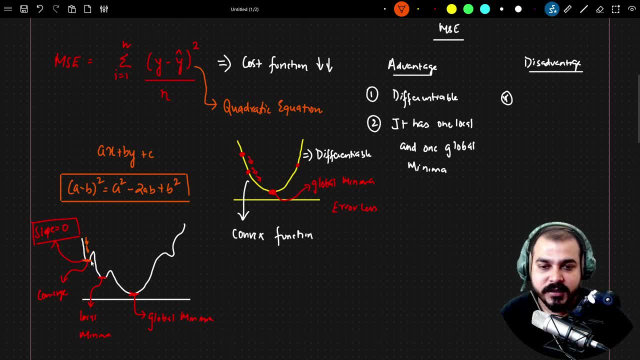 happening like this, it will go ahead and it will stop over here, because here your slope is zero, right, but in the real you really need to reach to the global minima right. so if you use any different kind of equation, specifically not quadratic equation, there are also some equation. 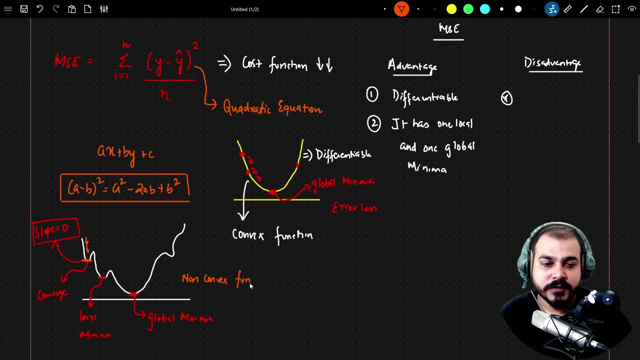 which is basically called as non-convex equations or non-convex functions. in this particular case, you will be seeing that they will be having both local minima and global minima, but currently we are using this quadratic equation, that is, y minus y hat whole square in this particular case, since 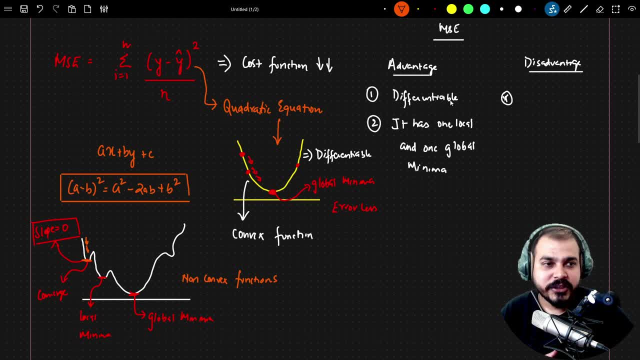 y hat whole square. in this particular case, since it is differentiable, it will just be having one local minima or one global minima. now coming to the third point, which is super important: this equation or this curve. let's say, if i use this particular equation, it converges faster. 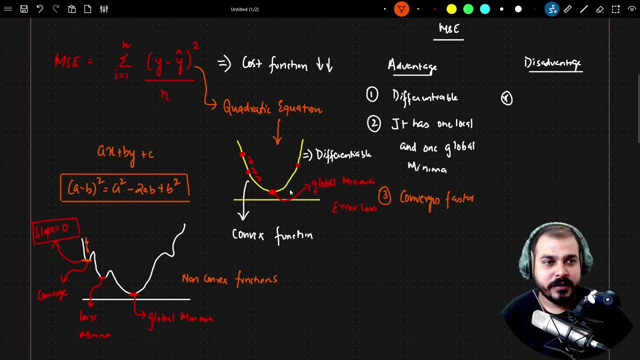 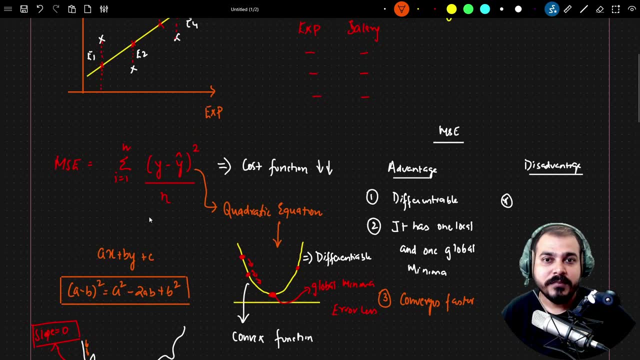 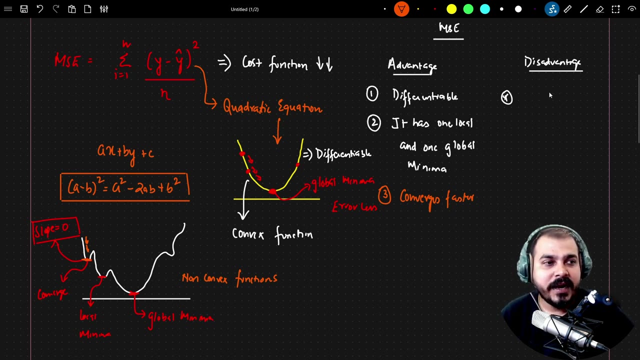 right and we have one already seen how the convergence will basically happen, right? so these are the three main advantages with respect to uh. by using this, uh mean squared error. right now, coming to the disadvantage, which is super important again. okay, now in disadvantage, you will be seeing that the 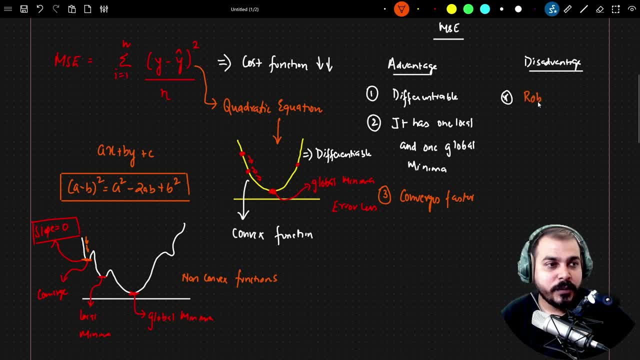 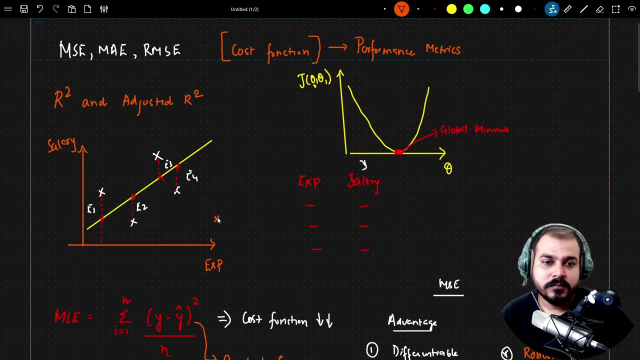 first and the foremost disadvantage of using this is that this equation is not robust. it is not robust to outliers. now why i am saying like this? it is not robust to outliers. let's say: i have a, i have a, i have an outlier like this right now. what will happen if i? 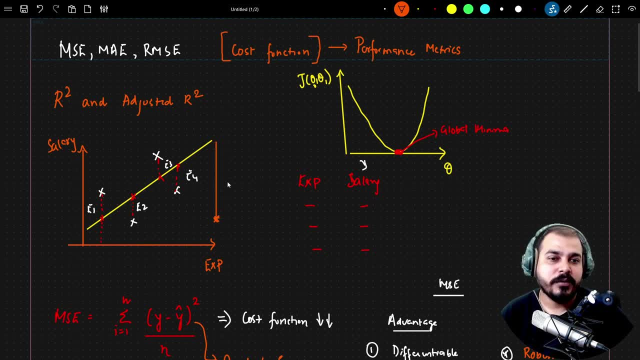 have an outlier obviously here the error that you are trying to compute. later on you will be squaring it right, because y minus y hat whole square right. so here you're penalizing this. this process is basically called as penalizing the outlier. penalizing the outlier now because of this. 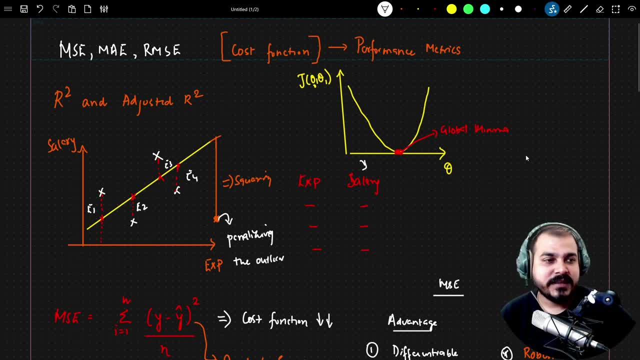 what will happen? error will impact the music increase. Now let's consider that I have some data points which looks like this. Initially, my data points was like this. let's say So. based on this, I created a best fit line. 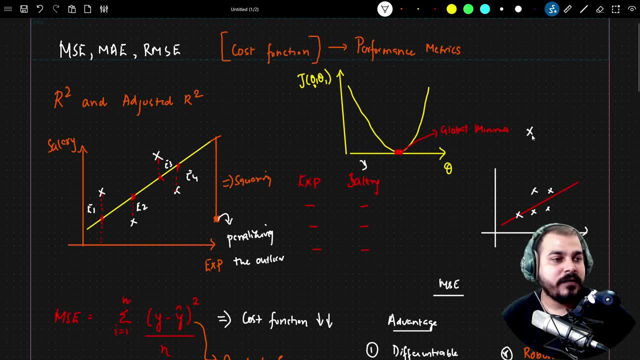 But later on. let's say that I included a new data point which is a kind of outlier, like this. Now, what will happen? your this line right As soon as it sees an outlier. obviously it'll go and compute the error. Now, because of this particular error, obviously this error will. 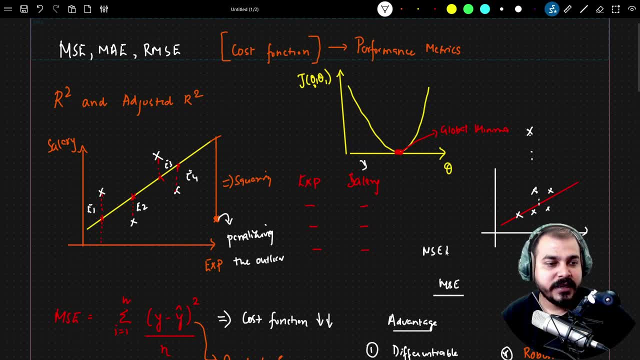 lead to the increase in the MSE right, The MSE will get increased. Now, when MSE is getting increased, we really need to optimize this MSE. Then what will happen is that, because of this error, this line will move towards that particular outlier, like this: But this is absolutely wrong. 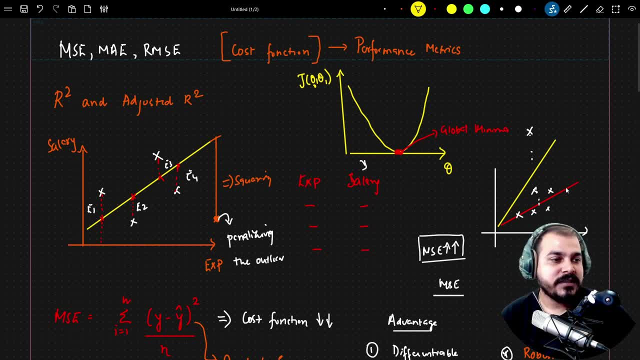 right, Because most of your data points are over here And because of this outlier, you can see that there is a huge shift of the best fit line from here to there, right. So this is what is an impact of an outlier. So this is not robust. 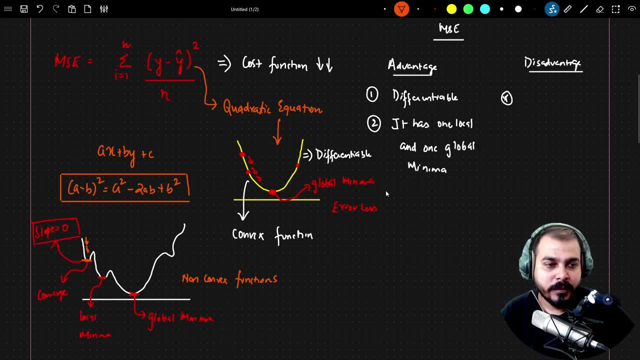 it is differentiable. it will just be having one local minima or one global minima. now coming to the third point, which is super important, this equation, or this curve, let's say, if i use this particular equation, it converges faster right, and we have already seen how the convergence will. 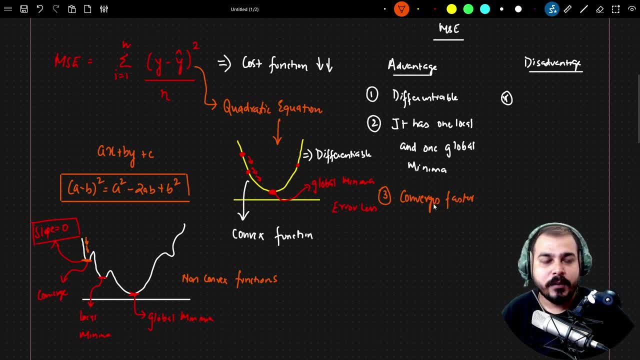 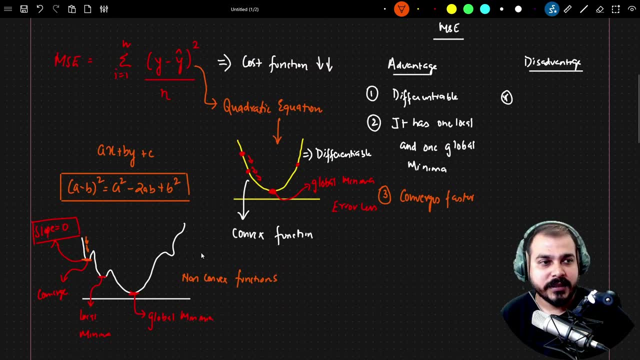 basically happen right. so these are the three main advantages with respect to uh, by using this mean squared error. right now, coming to the disadvantage, which is super important again. okay, now in disadvantage, you will be seeing that the first and the foremost disadvantage of using this is that this equation is not robust. it is not robust to outliers now why i am saying like: 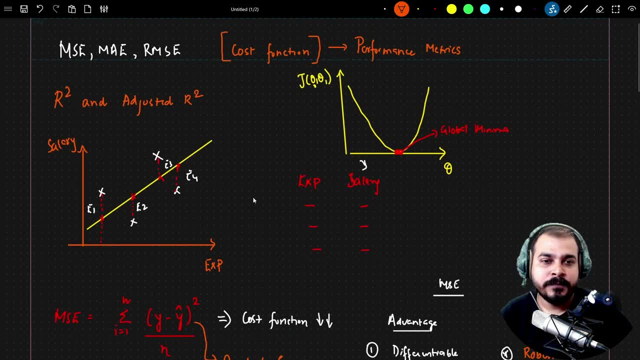 this. it is not robust. to outliers let's say: i have a, i have a, i have an outlier like this right, like this, right now. what will happen if i am an outlier? obviously, here the error that you are trying to compute, later on you will be squaring it. 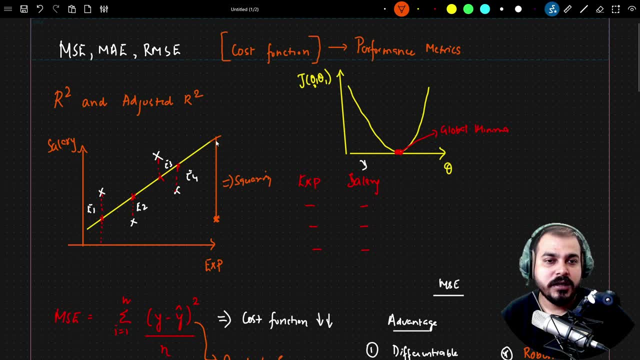 right, because y minus y hat whole square right. so here you are penalizing this. this process is basically called as penalizing the outlier: penalizing the outlier. now, because of this, what will happen? error will increase. now let's consider that i have some data points, which looks like this: 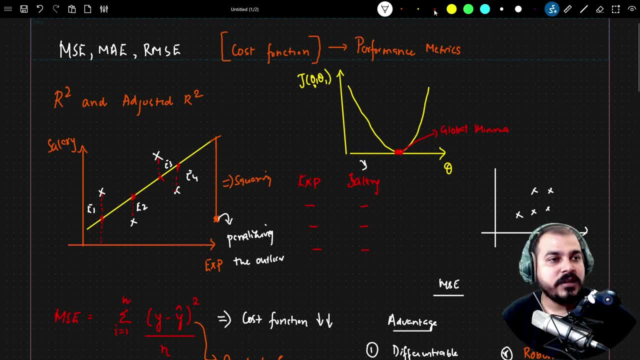 initial points was like this. let's say so. based on this, i created a best fit line. but later on, let's say that i included a new data point which is a kind of outlier, like this: now what will happen? your this line right as soon as it sees an outlier, obviously it will go and compute the error. 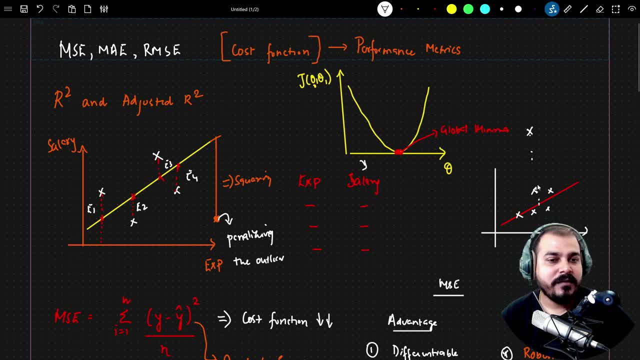 now because of this particular error. obviously this error will lead to the increase in the msc right. the msc will get increased. now, when msc is getting increased, we really need to optimize this msc- then what will happen is that, because of this error, this line will move towards that particular. 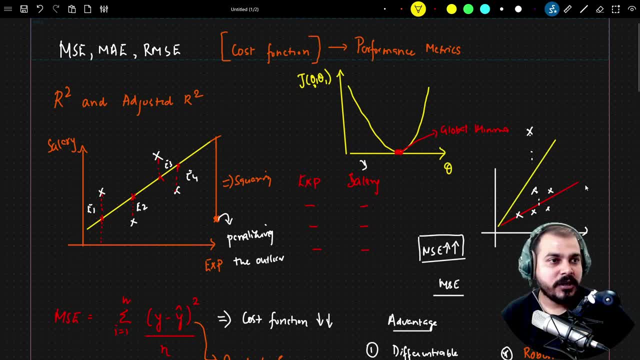 outlier like this, but this is absolutely wrong. right, because most of your data points are over here and, because of this outlier, you can see that there is a huge shift of the best fit line from here to there. right? so this is what is an impact of an outlier. so this is not robust. there is. 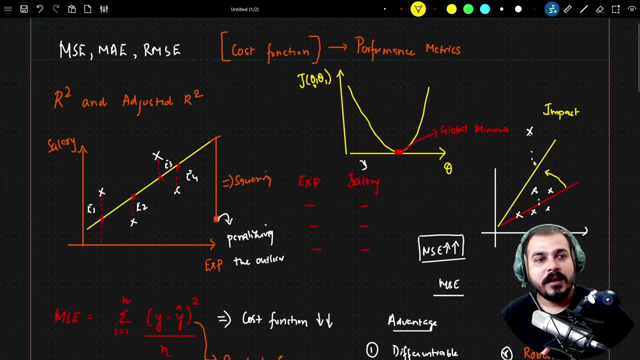 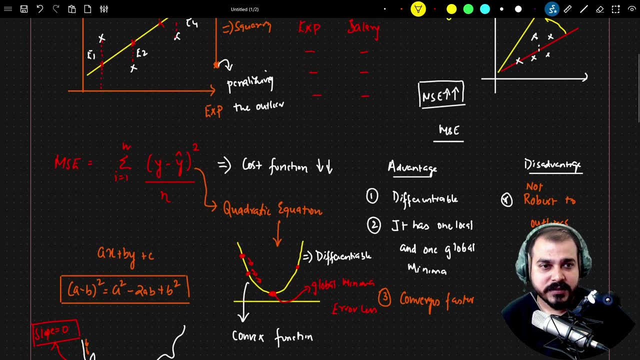 There is definitely because of the outlier. the line is moving from here to there by a huge difference, right, Because obviously we need to reduce the MSE, but currently the MSE is increasing in this particular case, right, So we definitely say that it is not robust to outliers. Okay, So this is the major 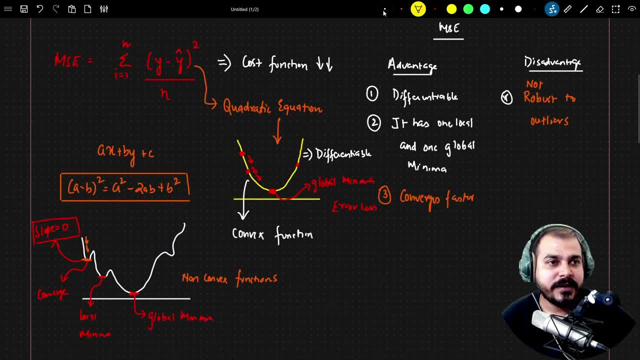 disadvantage with respect to using MSE. Now, coming to the next point, with respect to MSE. Okay, Here, when I try to find out the difference between Y of I and Y hat whole square, you'll be able to see that whatever MSE that I get right, This is basically one by n. 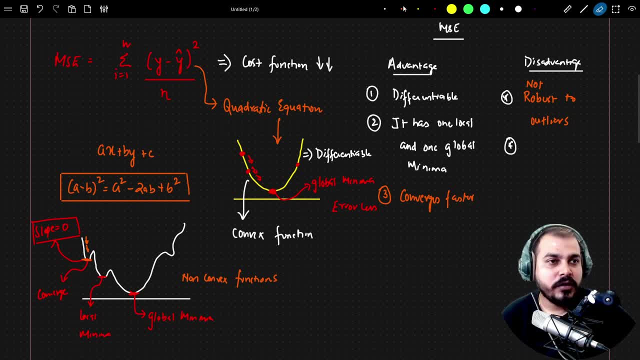 summation. or let me just use this particular equation Again. you know that what is MSE? MSE is nothing but one by n. summation of I is equal to one to n Y of I minus Y of I hat whole square right. So this is the equation over here. right Now, in this specific equation, what is? 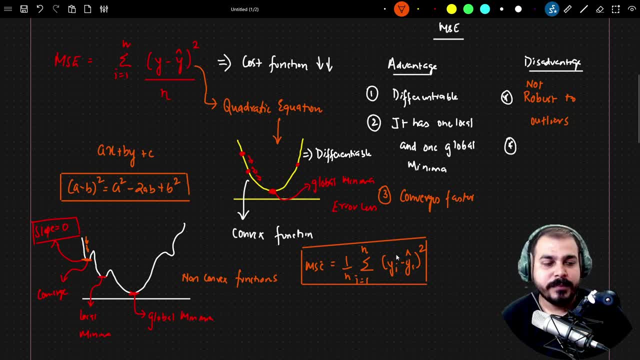 happening is that you're trying to find out the differences between the truth and the predictor value right over here. just focus on this one, okay, here you'll be able to see that y of i minus y of hat whole square. when you're doing whole square, just focus on the units. let's say my y of i. 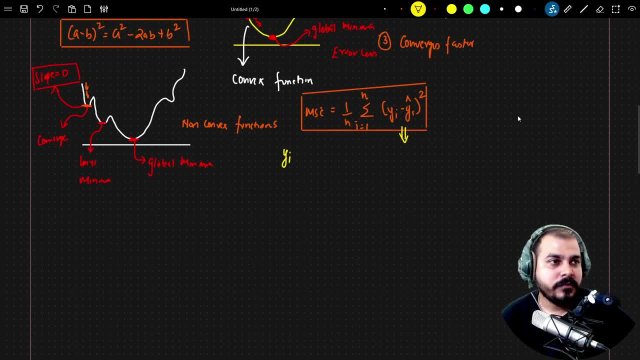 which is, which is the salary variable. okay, let's say, my x axis is basically experience, y axis is salary, and if i do y of i minus y of i hat whole square. the salary will be in some units. let's say, this is in units like lax. now, right now, y of i is basically in lax. but if i do y of i minus y of i, 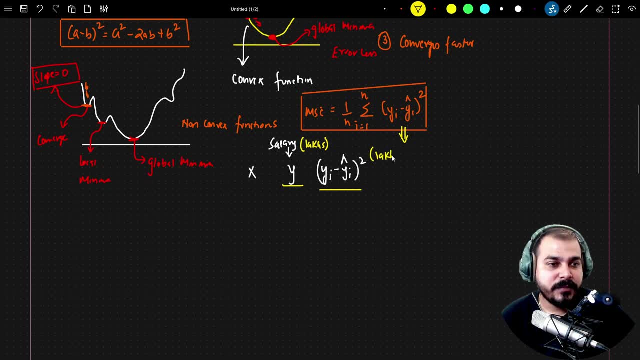 hat whole square that basically i'm changing the units. now this is basically becoming lax whole square. so at the end of the day, you know what is happening with respect to msc is that the y of i and y of i hat whenever we are trying to compute the msc, you know the units is changing when. 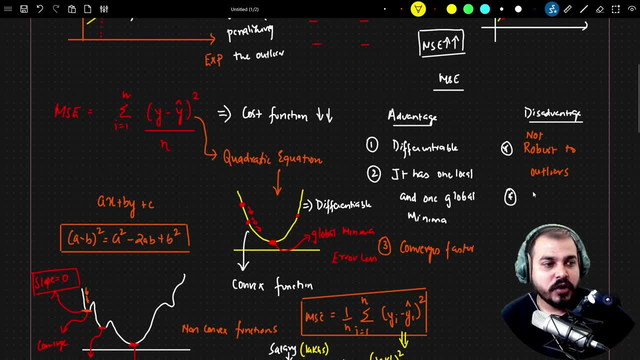 compared to the output variable. so this is also a major disadvantage. so it is no longer in the same unit, longer in same unit. now why i'm putting up this point? because it basically becomes very difficult in terms of understanding that specific information. because, let's say, if my error is, 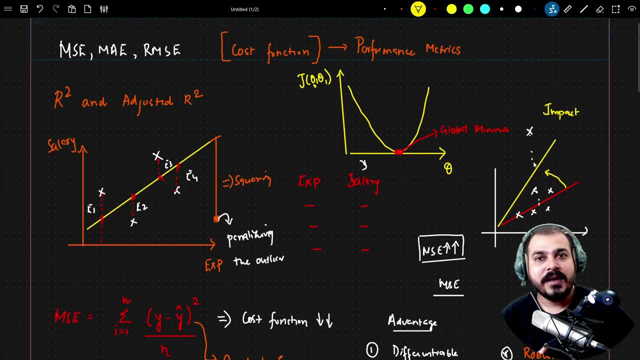 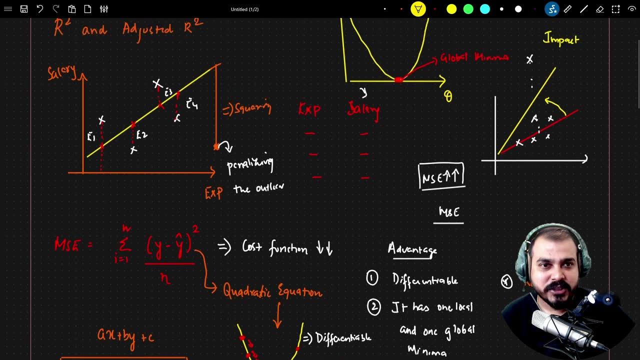 definitely because of the outlier, the line is moving from here to there by a huge difference. right, because obviously we need to reduce the msc, but currently the msc is increasing in this particular case. right, so we definitely say that it is not robust to outliers. okay, so this is the major disadvantage with respect to using msc. 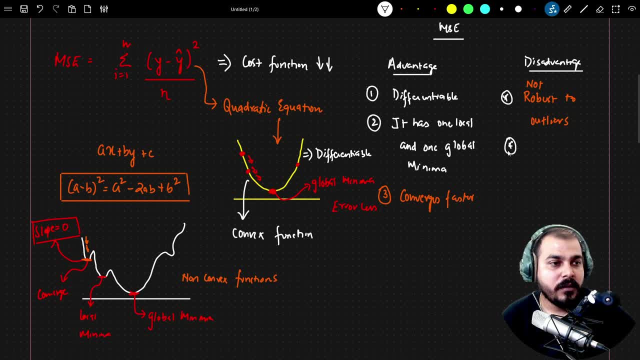 now, coming to the next point, with respect to msc. okay, here, when i try to find out the difference between y, y, y of i and y hat whole square, you'll be able to see that, whatever msc that i get right, this is basically one by n summation, or let me just use this. 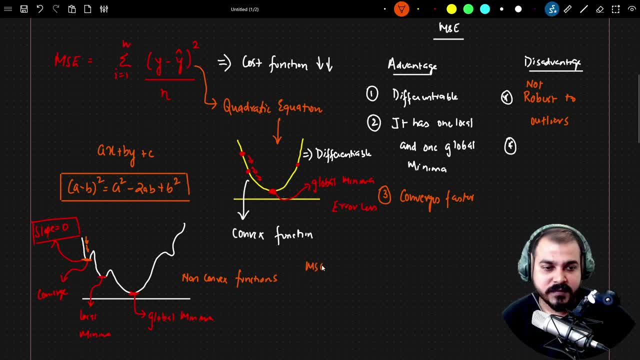 particular equation. again, you know that what is msc? msc is nothing but uh, one by n summation of i is equal to one to n. y of i minus y of i hat whole square right. so this is the equation over here. right now, in this specific equation, what is happening is that you're trying to find out the. 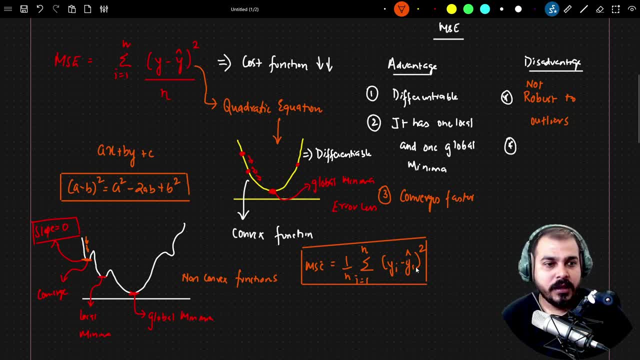 differences between the truth and the predicted value right over here. just focus on this one. okay, here you'll be able to see that y of i minus y hat whole square. when you're doing whole square, just focus on the units. let's say, my y of i. 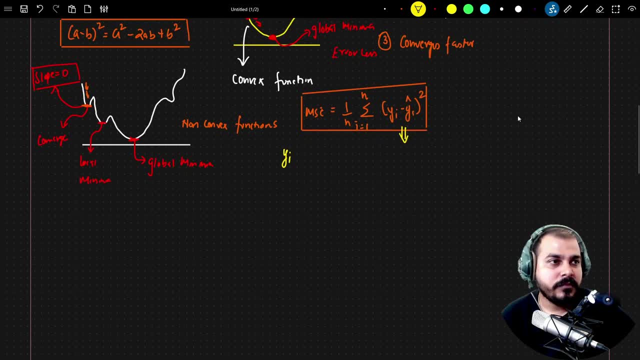 which is? which is the salary variable. okay, let's say, my x axis is basically experience, y axis is salary and if i do y of i minus y of i hat whole square. the salary will be in some units. let's say this is in units like lax now, right now, y of i is basically. 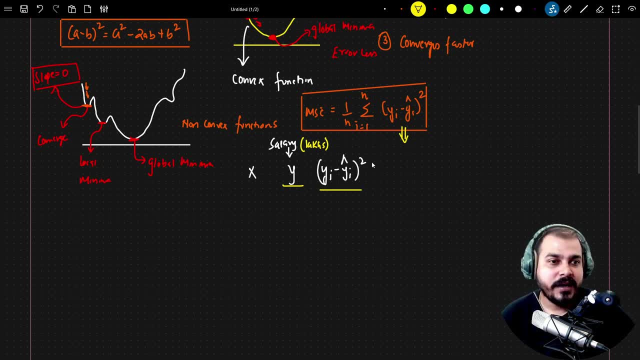 in lax, but if i do y of i minus y of i hat whole square. that basically i'm changing the units. now this is basically becoming lax, whole square. so at the end of the day, you know, what is happening with respect to msc is that the y of i and y of i hat, whenever we are trying to compute the msc. 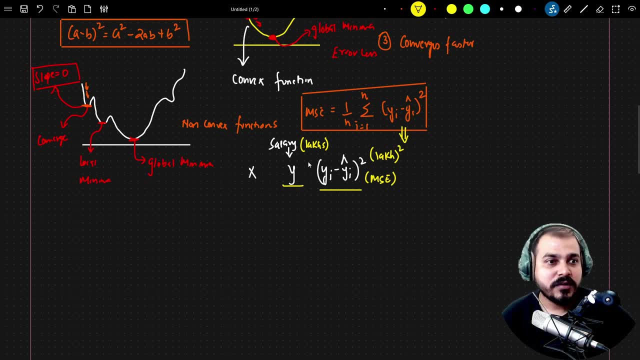 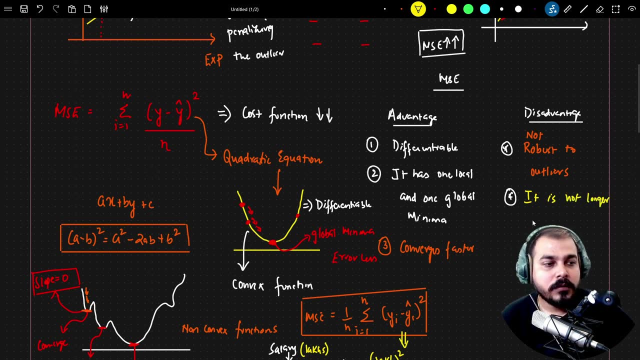 you know, the units is changing when compared to the output variable, so this is also a major disadvantage. so it is no longer in the same unit, longer in same unit. now why you think that this is? i'm putting up this point because it basically becomes very difficult in terms of, uh, understanding. 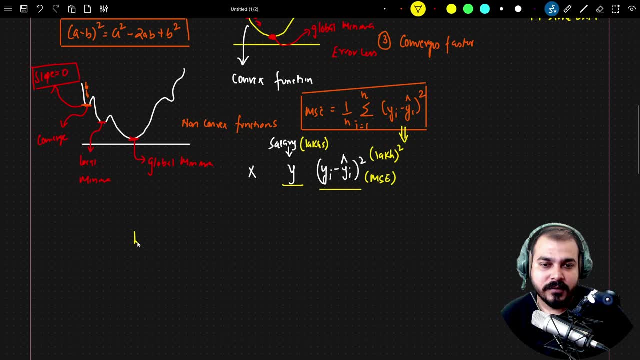 that specific information, because let's say, if my error is coming as, let's say, it is coming as 2.5, lax, right or whatever error that i'm getting with respect to y of i minus y of i, hat whole square is, let's let's say that it is 2.5. now here you know that this particular units, that it is. 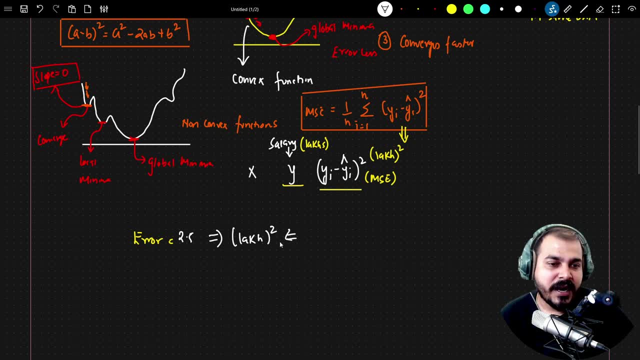 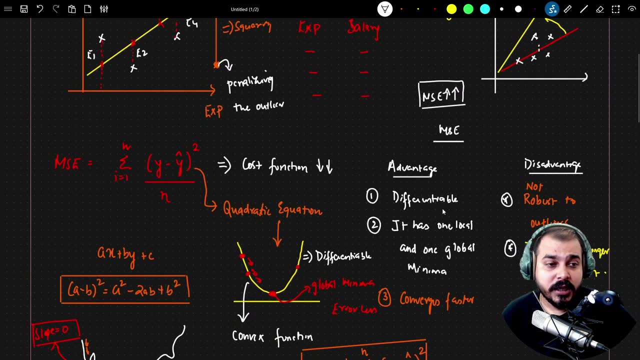 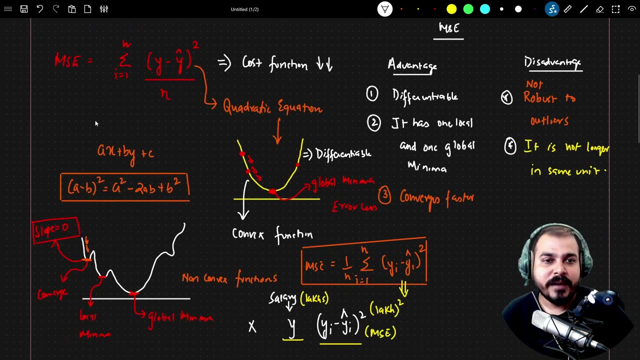 specified, it is with lax square, so it becomes difficult in understanding when you're comparing it with the truth value. okay, so this is the major, major advantage, major major disadvantage. so again, let me revise with respect to advantage and disadvantage. first, the advantage is that obviously, whenever you use msc, it is going to create this. 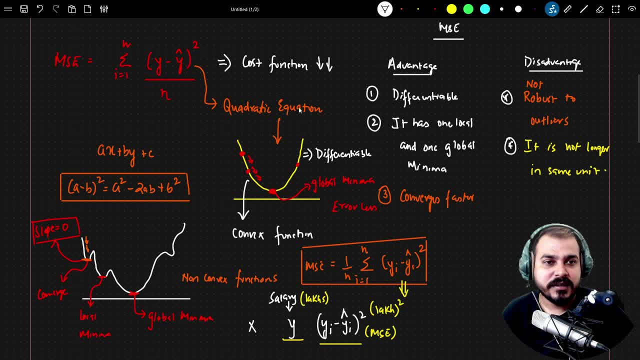 kind of curve, because y minus y hat whole square is nothing, but it is a quadratic equation and whenever you have a quadratic equation, at the end of the day you are going to get this kind of curve. so the major advantage with respect to this curve, which is called as a gradient descent curve, it is first of all differentiable. that which i have 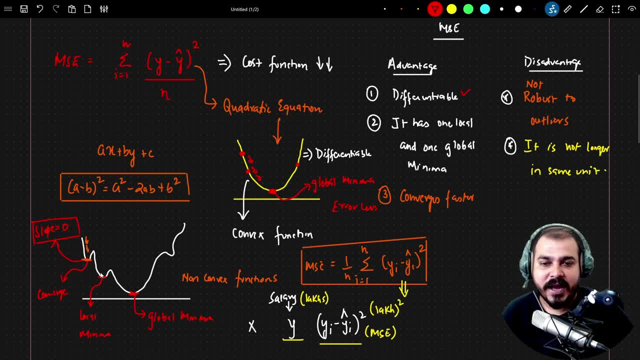 specified. it has one local and one global minima. it does not have multiple local or or more than one global minima, like like this kind of situation. so obviously we know that where we really need to reach, that is over here, and when we reach near this, the error will be less. the third thing is: 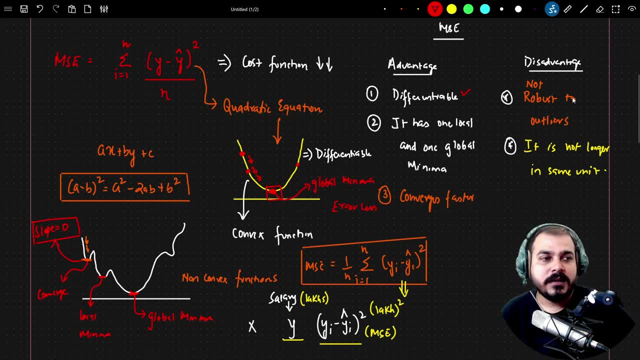 that it converges faster because we don't have any local minima over here. the disadvantage is that it is not robust to outliers, and it is not. it is not longer in the same minute, it it? that basically means it is not in the same unit. okay, i'm just 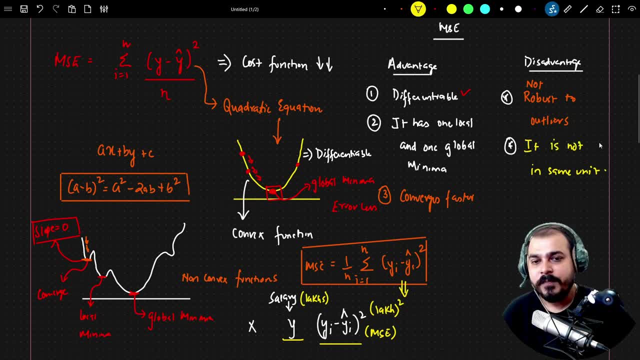 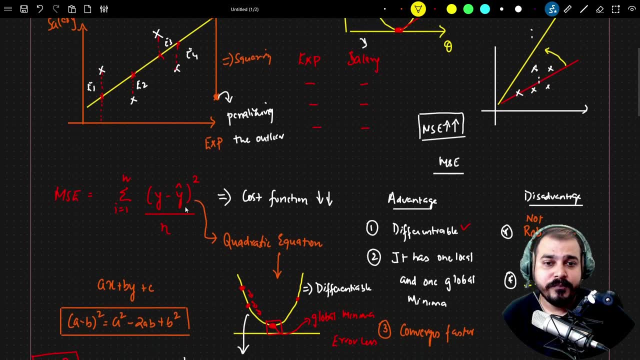 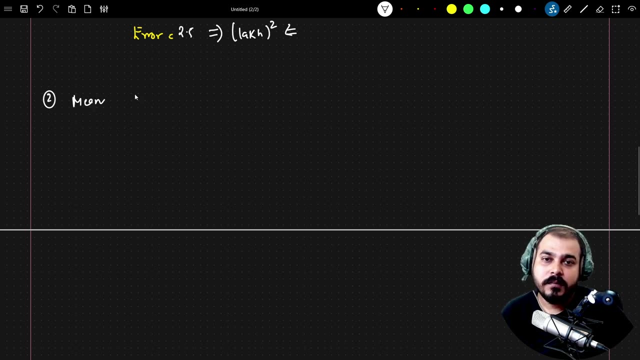 going to mention this again. it is not in the same unit. okay, so this is about msc. now let's go ahead and discuss about mean squared error. uh, sorry, mean absolute error. so here, uh, i've discussed about msc. the second one that i'm going to discuss is about mean absolute error. 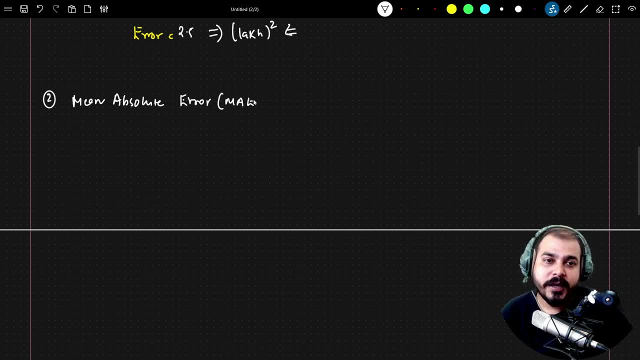 now mean absolute error. what happens when you have a mean absolute error? what happens if we take this cost function or loss function when we are creating our gradient descent right? so mean absolute error is basically given by the formula one: by n, summation of i is equal to. 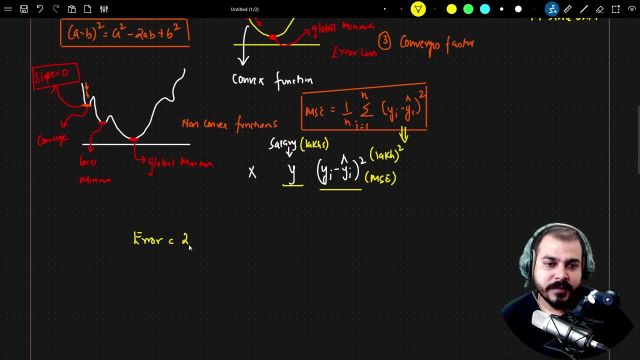 coming as, let's say it is coming as two point five, lax right, or whatever error that i'm getting with respect to y of i minus y of i hat whole square is. let's let's say that it is two point five. now here you know that this particular 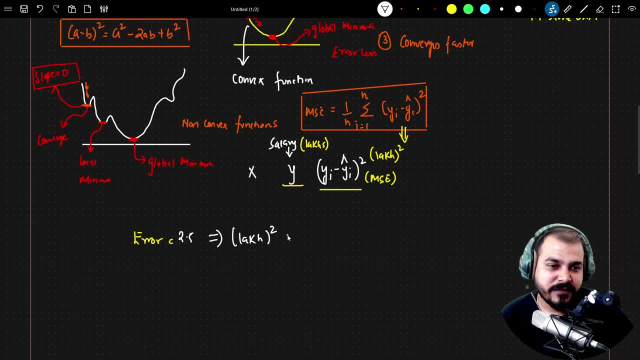 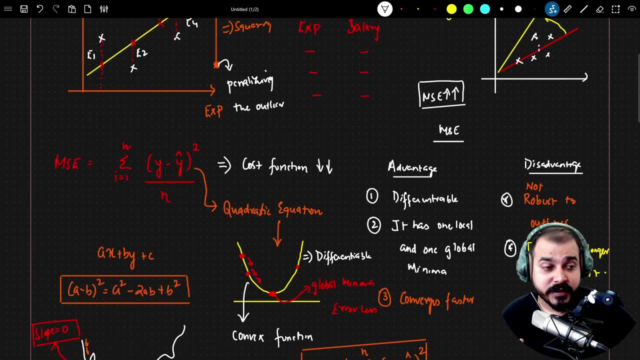 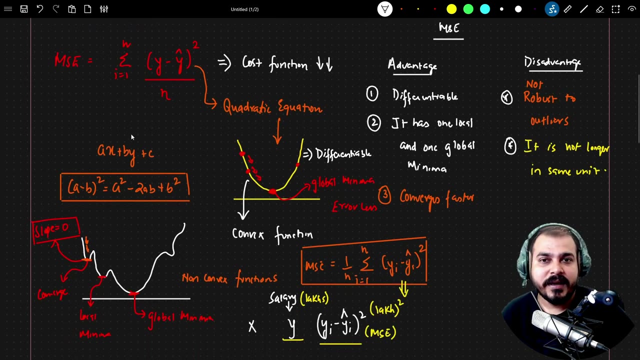 units that it is specified. it is with lax square, so it becomes difficult in understanding when you are comparing it with the truth value. okay, so this is the major major advantage, major major disadvantage. so again, let me revise with respect to advantage and disadvantage. first, the advantage is that obviously, whenever you are comparing it with the truth value, you are comparing it with 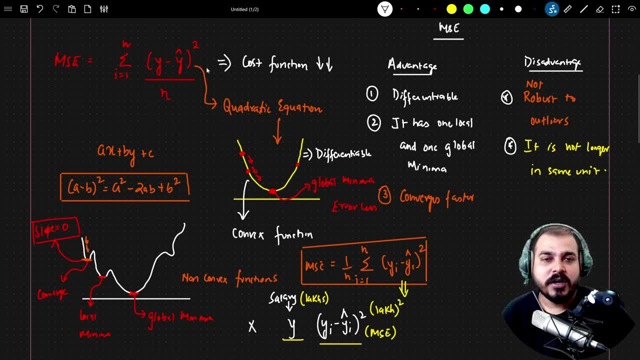 the truth value. so whenever you use msc it is going to create this kind of curve, because y minus y, hat whole square is nothing, but it is a quadratic equation and whenever you have a quadratic equation, at the end of the day you are going to get this kind of curve. so the major advantage with 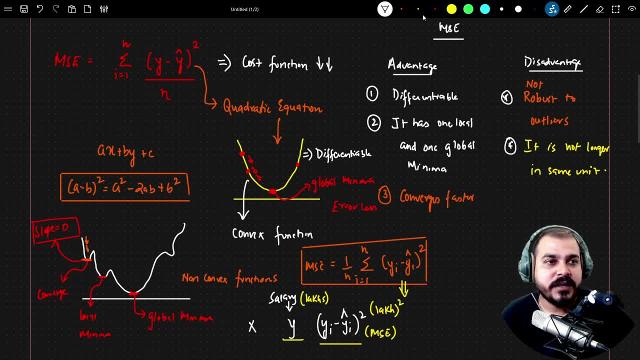 respect to this curve, which is called as a gradient descent curve, it is, first of all, differentiable, that which i have specified. it has one local and one global minima. it does not have multiple local or or more than one global minima, like like this kind of situation. 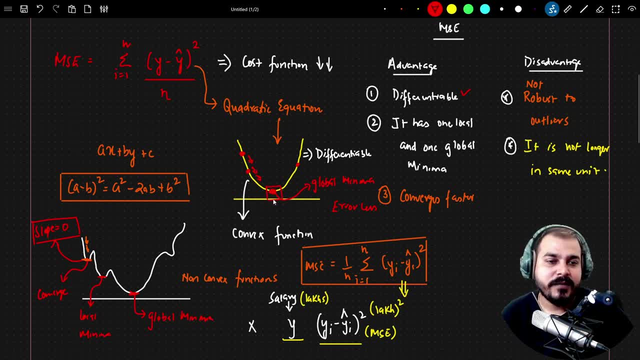 so obviously we know that where we really need to reach that is over here, and when we reach near this, the error will be less. the third thing is that it converges faster because we don't have any local minima over here. the disadvantage is that it is not robust to outliers and it is not 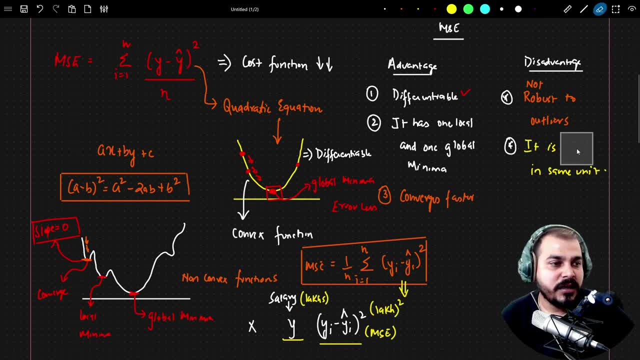 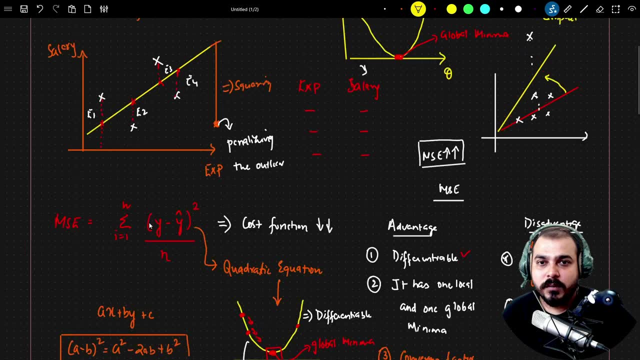 it is not longer in the same minute, it that basically means it is not in the same unit, okay? i'm just going to mention this again. it is not in the same unit, okay? so this is about msc. now let's go ahead and discuss about mean squared error. uh, let's go ahead and discuss about mean squared error. 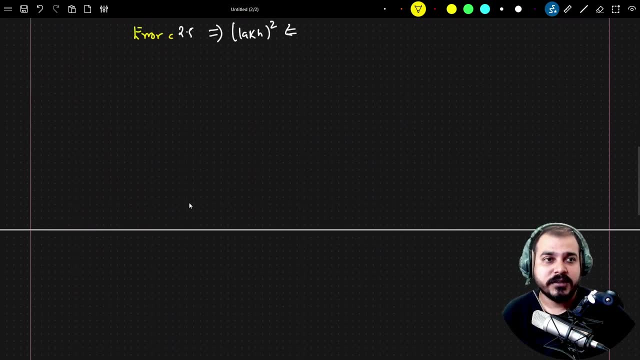 sorry, mean absolute error. so here, uh, i've discussed about msc. the second one that i'm going to discuss is about mean absolute error. now, mean absolute error. what happens if we take this cost function or loss function when we are creating our gradient descent right? so mean. 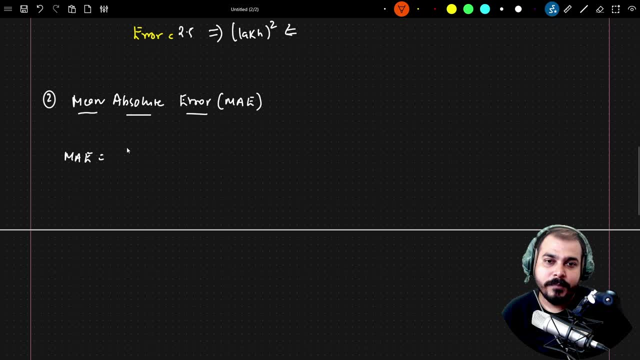 absolute error is basically given by the formula 1 by n. summation of i is equal to 1 to n, and this is y minus y hat whole, not whole square. it will be the absolute value of y minus y hat. now here let's talk about the advantages and disadvantages. first of all, let's go ahead towards. 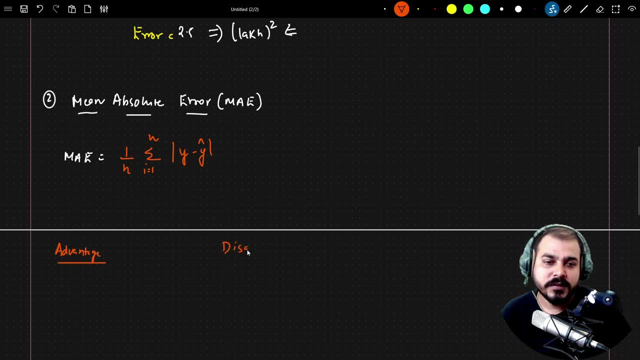 the advantage and let's go towards the disadvantage now. i think just by seeing the equation, you'll be able to understand the advantage. first of all, this will definitely be robust to outliers. now, why it is robust to outliers? because, let's consider- these are my data points. 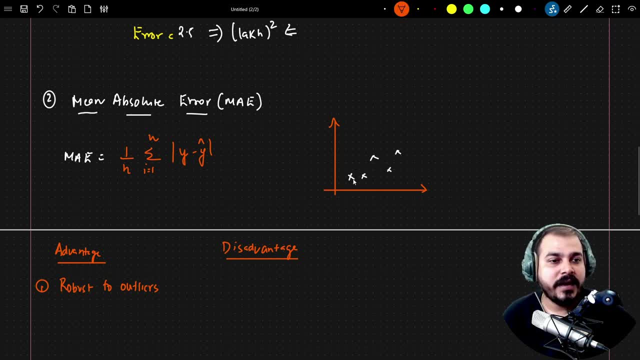 and let's say i have some of the data points like this and let's say i have created a best fit line. let's say again, while training my data points, you know, i get an outlier which is over here now. what will happen is that, since my formula is not squaring, or not, 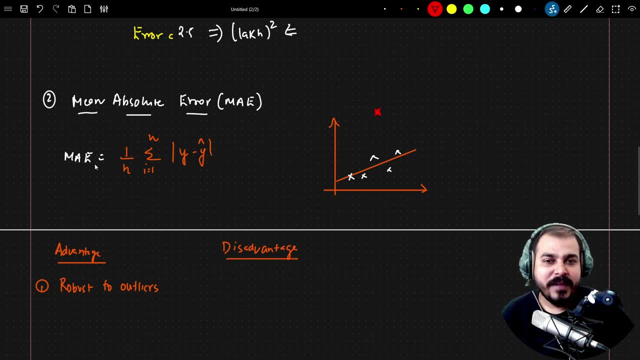 penalizing this specific error. you know that mae will get increased, but it will not get increased like how mse used to get increased. right error, we are trying to square it over there. but here the error, what it is coming: it will just increase mae by some amount. okay, so because of this, what will happen? my line will not, my best fit line will not. 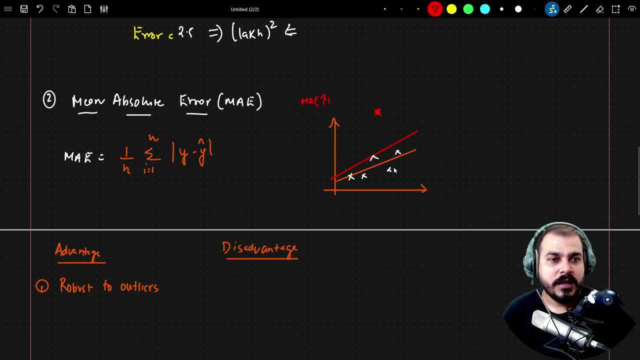 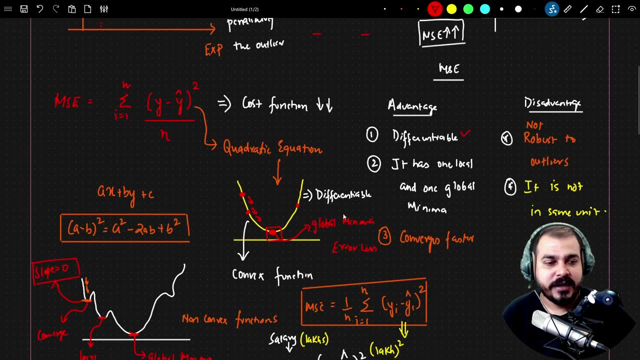 divert that much, but it will just divert in a simpler way like this: okay, so this movement is just this much, whereas in the case of uh msc you could see there is a huge movement in the best fit line. okay, and obviously we need to uh reduce this mac also. that is also the 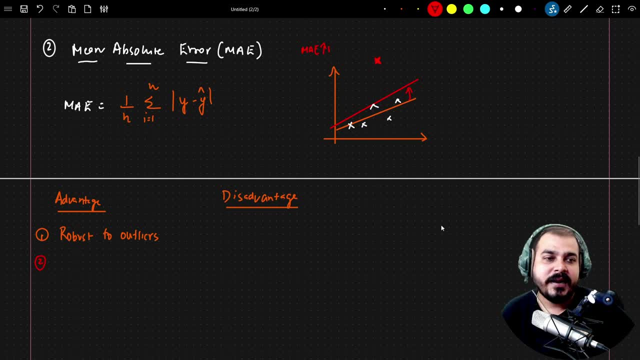 major thing, okay. the second advantage is that when i'm trying to calculate y minus y hat, it will be in the same unit. right, it will be in the same unit, so same unit. so understanding the data over here will be simple, because your y hat and y minus y 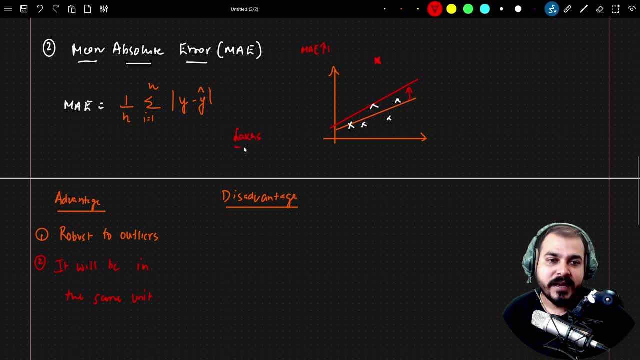 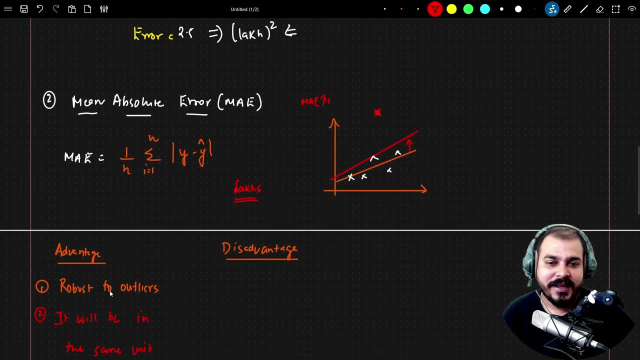 hat will be in the same units. that is like lax if i compare with respect to salary. it is not becoming lax square right. so this is the second advantage and obviously because of this, only this thing is getting there right. but coming to the disadvantage, which is super important point, 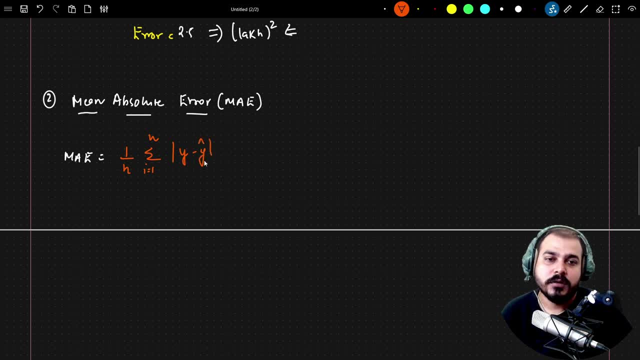 one to n, and this is y minus y hat. whole, uh, not whole square. it will be the absolute value of y minus y hat. now here let's talk about the advantages and disadvantage. first of all, let's go ahead towards the advantage and let's go towards the disadvantage. 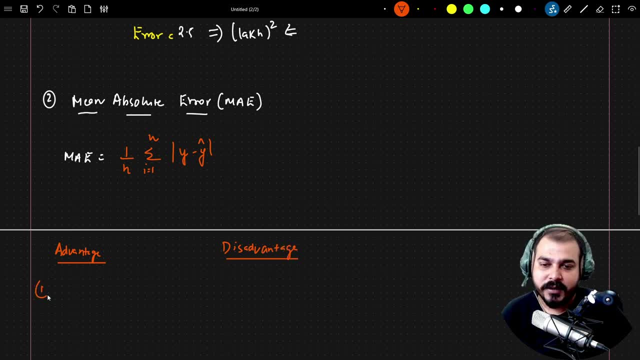 now. i think just by seeing the equation you'll be able to understand that advantage. first of all, this will definitely be robust to outliers. now, why it is robust to outliers? because let's consider: these are my data points. and let's say i have some of the data points like this, and let's say: 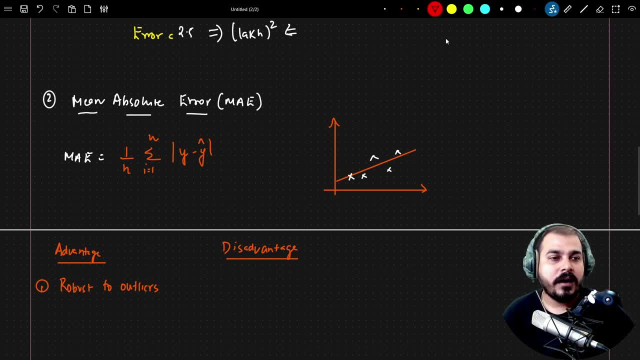 i have created a best fit line. let's say i've again, while training my data points, you know i get an outlier which is over here now. what will happen is that, since my formula is not squaring or not penalizing this specific error, you know that mae will get increased, but it will not get. 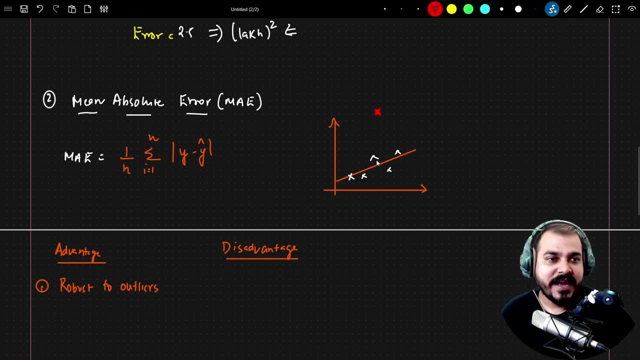 increased, like how mse used to get increased. right error. we are trying to square it over there, but here the error, what it is coming, it will just increase mae by some amount. okay, so because of this, what will happen? my line will not, my best fit line will not divert that much, but it will. 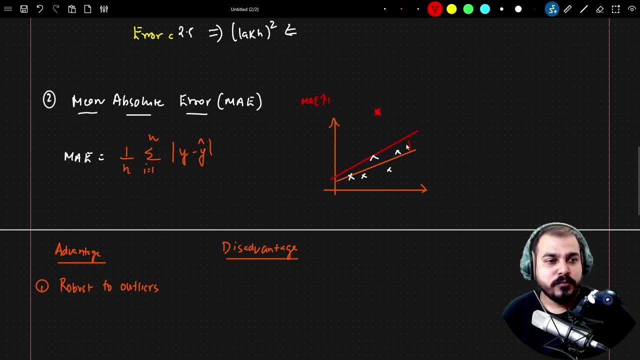 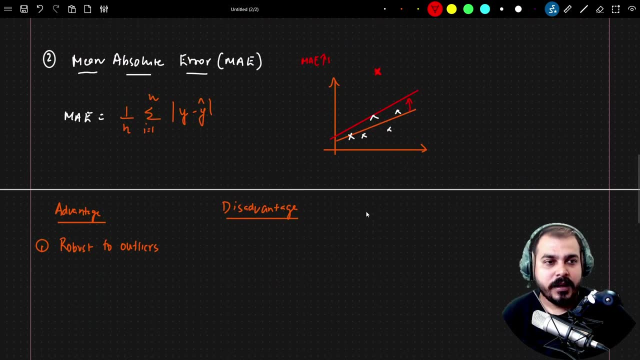 just divert in a simpler way like this: okay, so this movement is just this much, whereas in the case of uh msc, you could see there is a huge movement in the best fit line. okay, and obviously we need to uh reduce this mac also. that is also the major thing, okay. the second: 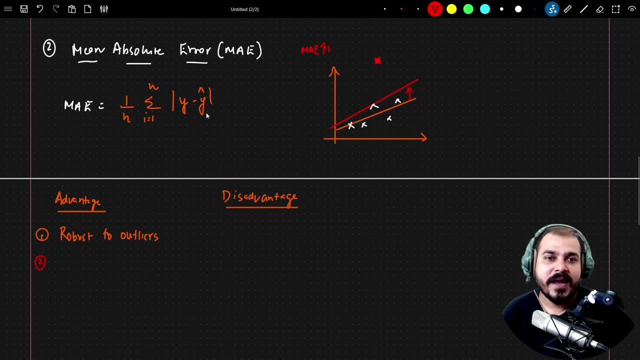 advantage is that when i'm trying to calculate y minus y hat, it will be in the same unit. right, it will be in the same unit, so same unit. so understanding the data over here will be simple, because your y hat and y minus y hat will be in the same units. that is like lax. 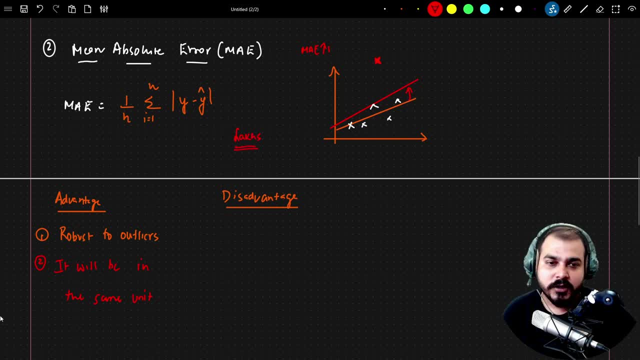 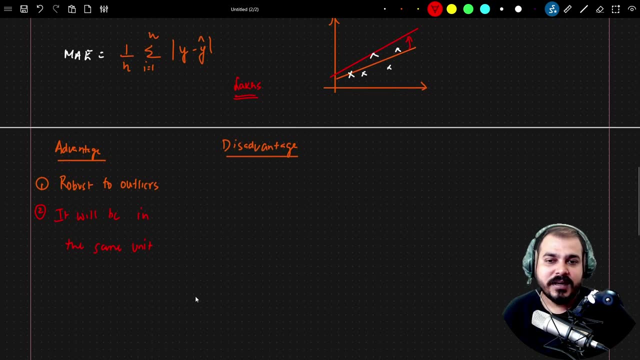 if i compare with respect to salary, it is not becoming lax square right. so this is the second advantage and obviously because of this, only this thing is getting there right. but coming to the disadvantage, which is super important point, okay, obviously, uh means mean absolute error is used to. 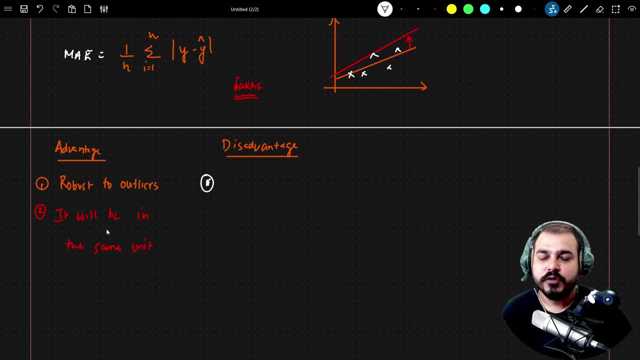 okay, obviously, uh means mean absolute error is used to, um you know, basically because of the outlier that is present in mean squared error, because of the impact of the outlier that is present in the mean squared error, we are trying to solve it with the help of mean absolute error. 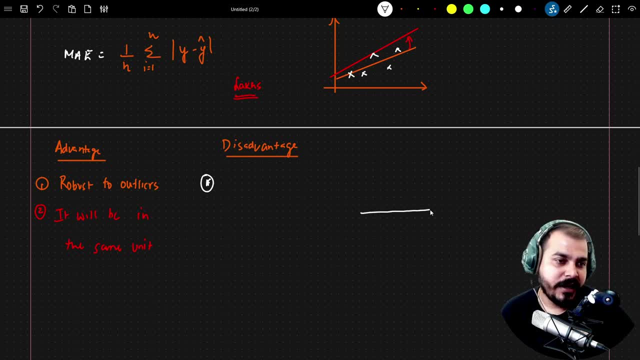 but here, if i talk about differentiability, right in the case of mean absolute error, if i use this equation, usually what happens? i will get this kind of curve. now this curve. you'll be thinking it looks like gradient descent. no understand, guys. here you are passing through zero. 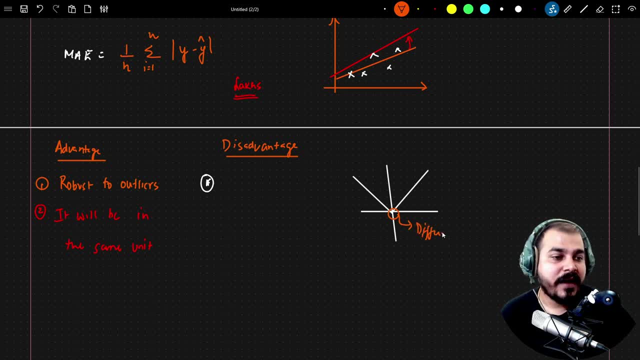 here. at this point, we cannot differentiate any value at zero. we cannot differentiate any value at zero, right? so what we do is that we create something called a subgradients. okay, subgradients. now. subgradient basically means what i will be taking a part of this part of this and then probably finding out the uh slope and then trying to compare. 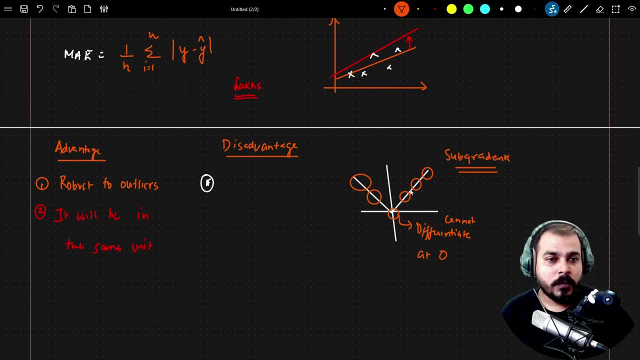 and trying to come to a global minimum point. okay, so this is a major disadvantage. with respect to this, the major disadvantage is that convergence usually take more time, usually takes more time. take more time because why, why? why? the convergence will take more time because understand the optimization. the optimization is a complex task. now what is the optimization over here? 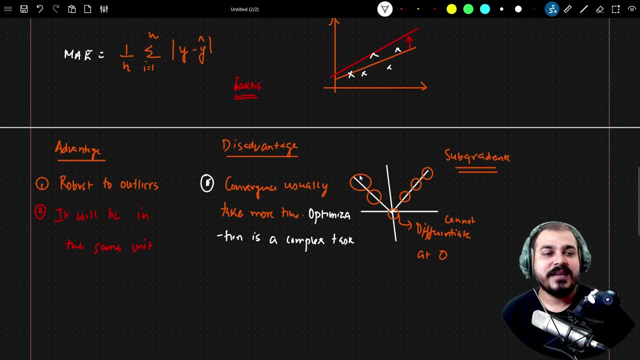 that we really need to come to a global minima. but right now, here you basically have this kind of gradient descent and you know that at this point of time, if you probably go at this re, at this particular point, that basically means it is not at all differentiable at zero, and that is what 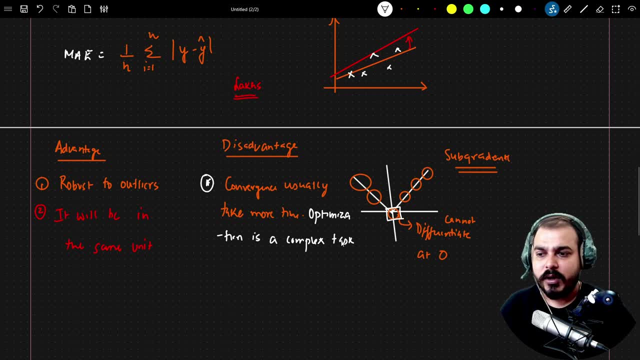 derivative. derivative will not happen at the point of zero, right, you cannot differentiate anything that is at zero. okay, so what you do is that you try to divide that into sub gradient and then you try to calculate the slope. okay, then only you will be able to calculate the slope. now, optimization is: 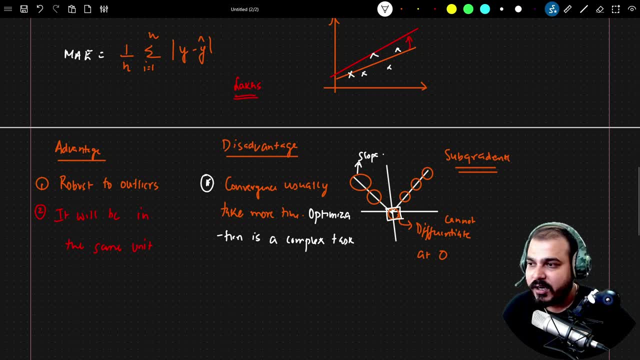 a complex task. so you have to calculate the slope and then you have to calculate the gradient descent over here. definitely, uh, optimization is not that specific, easy, but one very important thing that you will be able to see that, uh, you know, uh, in this it is definitely robust to outliers, right. 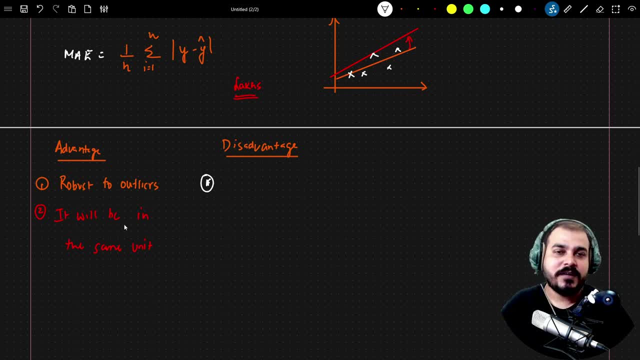 um, you know, basically, because of the outlier that is present in mean squared error, because of the impact of the outlier that is present in the mean squared error, we are trying to solve it with the help of mean absolute error. but here, if i talk about differentiability, right, in the case of mean absolute error, if i use this, 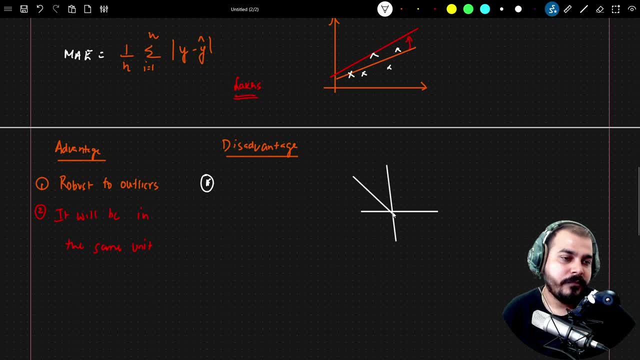 equation. usually what happens? i will get this kind of curve. now this curve, you'll be thinking it looks like gradient descent. no understand, guys. here you are passing through zero here. at this point we cannot differentiate any value at zero. we cannot differentiate any value at zero, right? 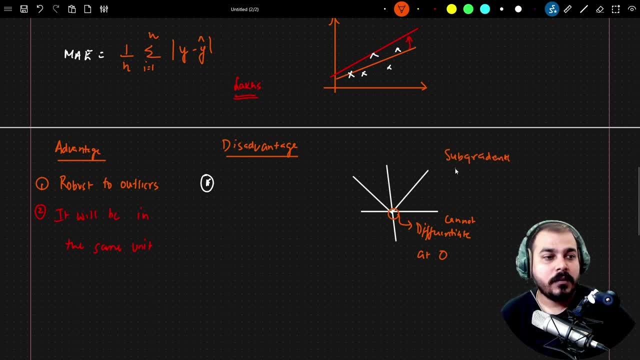 we create something called a sub gradients. okay, sub gradients now, sub gradient basically means what: I will be taking a part of this part of this and then probably fighting out the slope and then trying to compute and trying to come to a global minimum point. okay, so this is a major disadvantage with 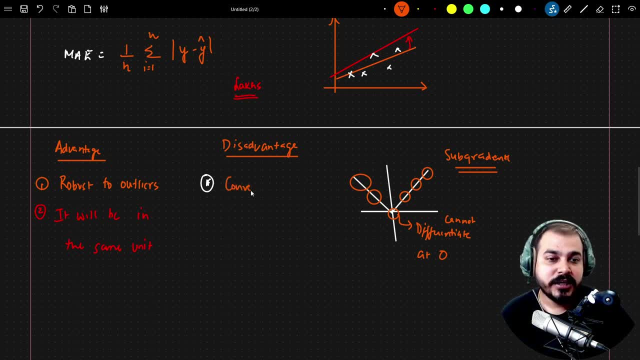 respect to this, the major disadvantage is that convergence usually take more time. usually takes more time. take more time because why the convergence will take more time? because understand the optimization. the optimization is a complex task. now, what is the optimization over here that we really need to come to a global minima? but right now here you basically have this. 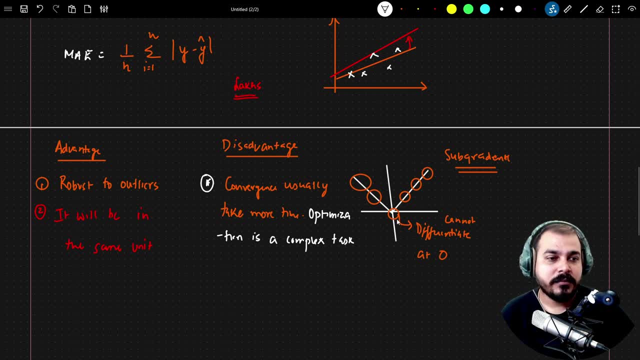 kind of gradient descent and you know that at this point of time, if you probably go at this, we at this particular point of time you will have this kind of gradient descent. and you know that at this point of time, if you point, that basically means it is not at all differentiable, at zero, and that is. 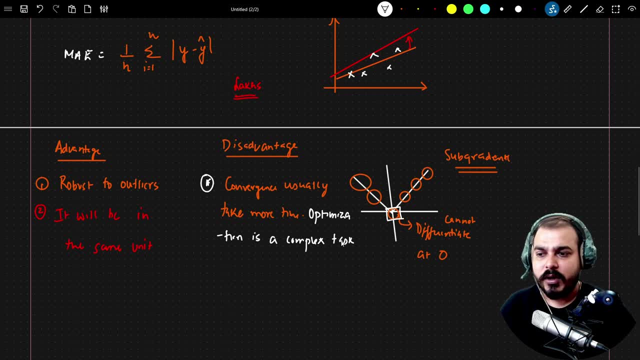 what derivative? derivative will not happen at the point of zero. right, you cannot differentiate anything that is at zero. okay, so what you do is that you try to divide that into sub gradient and then you try to calculate the slope. okay, then only you will be able to calculate the slope. now, optimization is a complex 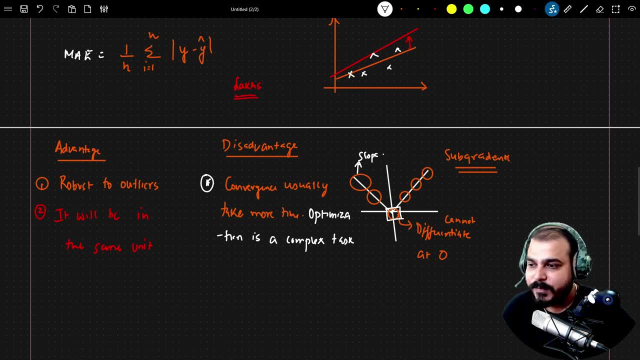 task over here. definitely, optimization is not that specific, easy, but one very important thing that you will be able to see, that you know, in this it is definitely robust to outliers right. this is the major task now. here it will definitely be time consuming, okay, so these are some. 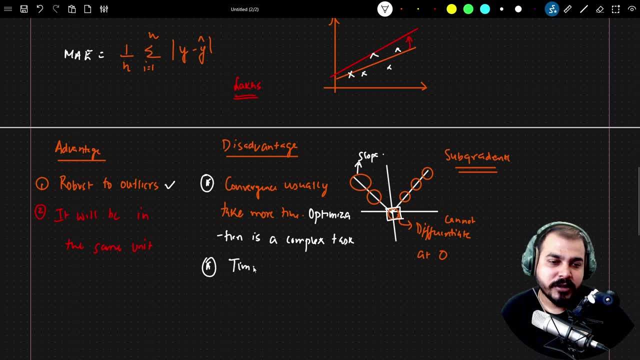 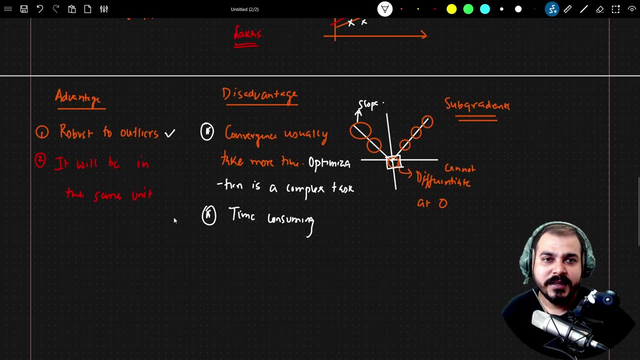 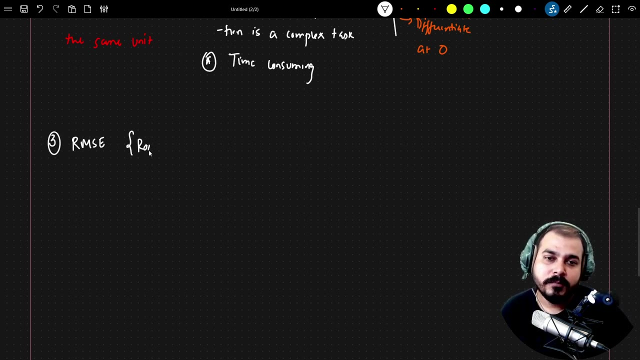 this is the major task now. here it will definitely be time consuming, okay, so these are some of the advantages and disadvantages. with respect to ma mae, that is mean, absolute error. now let's go ahead with respect to third one, which is called as, so here i'm just going to write it as root: mean squared error. now, here we can definitely write. 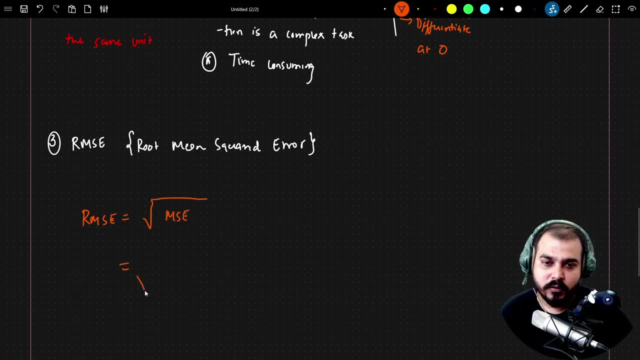 our mac as root of mac. so if i say root of msc, what it is, it is nothing but root of 1 by n. summation of i is equal to 1 to n. y of i minus y of i hat whole square. okay, so this is the entire. 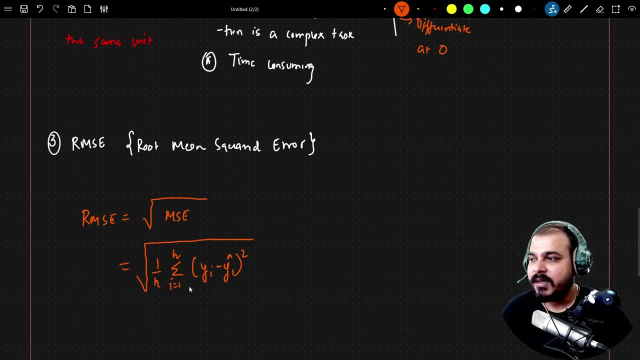 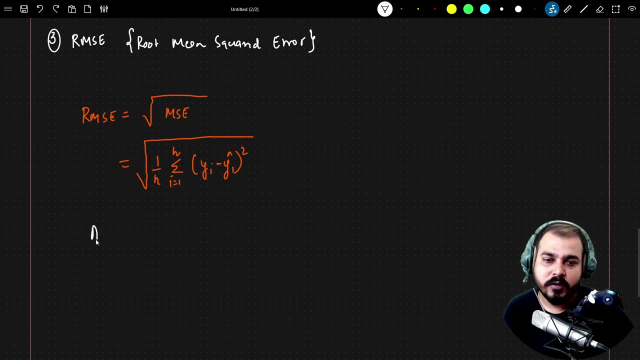 formula with respect to our msc again, uh, in this, uh, what will be the benefit? one benefit that i can definitely compare, uh, since i am doing the square root, right. so initially in msc it was not in the same unit, right? so first advantage that i would like to call about is that. 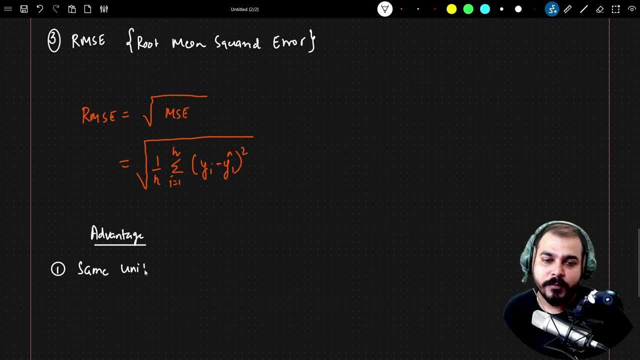 first advantage: here the values that you are getting is in the same unit. second thing: this is obviously differentiable. okay, since here also you will be anyhow getting a gradient descent. but the major disadvantage- if i die down here it is the gradient descent to talk about- is that, since we are again doing squaring here, it is not robust to outliers. 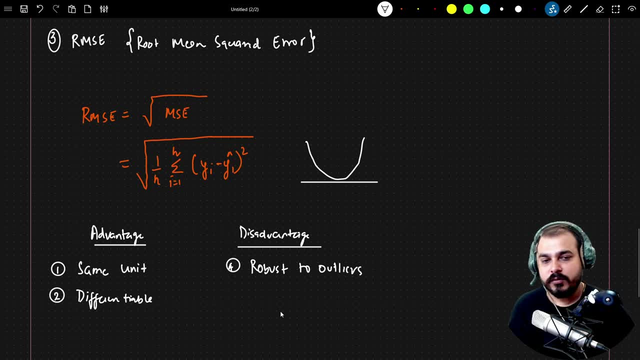 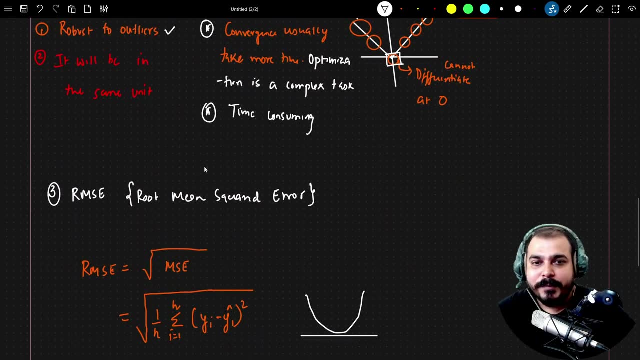 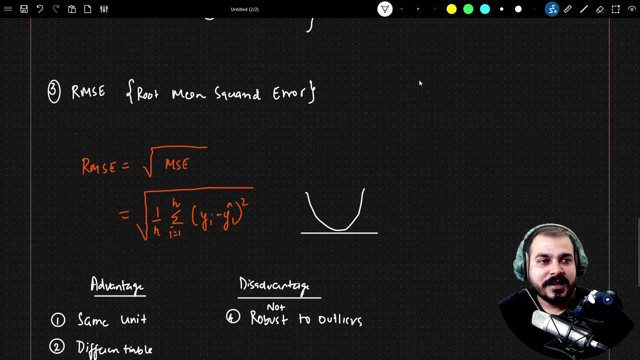 okay, not robust to outliers. now we have learned about this. all three techniques. at the end of the day- you may be considering krish- which one should we use. should we use ma he, mac or rmse? my answer will be that, guys, as a starter we should try to look on all three of them right: rmse, all three of 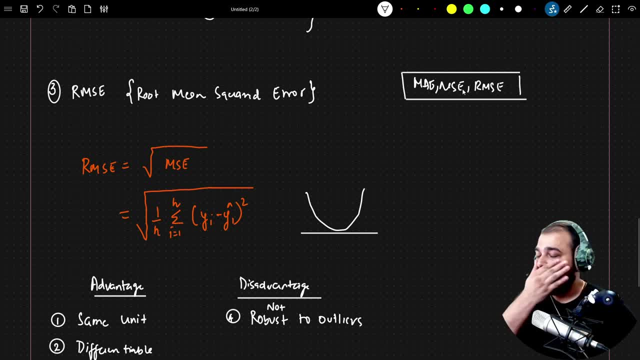 them. so whenever you'll also be seeing that in further, whenever i try to create any linear regression model, i will also be showing you the errors that is going to come, because, see, once, we probably create a best fit line. obviously, let's say if there are some data points, first of all, i 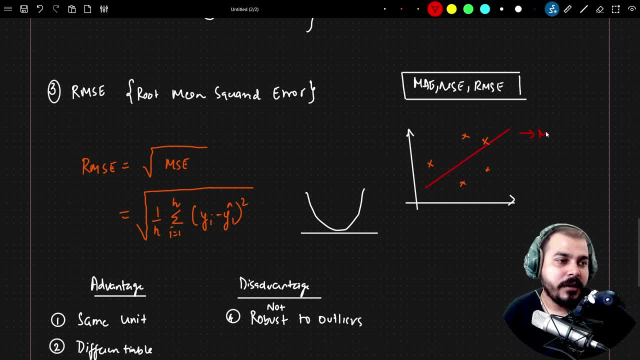 will try to create a best fit line. then what i'll do? i will try to calculate the best fit line, the mac, the mean squared error, the mean absolute error and rmse, and after this i will also try to check the performance of this model with the help of r square and adjusted r square. so as a starter, 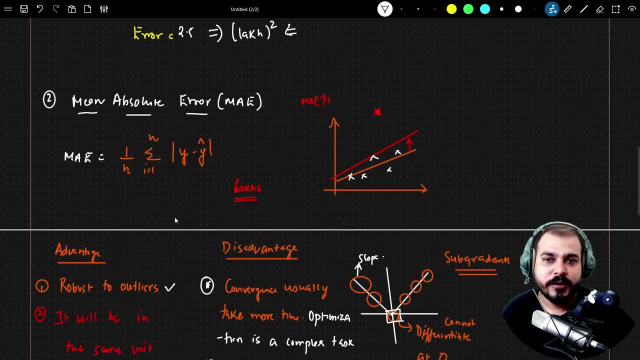 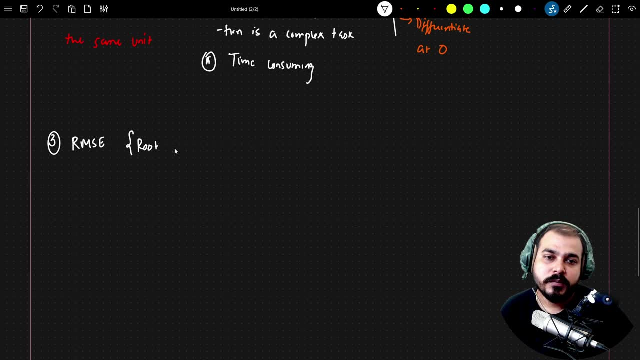 of the advantages and disadvantages with respect to M a me, that is mean absolute error. now let's go ahead with respect to third one, which is called as error. so here I'm just going to write it as root: mean squared error. now, here we can definitely write R ma c as root of a missy. R ma c is coming as the root of a missy. 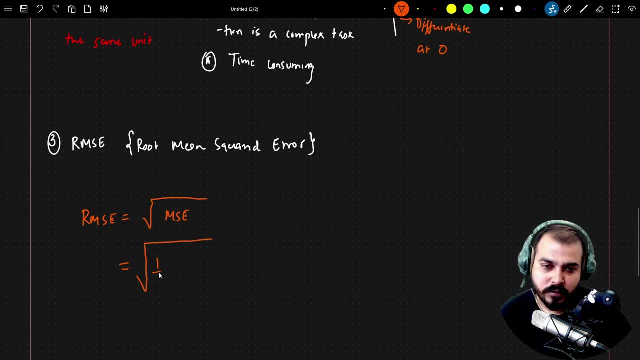 so if i say root of mse, what it is, it is nothing but root of 1 by n. summation of i is equal to 1 to n. y of i minus y of i hat whole square. okay. so this is the entire formula with respect to. 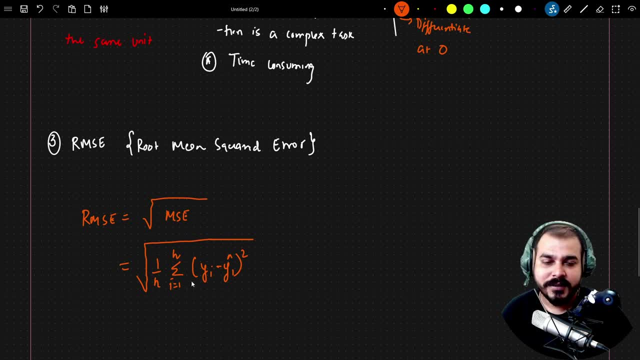 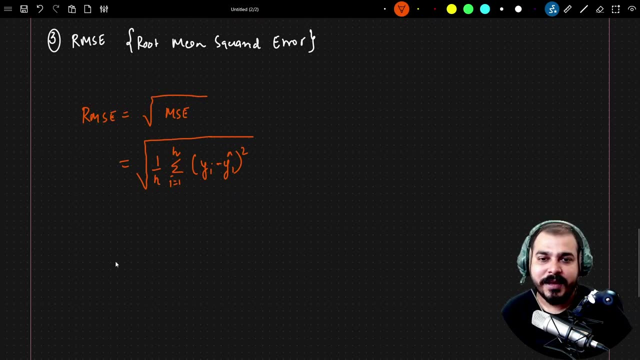 our mse again. uh, in this, uh, what will be the benefit? one benefit that i can definitely compare, uh, since i'm doing the square root, right, so initially in mse it was not in the same unit, right? so first advantage that i would like to call about is that first advantage here: the values that 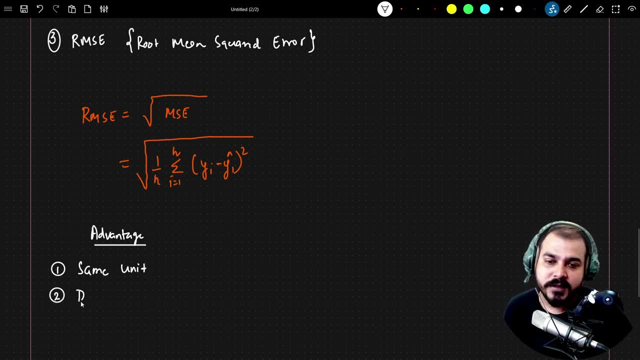 you are getting is in the same unit. second thing: this is obviously differentiable. okay, since here also you will be anyhow getting a gradient descent. but the major disadvantage if i try to talk about is that, since we are again doing squaring here, it is not robust to outline. 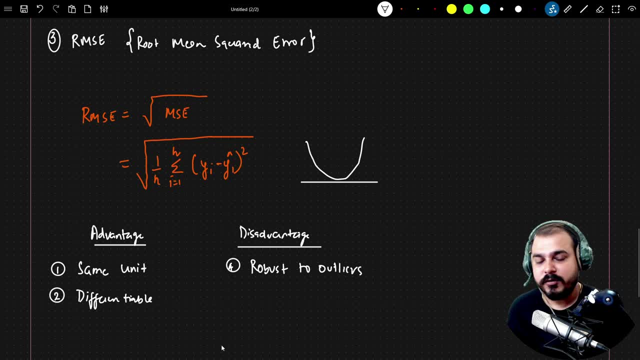 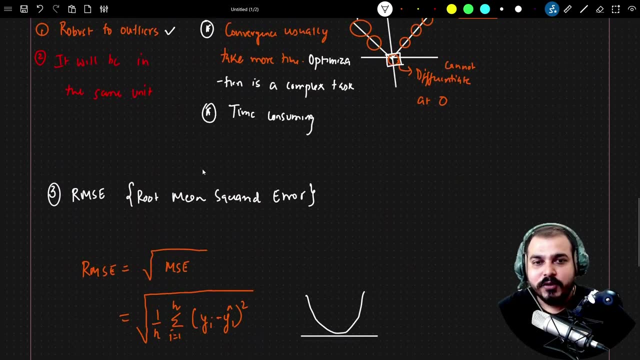 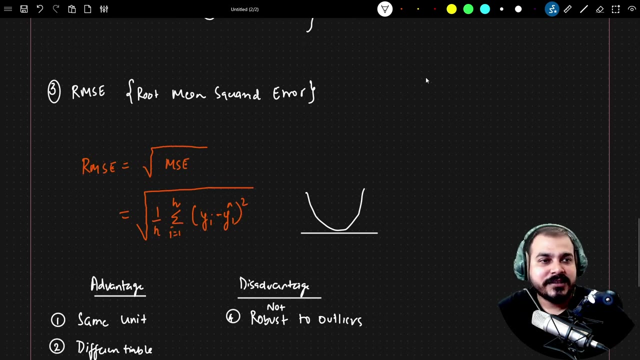 okay, not robust to outliers. now we have learned about this. all three techniques. at the end of the day- you may be considering krish, which one should we use. should we use ma he, mse or rmse? my answer will be that, guys, as a starter we should try to look on all three of them right: rmse, all three. 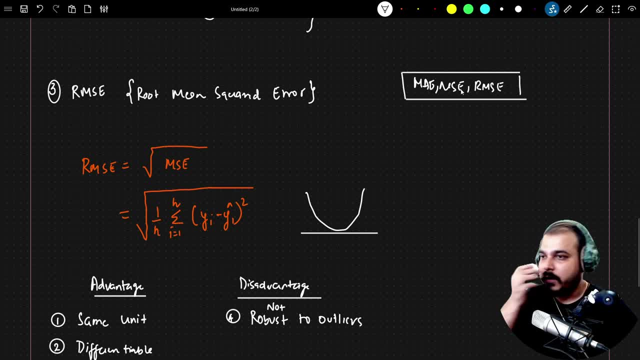 of them. so whenever you'll also be seeing that in further, whenever i try to create any linear regression model, i will also be showing you the errors that is going to come, because, see, once we probably create a best fit line obviously, let's say, if there are some data points, first of all i will try to create. 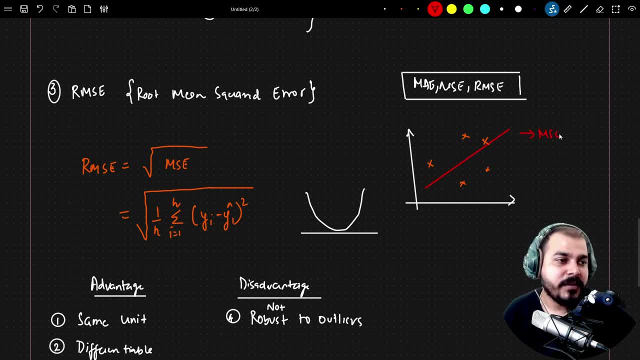 a best fit line, then what i'll do? i will try to calculate the mse, the mean squared error, the mean absolute error and rmse, and after this i will also try to check the performance of this model with the help of r square and adjusted r square, so as a 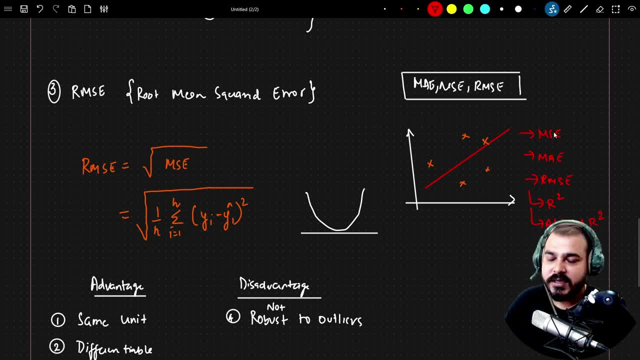 starter. i will also be showing you the errors that is going to come, because, see once, we probably get this all. well, as a starter, you should try to focus on all these things and try to see the performance param- uh, performance metrics- that you are able to get, but all this in combined totally. 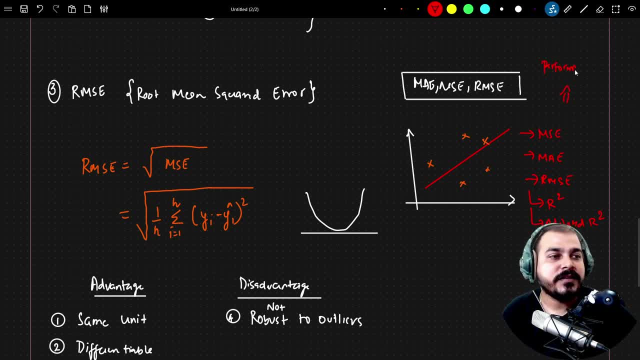 will basically become my performance metrics that i'm specifically going to use. okay, similarly, in classification problem you have different performance metrics but, as mentioned over here, you have to focus both on. you have to focus on all the metrics like performance, mean squared error, mean absolute error, rmsc, r square and adjusted r square. but if someone asks you to perform the function, your prediction is going to be used for the performance of this other one. you may not see the performance matrix you're able to get as the one. you are doing all the data as the one you have spent in the previous lecture, which is the data that is being thanks to the problem. 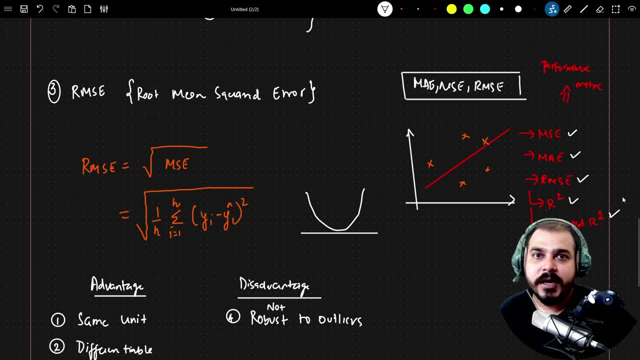 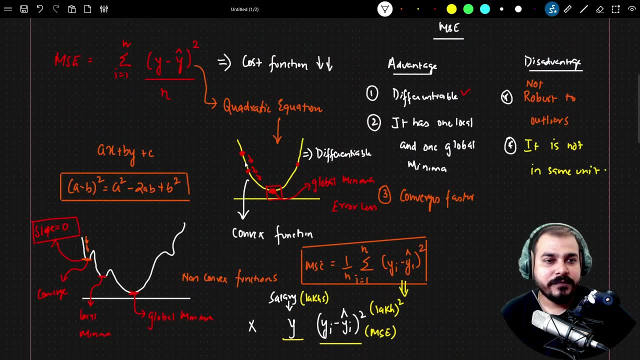 here and i have enhanced this data, so the i will also use one of these data. two, i will use R square and register R square. but if someone asks you in an interview question, why should you use MAC when compared to MAE, then you know that you have to tell the answer that it is very 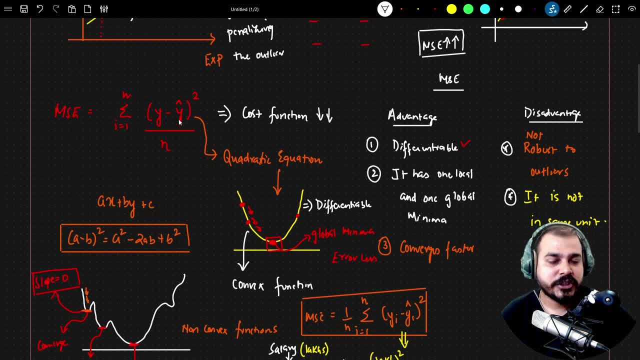 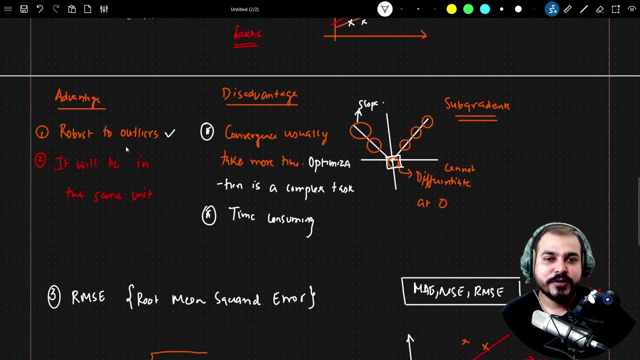 differentiable because the curve that you're going to get because of this quadratic equation it has one and local and one global minima. it converges faster, suppose. if they say that, what about MAE? then you should say that MAE, most advantage thing is that it is robust to outliers. 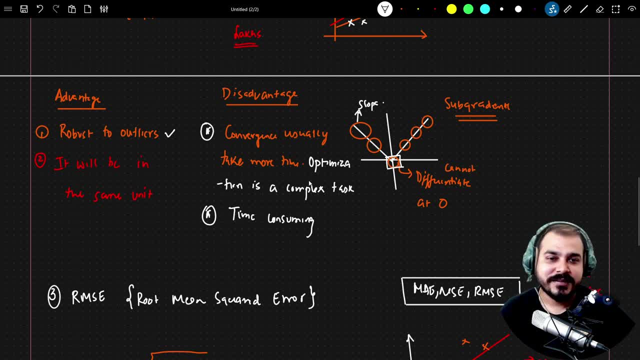 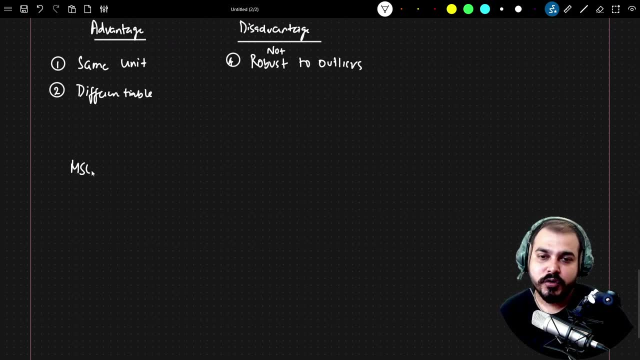 right and the convergence usually take more time. this is the disadvantage, right. and then why should we use RMSE? so this is the specific question. so the question that may come is that when should you use MAC versus when should you use MAE versus when should you use RMSE, and the other question. 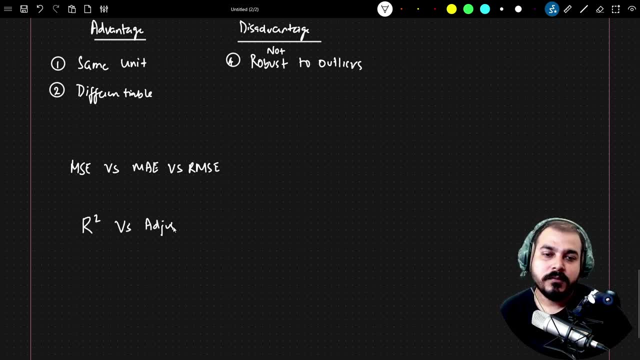 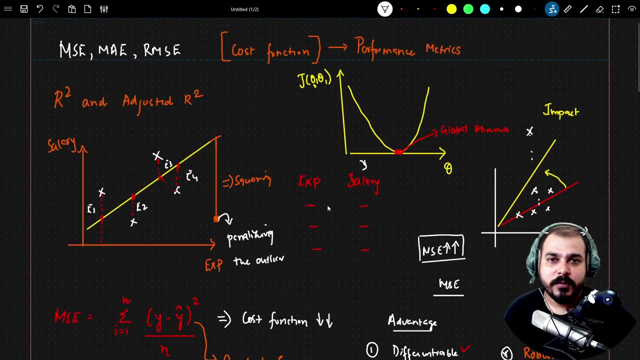 is that? when should you use R square versus adjusted R square? so these are the two important questions that may come in up in the interview, right? so I hope you have understood all the performance metrics till now in this video. we have covered MAC, MAE, RNMSE. now we are going to. 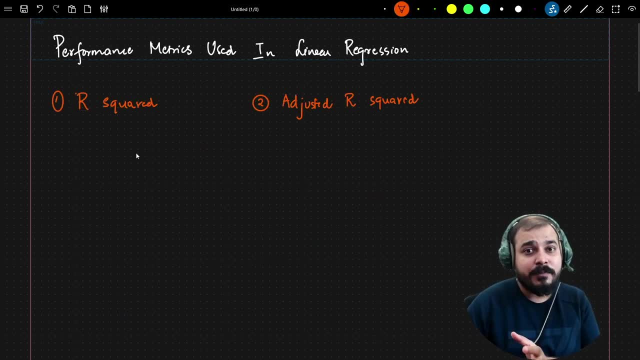 understand some of the performance metrics that is used to determine whether the model is good or not for a specific problem statement, and the metrics that will basically be used is something called as R squared and adjusted R square. now let us understand what exactly R squared is, and you know what is adjusted R square. what is the exact? 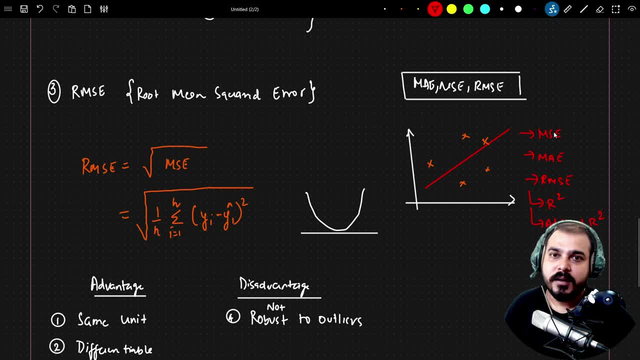 you should try to focus on all these things and try to see the performance parameter, performance metrics that you are able to get. but all this in combined totally will basically become my performance metrics that i'm specifically going to use. okay, similarly, in classification problem, you have different performance metrics but, as mentioned, 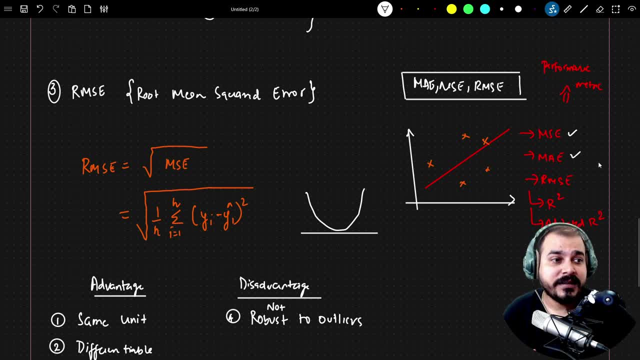 over here. you have to focus both on. you have to focus on all the metrics like performance, mean squared error, mean absolute error, rmse, r square and adjusted r square. but if someone asks you in an interview question, why should you use mse when compared to ma, then you know that you. 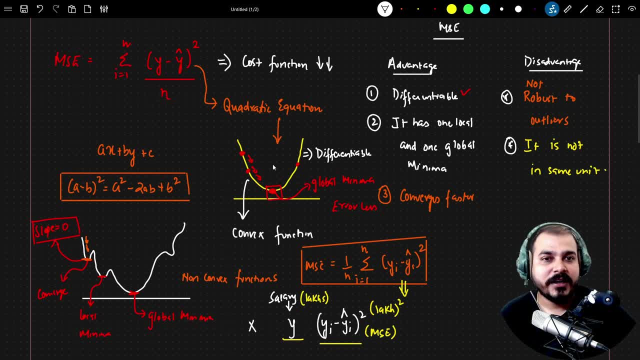 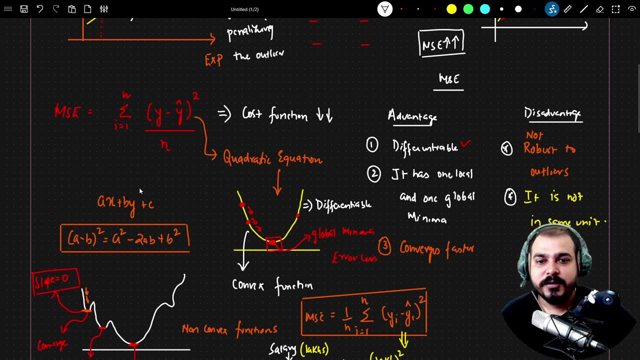 have to tell the answer that it is very differentiable, because the curve that you're going to get because of this quadratic equation, it has one and local and one global minima. it converges faster, suppose. if this is the case, then you have to tell the answer that it is very differentiable. 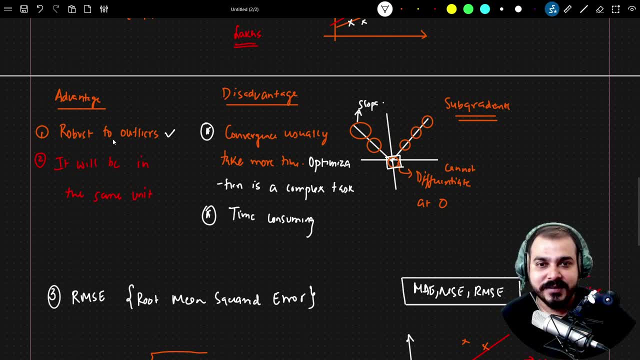 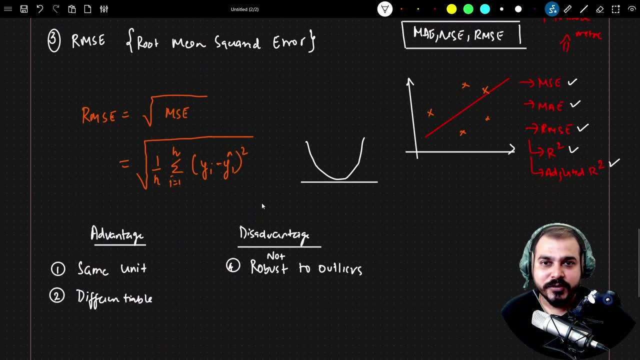 but if they say that, what about ma? then you should say that ma most advantage thing is that it is robust to outliers, right, and the convergence usually take more time. this is the disadvantage, right, and then why should we use rmse? so this is the specific question. so the question that may 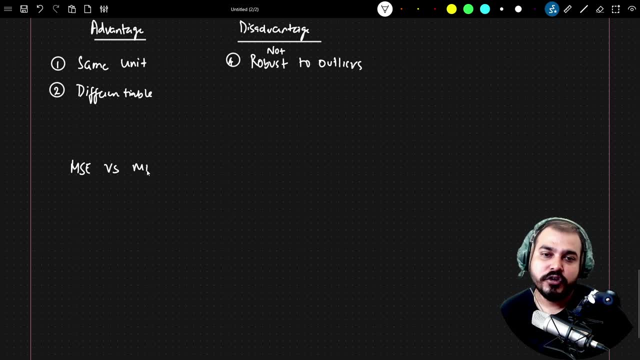 come, is that when should you use mse versus when should you use mae versus when should you rmse? and the other question is that when should you use r square versus adjusted r square? so these are the two important questions that may come in up in the 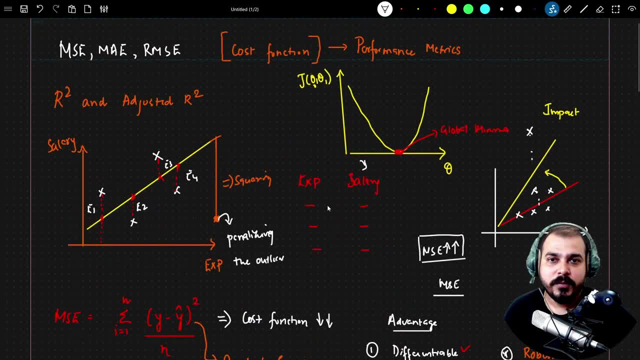 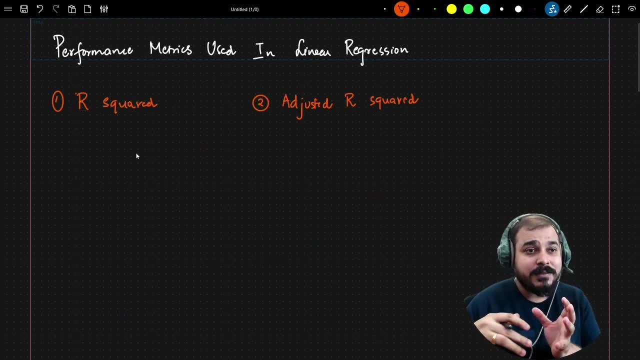 interview right, so i hope you have understood all the performance metrics till now. uh, in this video we have covered mse ma r and mse. now we are going to understand some of the performance metrics that is used to determine whether the model is good or not for a specific problem. 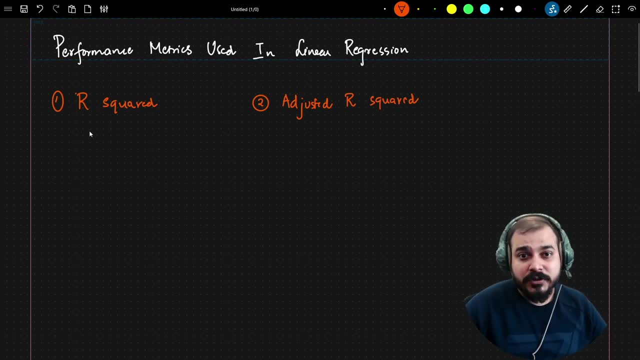 statement and the metrics that will basically be used is something called as r squared and adjusted r square. now let us understand what exactly r squared is and you know what is adjusted r square, what is the exact difference between the two and what is the difference between both of them. now, first of all, let us go ahead and understand about r squared. 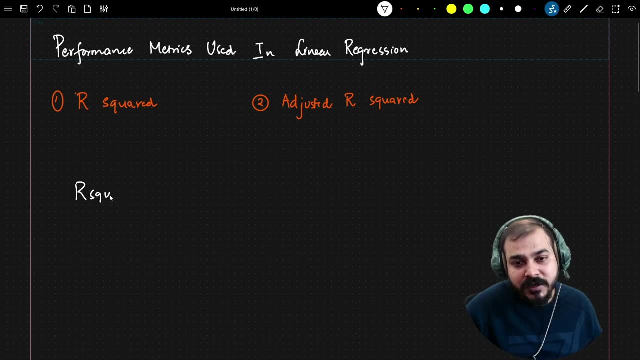 and r? squared is basically given by the formula, which looks something like this: so this is: r squared is equal to 1 minus sum of square residual. i'll talk about what is this: residual and all and this is sum of square total. okay, so here a simple definition that you can probably see. 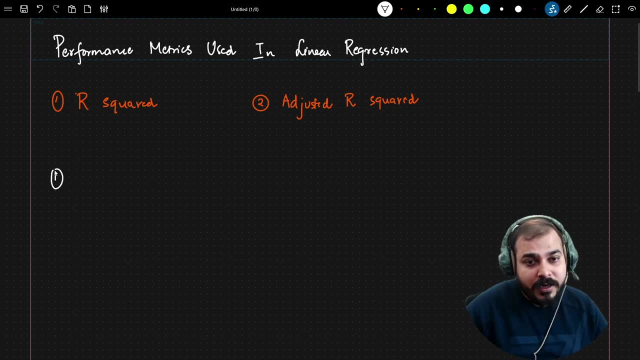 difference between both of them. now, first of all, let's go ahead and understand about R square, and R square is basically given by the formula, which looks something like this: so this is: R squared is equal to 1 minus sum of square residual. I'll talk about what is this: residual and all and this is sum of. 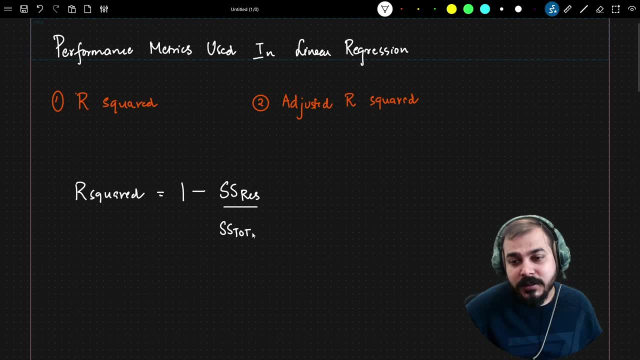 square total. okay, so here a simple definition that you can probably see is that R squared is nothing but 1 minus SS residual, that is, sum of squared residual divided by sum of squared total. okay, now let's understand what is the sum of squared residual. suppose if I say this is my problem statement. 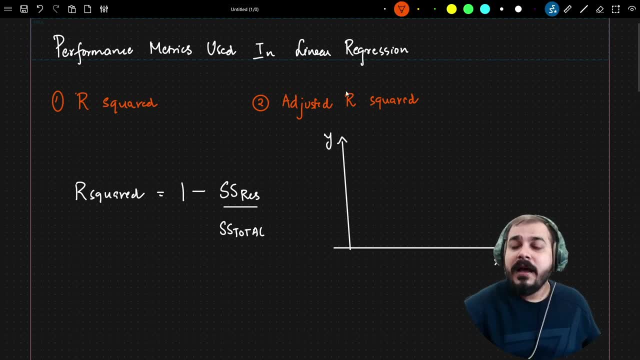 let's say, this is my x-axis, y-axis, okay, and i have some of the data points which looks like this, okay, which looks like this: okay. i'm just drawing some data points over here. our main aim is that we need to find out the best fit line. so if we are trying to find out the best fit line, with respect, 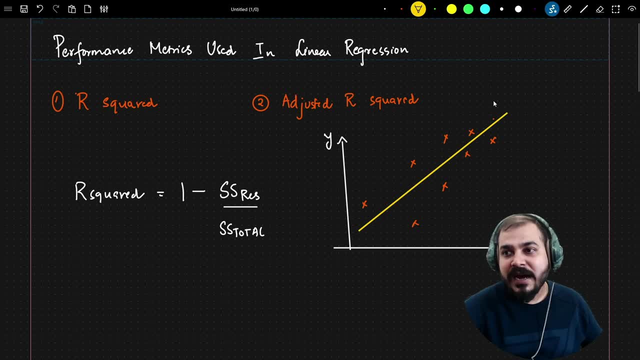 to these orange points. these are my true output, right? I specifically say: all these points belongs to y of I, right, y of I are basically my true outputs right now. similarly, with respect to to this particular point, the predicted point is nothing but this part, right? so this I can basically. 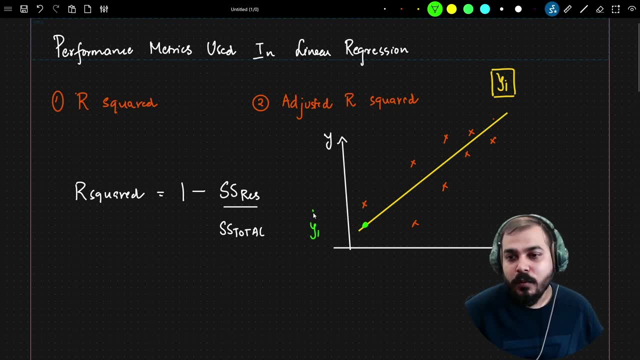 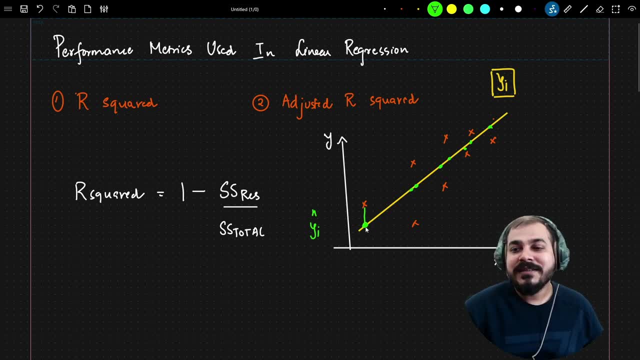 out the difference between them then, in short, I am basically saying that as this is basically my residual, okay, residual or error. so if i probably try to find out this particular distance, this particular distance, this distance, this distance, this distance and this distance, this is basically the residual. okay, now understand the definition over here i am basically writing 1 minus sum of 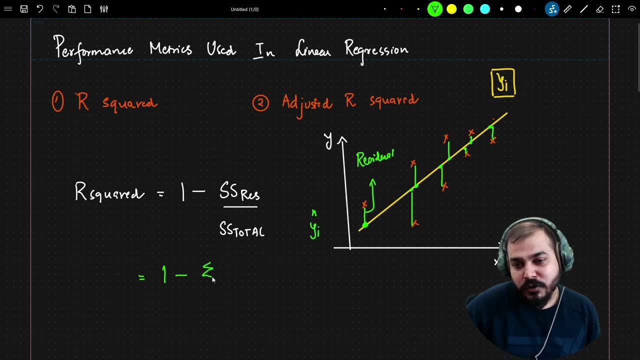 square residual. so i can basically write this as with this notation, that is summation of y of i minus y of i hat whole square, right? so, in short, what i'm doing, i'm basically trying to find out the difference between y of i and y of i hat, okay, and i'm doing all the summation of all this. 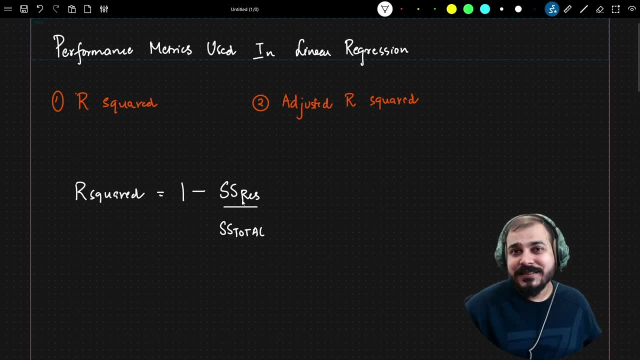 is that r squared is nothing but one minus ss residual, that That is sum of squared residual divided by sum of squared total. OK, now let's understand what is the sum of squared residual. Suppose if I say this is my problem statement, let's say this is my x-axis, y-axis. 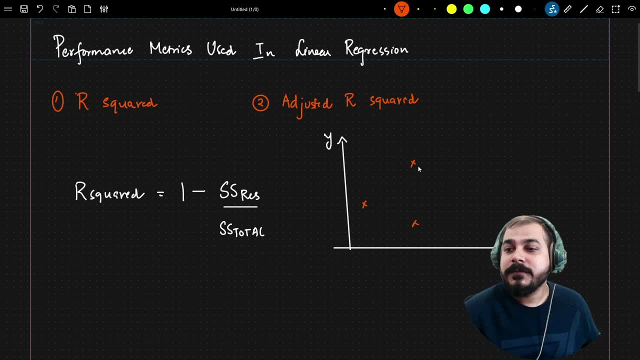 OK, and I have some of the data points which looks like this: OK, Which looks like this: OK. I'm just drawing some data points over here. Our main aim is that we need to find out the best fit line. So if we are trying to find out the best fit line with respect to this orange points, 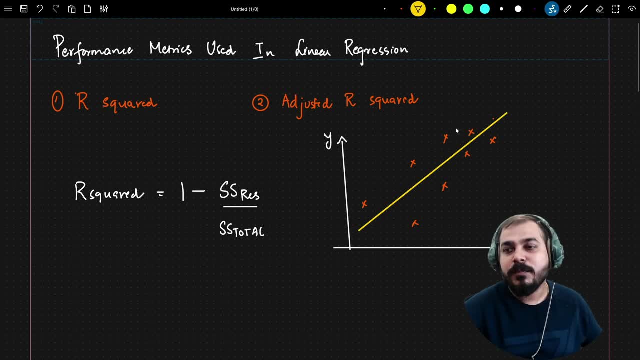 these are my true output, right. I specifically say: all these points belongs to y of i right. y of i are basically my true outputs right Now. similarly, with respect to this particular point, the predicted point is nothing but this part, right. 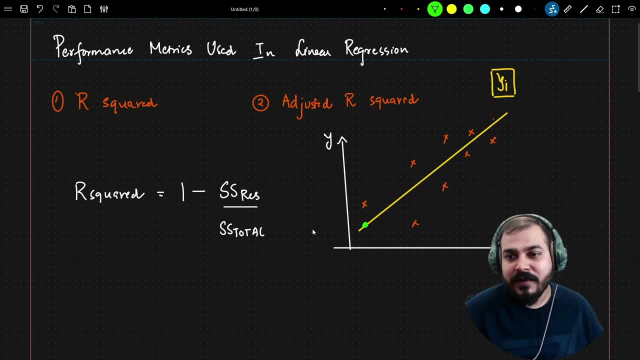 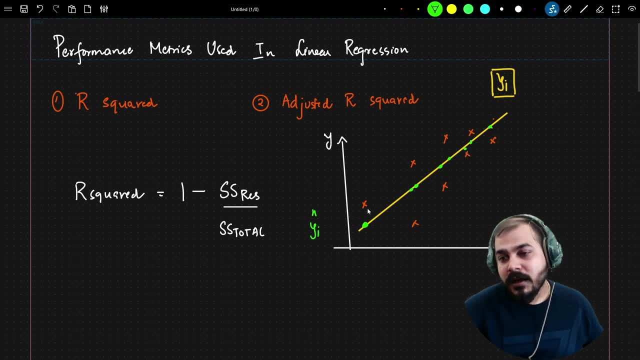 This is my predicted point. So I'm just drawing all my predicted point Now, whenever I try to find out the difference between them. then, in short, I am basically saying that, as this is basically my residual, OK, Residual or error. 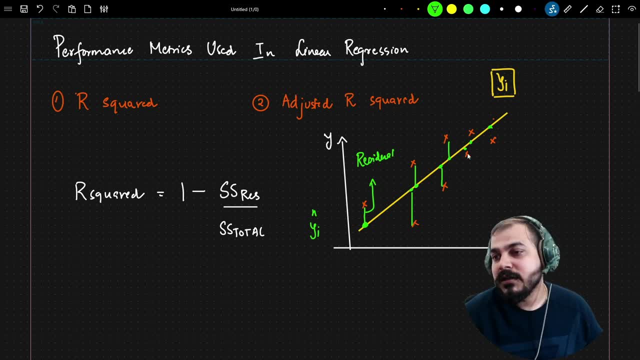 So if I probably try to find out this particular distance, this particular distance, this distance, this distance, this distance and this distance, this is basically the residual. OK, Now understand the definition. over here I am basically writing 1 minus sum of. 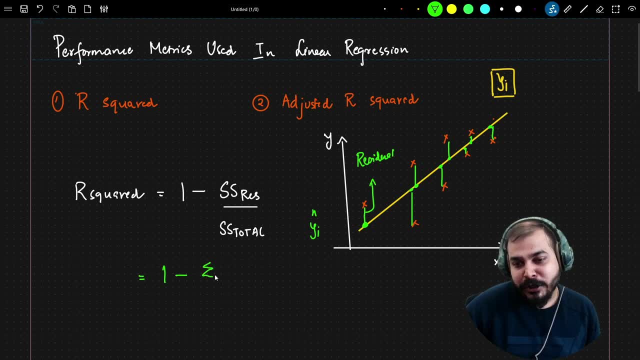 So I can basically write this as with this notation: that is summation of y of i minus y of i hat, whole square right. So, in short, what I'm doing? I'm basically trying to find out the difference between y of i and y of i hat, OK. 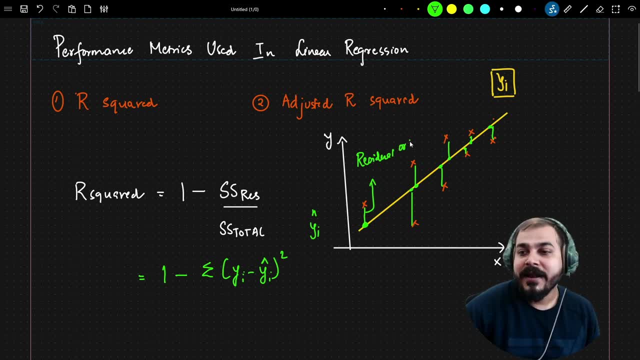 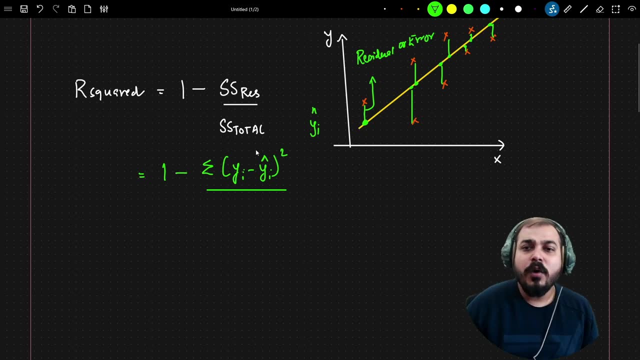 And I'm doing all the summation of all this particular residual or error- I can also say this as errors. OK, Now, this will be divided by sum of square total. Now, what is this sum of square total Now, with respect to this particular point? I hope everybody found out. OK, this is my 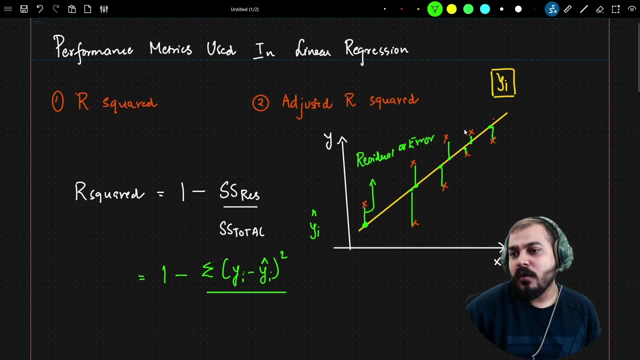 best fit line, But with respect to the y-axis and with respect to all these y points, if I try to calculate the average, OK. So if I try to calculate the average, then you may probably be seeing that y of i average will come with respect to this specific point. OK, 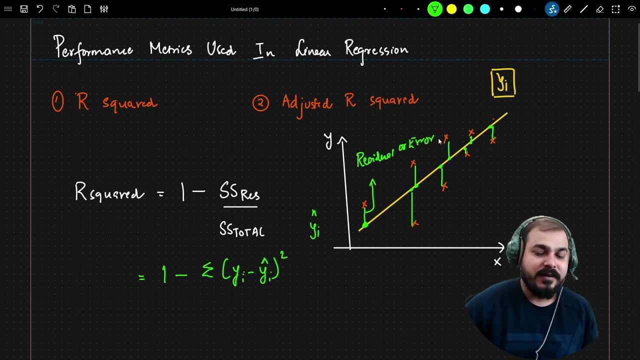 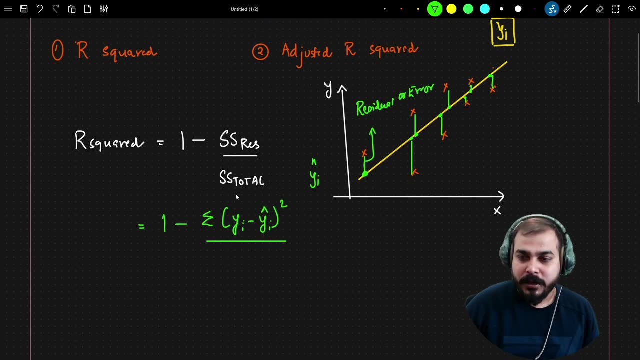 particular residual or error- i can also say this as errors. okay, now, this will be divided by sum of square total. now, what is this sum of square total now, with respect to this particular point? i hope everybody found out. okay, this is my best fit line, but with respect to the y axis, 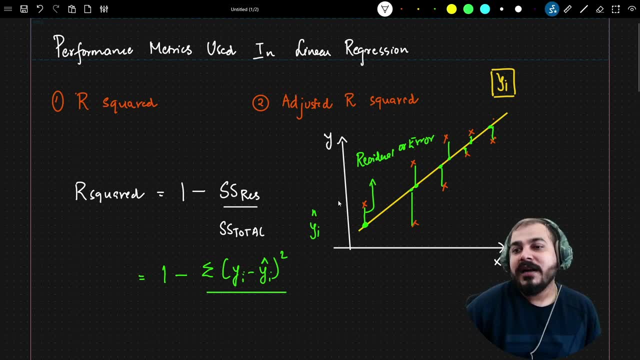 and with respect to all these y points, if i try to calculate the average? okay. so if i try to calculate the average, then you may probably seeing that y of i average will come with respect to this specific point, okay. or let's say, i'm just trying to calculate all the y of i points, i'm just taking. 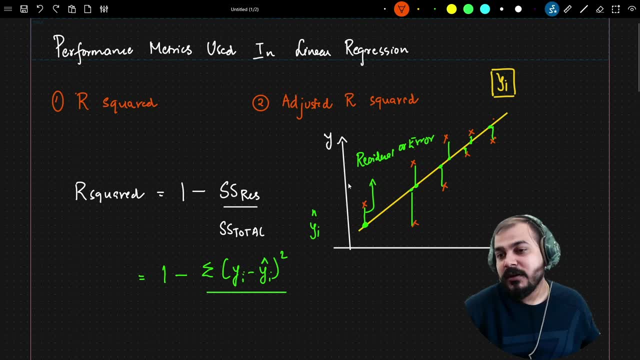 all the y of i points and i'm just calculating the average now and with respect to this kind of distribution, let's let's assume that my y of i is basically getting passed over here. this y of i hat i will say okay. so this basically indicates this is nothing but average of the true points. that is y of i okay, average of all the y of. 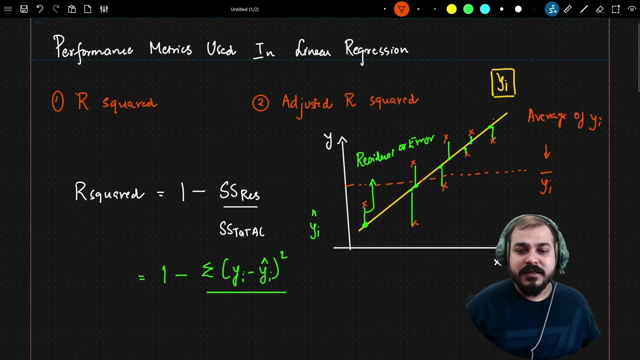 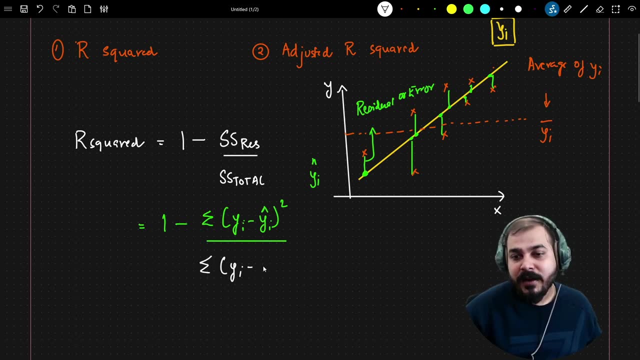 i now this sum of square. total basically means, if i really want to give it in a mathematical notation, this is nothing but summation of y of i minus y hat y of i hat whole square. so this basically means that we are trying to find out the difference between the true point and this specific point. 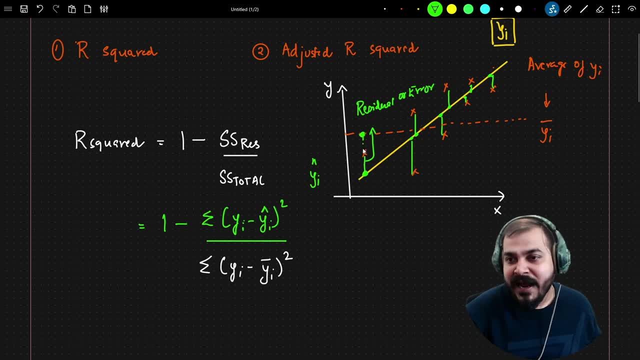 which is basically indicated by y of i hat. y of i hat is nothing, but it is the average point. okay, so from here to here, i'll calculate a difference. then, from here to here, i'll calculate the difference. similarly, here to here, i'll calculate the difference. here to here, i'll calculate the difference. here to here, i'll. 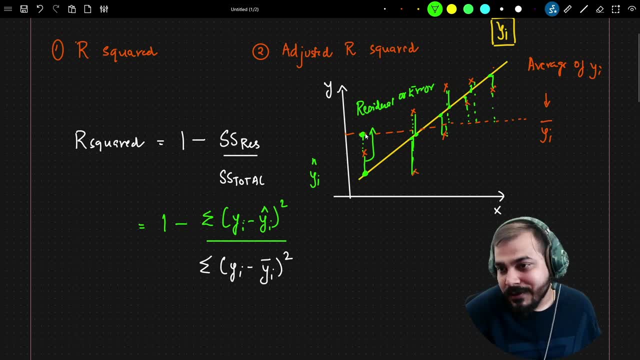 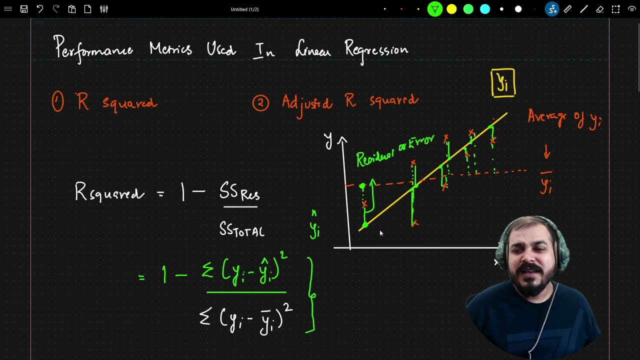 calculate the difference here to here and here to here. okay, so this orange line that you see, this is basically the mean of all the y of i points. okay, so this basically will be giving my r squared value. okay, now, here you can clearly see that, obviously, just by a simple understanding, right, you can definitely see that y of i minus y. 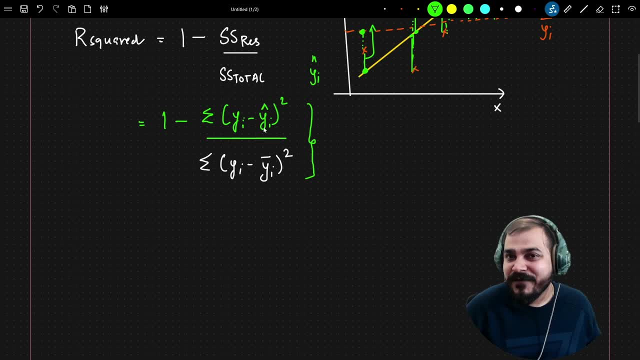 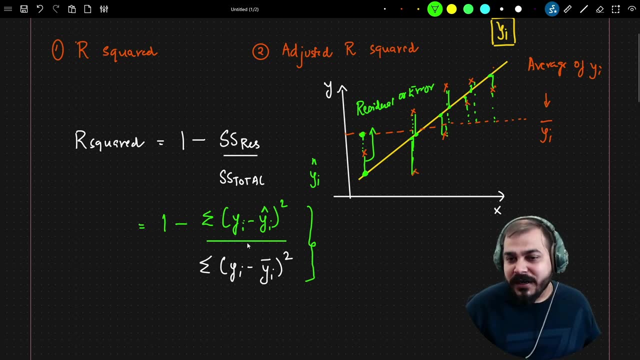 of. i hat whole square, this residual, this, this difference of the residual, because my best fit line passes through almost near to all the true points, right, so this particular difference will be smaller number when compared to this particular difference. right, because this is with respect to the average, this specific line, and obviously the distance will be quite big. so here i can. 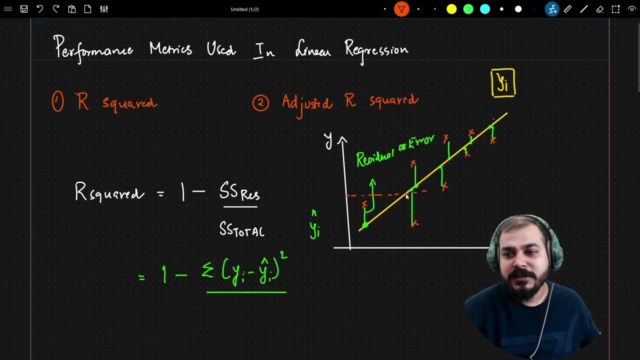 Or let's say: I'm just trying to calculate all the y of i points. I'm just taking all the y of i points and I'm just calculating the average. Now, with respect to this kind of distribution, let's assume that my y of i is equal to 1.. 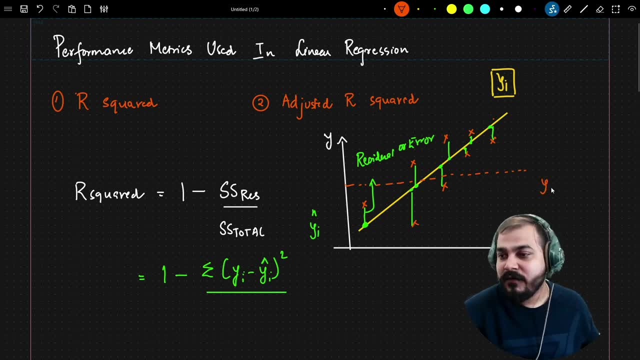 So this y of i is basically getting passed over here, This y of i hat I will say OK. So this basically indicates this is nothing but average of the true points. That is y of i, OK. Average of all the y of i. 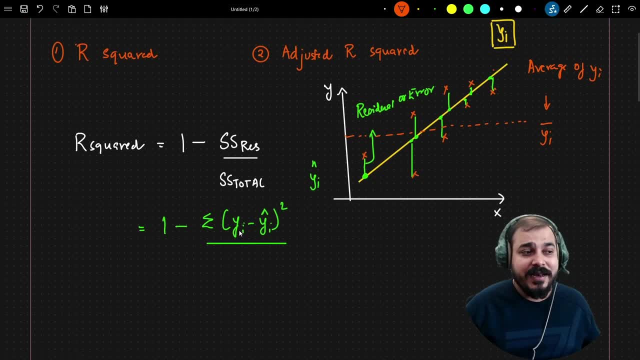 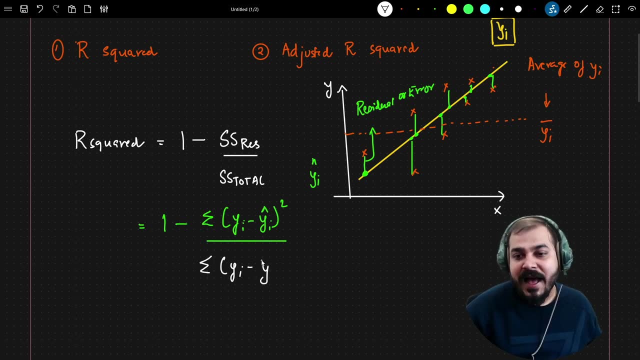 Now this sum of square total basically means, if I really want to give it in a mathematical notation, this is nothing but summation of y of i minus y hat y of i hat whole square. So this basically means that OK. 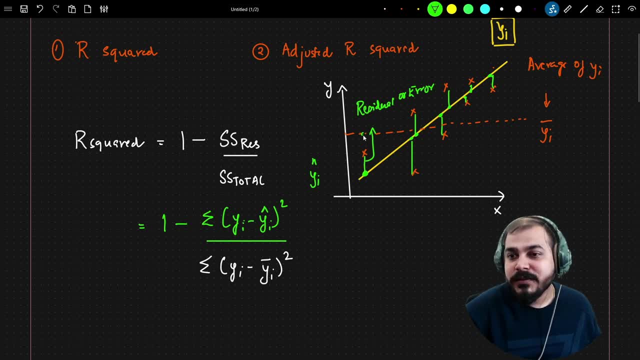 to find out the difference between the true point and this specific point, which is basically indicated by Y of I hat. Y of I hat is nothing, but it is the average point. Okay, So from here to here, I'll calculate a difference. Then, from here to here, I'll calculate the difference. Similarly. 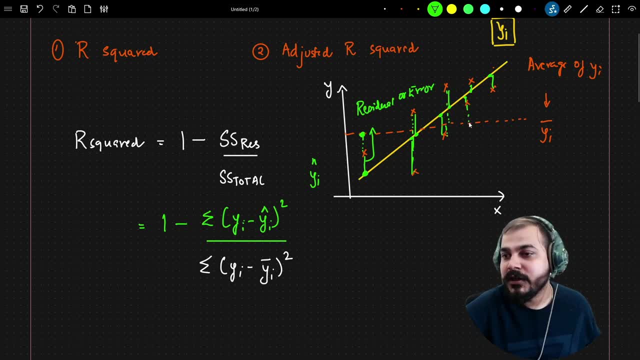 here to here. I'll calculate the difference Here to here. I'll calculate the difference Here to here. I'll calculate the difference Here to here and here to here. Okay, So this orange line that you see, this is basically the mean of all the y of i points. okay, so this basically will be giving. 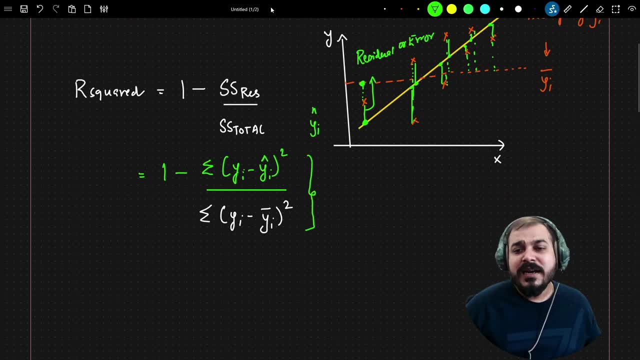 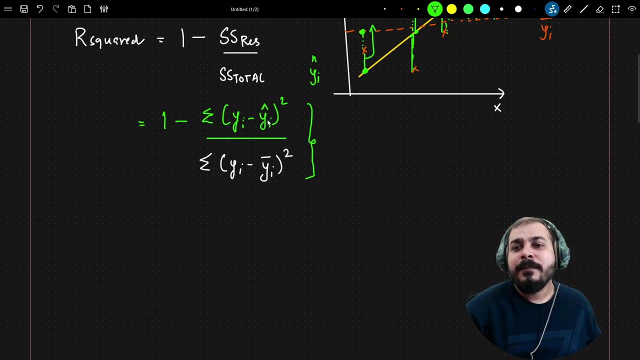 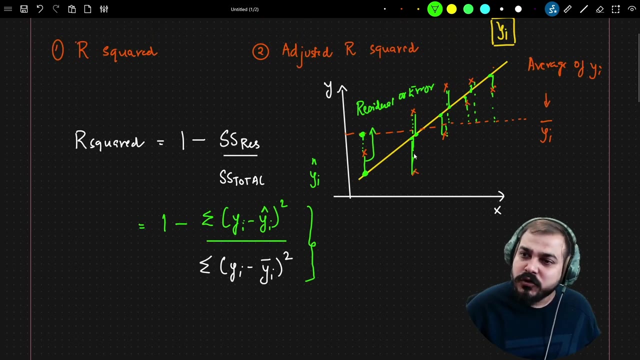 my r squared value. okay, now here you can clearly see that. obviously, just by a simple understanding right, you can definitely see that y of i minus y of i hat whole square, this residual, this, this difference of the residual, because my best fit line passes through almost near to all the true. 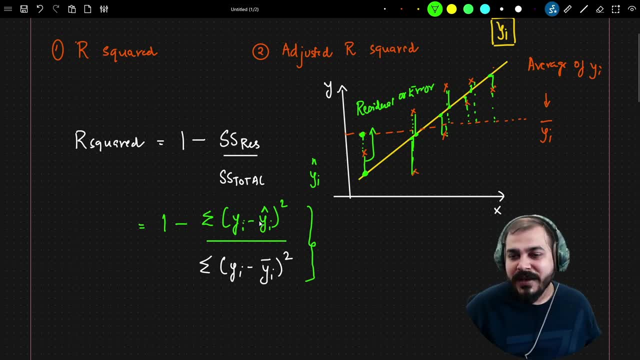 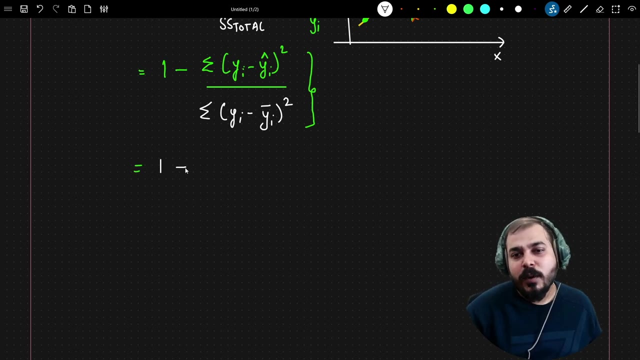 points, right, so this particular difference will be smaller number when compared to this particular difference. right, because this is with respect to the average, this specific line, and obviously the distance will be quite big. so here i can definitely write something like this. i will write that it is. 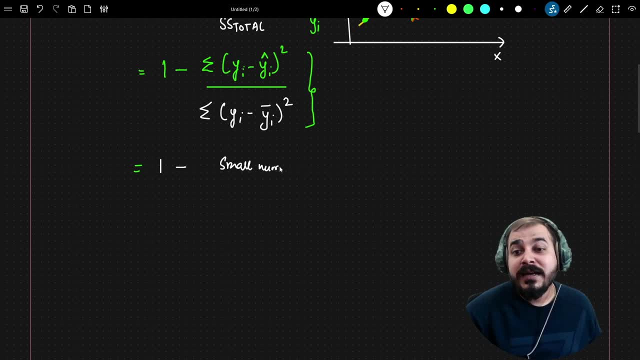 y minus. let's consider: this is a small number when compared to the denominator, right? so the denominator will be a bigger number, right? small number divided by bigger number. so now, when we do this, we are going to get a bigger number, right, so we are going to get a bigger number. 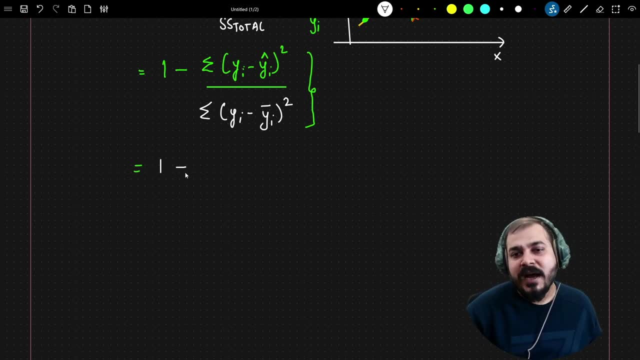 definitely write something like this. i will write that it is y minus. let's consider this is a small number when compared to the denominator, right? so the denominator will be a bigger number, right? small number divided by bigger number. so now, when we do this kind of division, 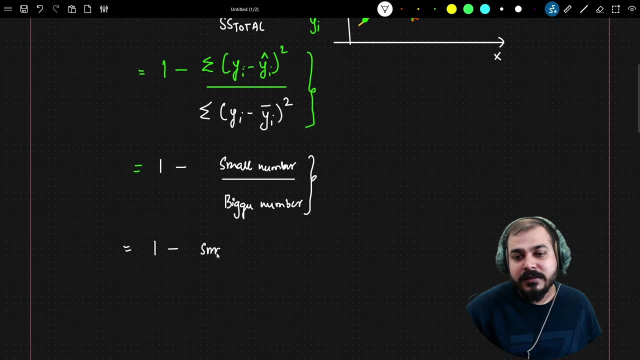 obviously we are going to get a smaller number itself, a smaller number itself, right? so let's consider if this numerator is a smaller number and denominator is a bigger number. obviously, when we try to find the denominator, it will be a smaller number. so let's consider this. 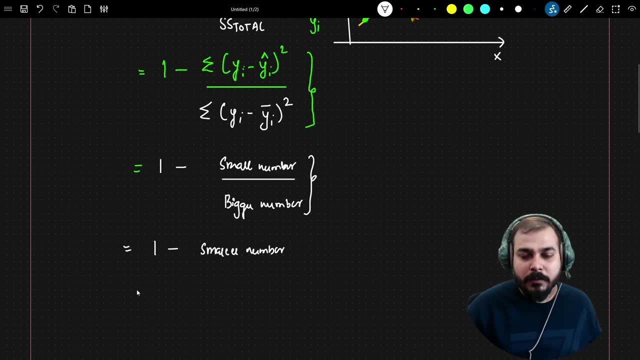 out the division of this two. obviously we are going to get a smaller number. so 1 minus smaller number will be, you know, very much near to 1 itself, right, it will be approximately near to 1. so let's consider that, suppose if i'm getting 0.70 right. so this basically indicates that i am actually 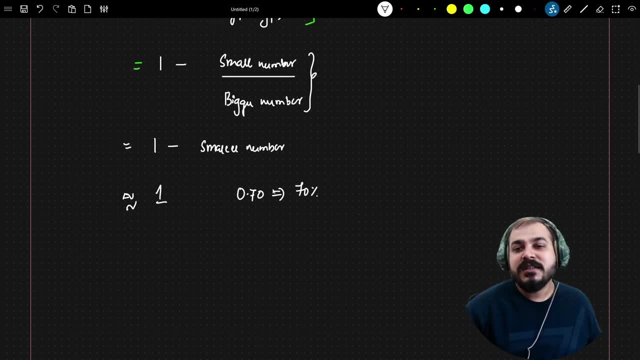 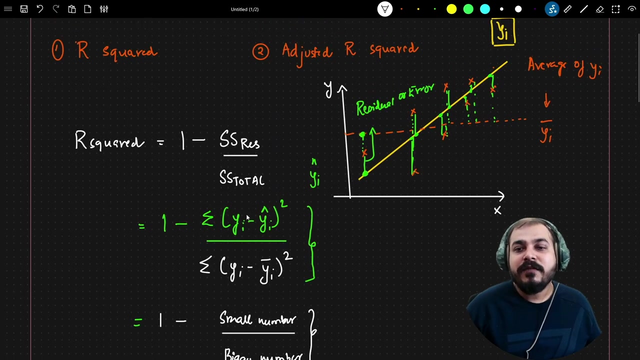 having 70 accuracy, right, suppose. if i get this specific difference is somewhere on 0.85, this basically indicates that i'm getting a 85 accuracy, suppose. if i say it is 0.90, i'm actually getting a 90 accuracy, right? so with the help of r squared, we are able to find out how our model is performing. 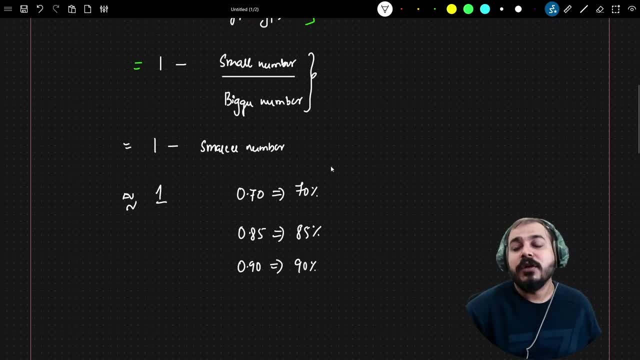 right and more this value, understand more this value. it is towards one right more accurate. my model is more accurate. my model is more accurate. my model is. my linear regression model is okay, but there is something called as overfitting okay, which we will probably discuss as we go ahead. 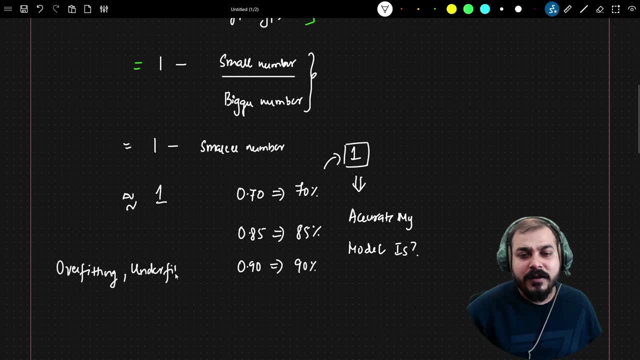 uh, we are going to discuss about overfitting and underfitting. just in some time. we'll discuss about it how we need to identify whether the model is basically getting overfitting or not. for that we really need to understand what is true in data, test, data, validation, data. just give me some time. we'll discuss about that as we 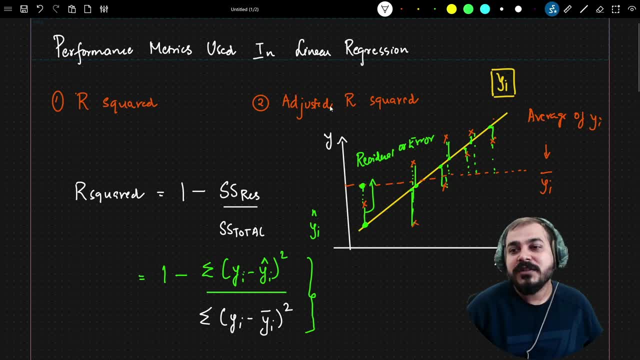 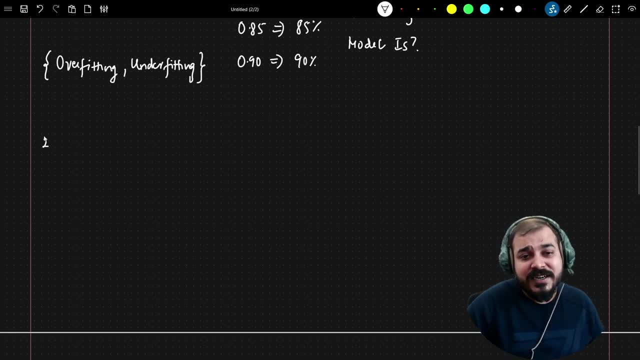 go ahead now. let's go ahead and understand about the second performance matrix, which is called as adjusted r squared, now with respect to existed r squared. okay, how it is basically different. that also we are going to discuss with respect to the r squared. so here i'm just going to write my 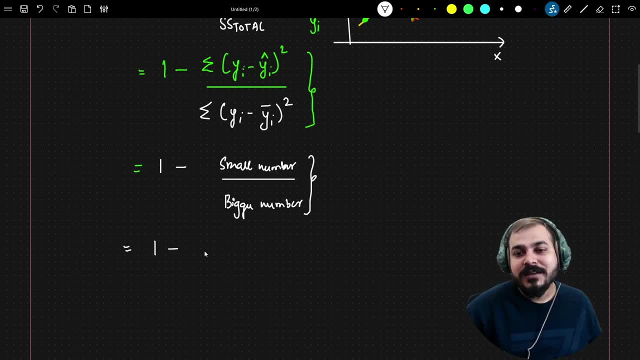 this kind of division, obviously we are going to get a smaller number itself, a smaller number itself, right? so let's consider if this numerator is a smaller number and denominator is a bigger number. obviously, when we try to find out the division of this two, obviously we are going to get a smaller. 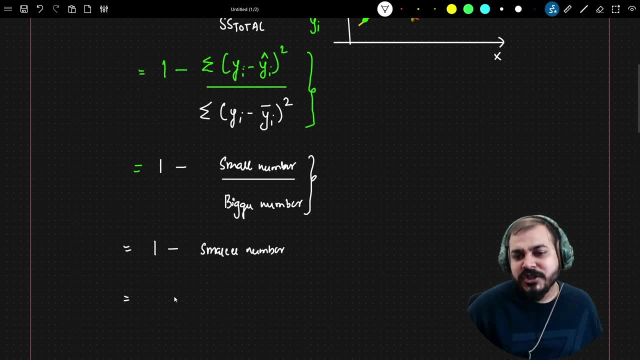 number. so one minus smaller number will be, you know, very much near to one itself, right? it will be approximately near to one. so let's consider that, suppose. if i'm getting 0.70 right, so this basically indicates that i have a smaller number, right? so i'm going to get a smaller number, right? 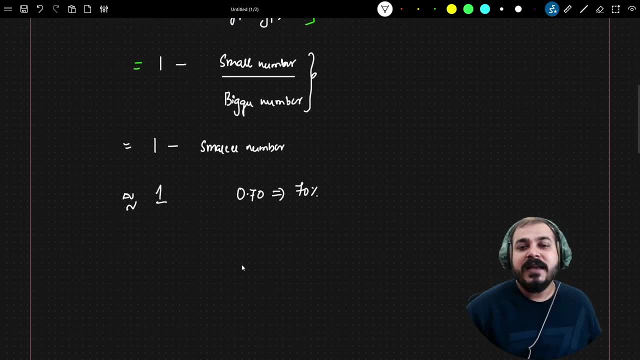 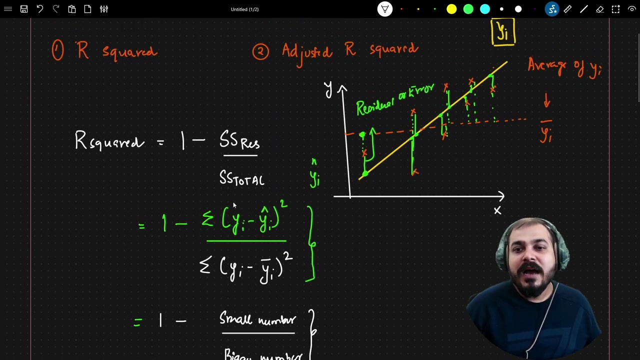 suppose, if i get this specific difference is somewhere on 0.85, this basically indicates that i'm getting a 85 accuracy. suppose if i say it is 0.90 i'm actually getting a 90 accuracy right. so with the help of r squared, we are able to find out how our model is performing right and more. 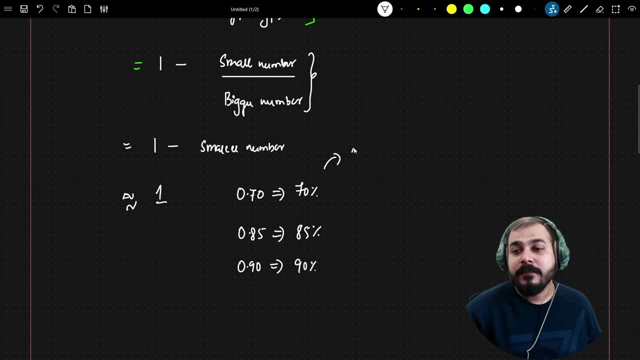 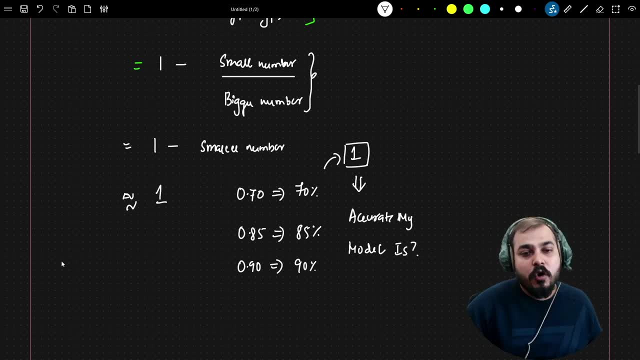 regression model is okay, but there is something called as overfitting, okay, which we will probably discuss as we go ahead. uh, we are going to discuss about overfitting and underfitting. just in some time we'll discuss about it how we need to identify whether the model is basically getting overfitting. 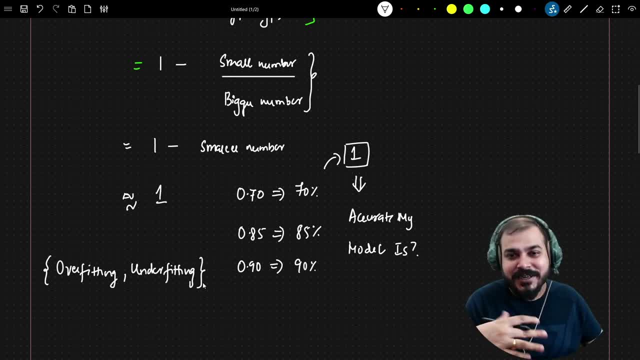 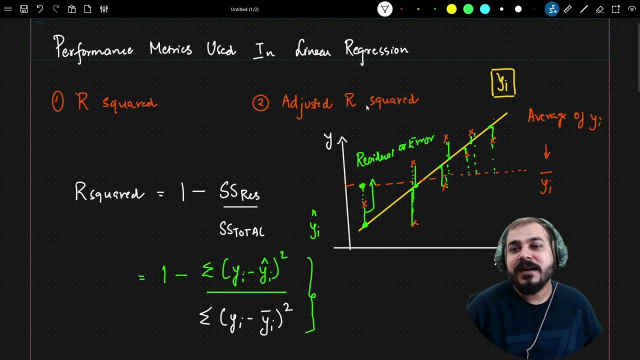 or not. for that we really need to understand what is true in data test, data validation data. just give me some time. we'll discuss about that as we go ahead. now let's go ahead and understand about the second performance matrix, which is called as adjusted r squared now with respect to adjusted 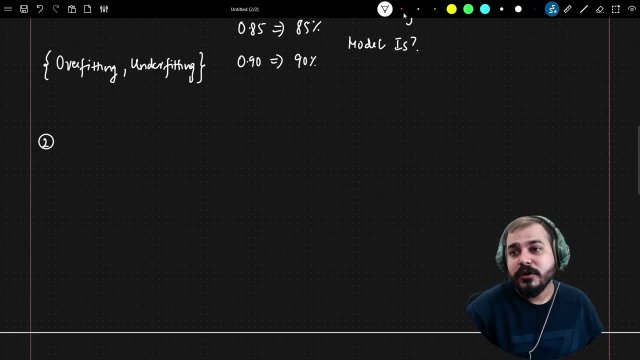 r squared. okay, how? it is basically different. that also we are going to discuss with respect to the r squared. so here i'm just going to write my adjusted r squared: okay, r squared. now, guys, if i consider this specific example, let's say: i have in my data set. okay, i have in my data set. 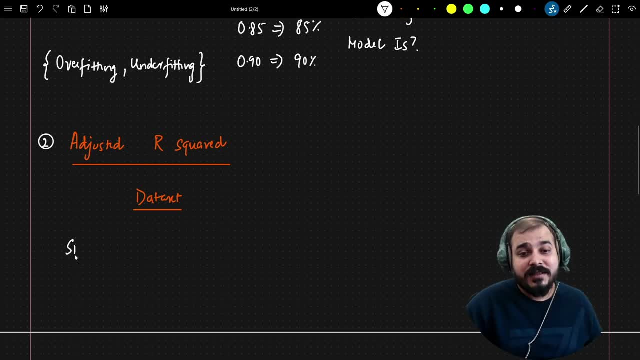 one feature which is called as, let's say, one of the feature is like size of the house. okay, size of the house. suppose this is my data set. i need to really predict what is the price of the house. okay, so i need to predict this specific thing. let's say, i have one of the feature which 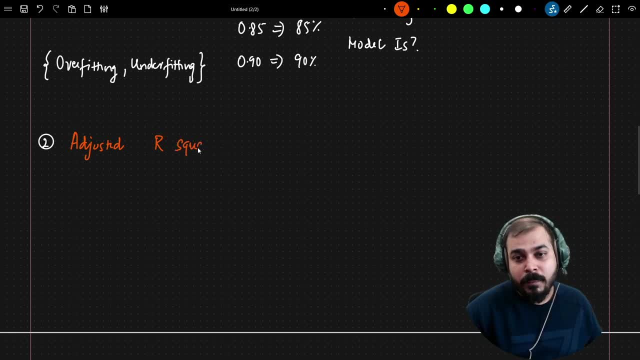 adjusted r squared. okay, r squared. now, guys, if i consider this specific example, let's say i have in my data set- okay, i have in my data set one feature which is called as. let's say, one of the feature is like size of the house. okay, size of the house. suppose this is my data set. i need to. 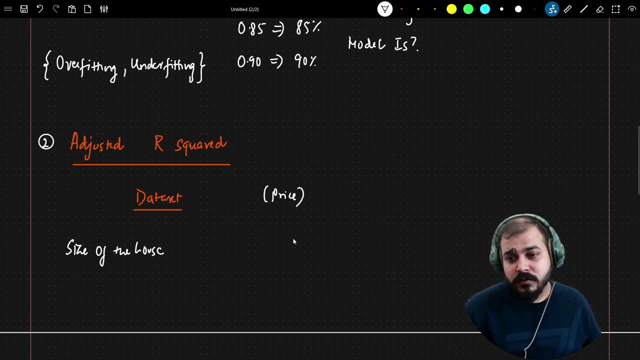 really predict what is the price of the house. okay, so i need to predict this specific thing. let's say i have one of the feature which is called as size of the house, so i am definitely going to write price over here. now suppose if i have size of the house and the price of the house. 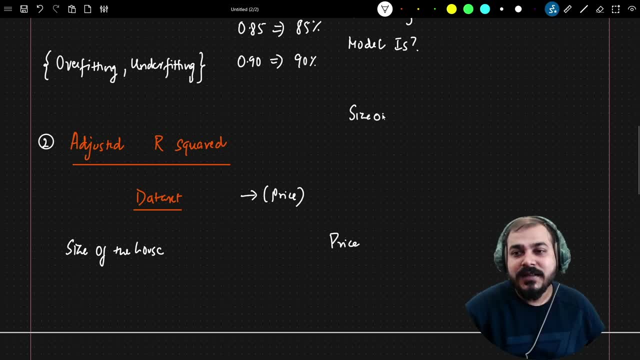 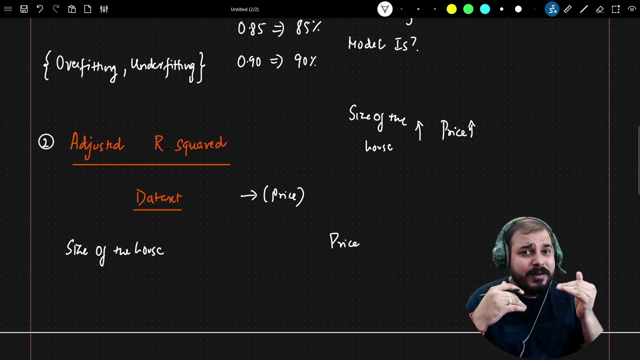 as we know that as the size of the house, as the size of the house increases, increases, my price is also going to increase. so there is a direct correlation between size of the house and price of the house, and this is usually happens in any any state or any region that you 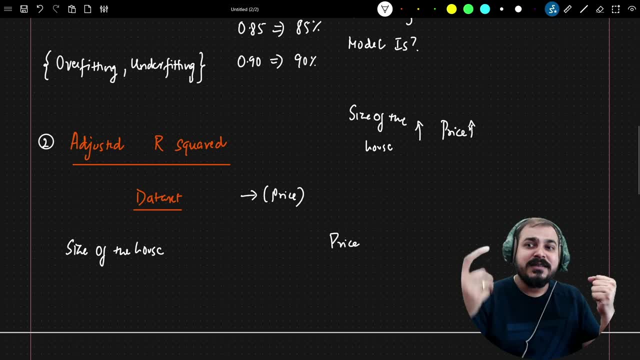 are probably seeing. you stay right. the size of the house as it increases, the price also increases, so, and similarly, when the size of the house decreases, the price also decreases. so here we can definitely find something called as a positive correlation, right, positive correlation, a good positive correlation. 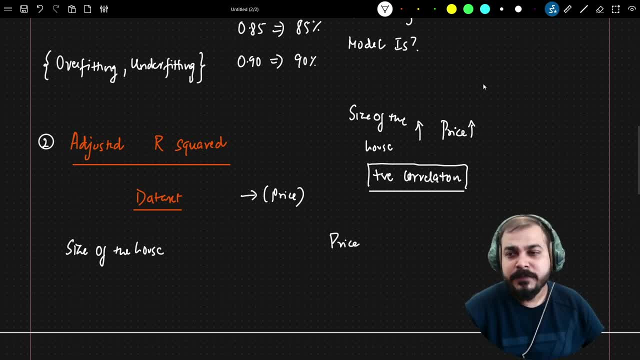 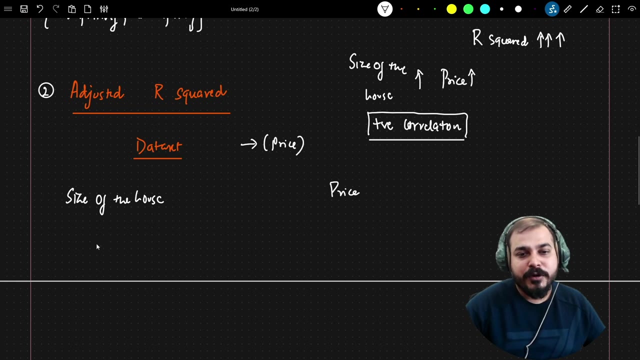 so when we have, in this particular case, a good positive correlation, then what happens? my r squared value probably increases, right, let's say, this value basically increases. now, let's say, in this particular case, when i'm using these two features, my- and let's say that i have actually computed my r squared, my r squared value, that was. 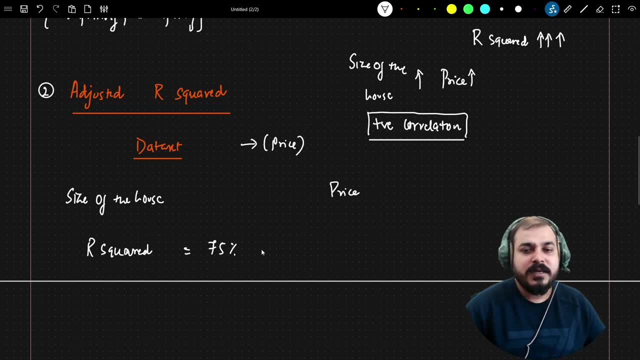 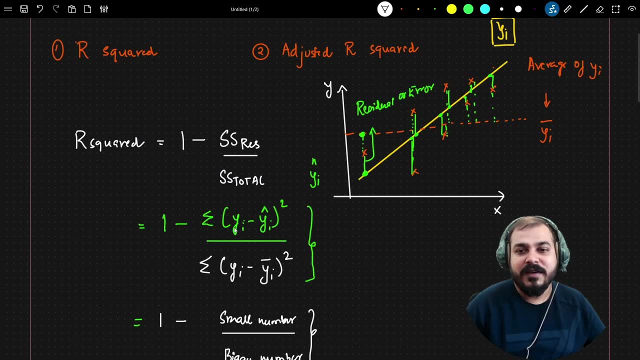 coming was somewhere around. you know, 75. let's say 75 is nothing but 0.75. with the help of the same formula- okay, let's say, with the help of this same formula that we have used over here- we got 0.75 now. 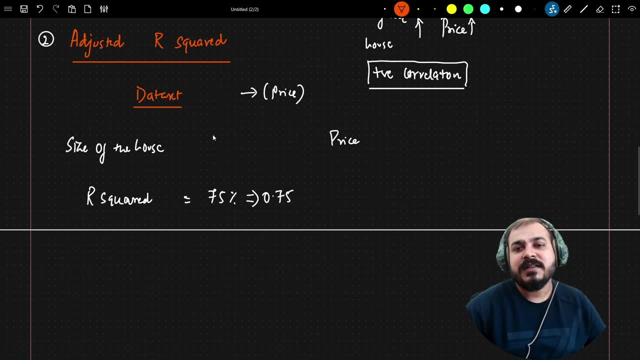 what happened is that, let's say, i included one more feature after the size of the house, i said number of bedrooms. now you know that as the number of bedrooms increases, right, the price is also going to increase. so from this i can definitely say: as my number of bedroom. 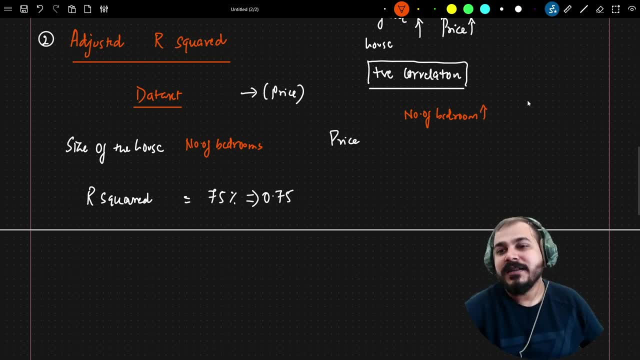 and this is just a domain knowledge right. when the number of bedroom increases, my price also is going to increase. so here also i can definitely see something called as positive correlation, right? so when i'm actually seeing this positive correlation now, if i go and probably find out my 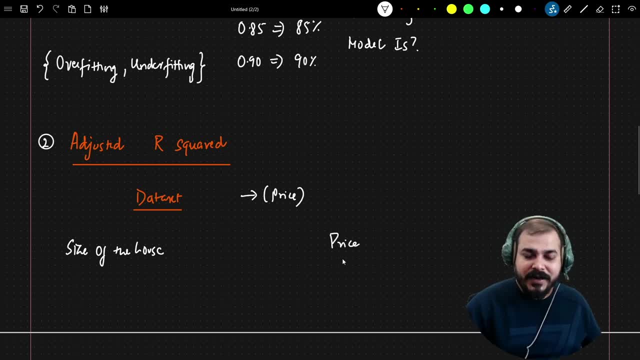 is called as size of the house. so i am definitely going to write price over here. now suppose if i have size of the house and the price of the house, as we know that as the size of the house, as the size of the house increases, increases, my price is also going to increase. so there is a direct. 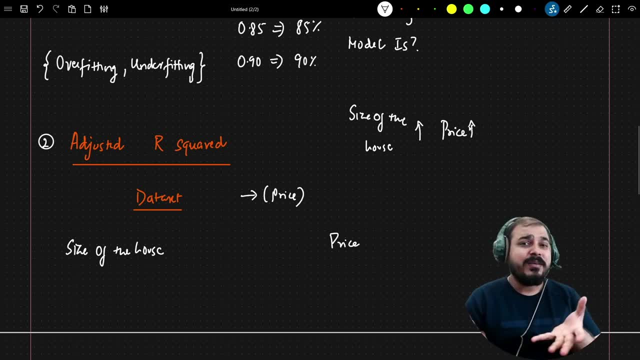 correlation between size of the house and price of the house- and this is usually happens in any, any state or any region- that you are probably seeing is staying right. the size of the house as it increases, the price also increases so, and similarly, when the size of the house decreases, 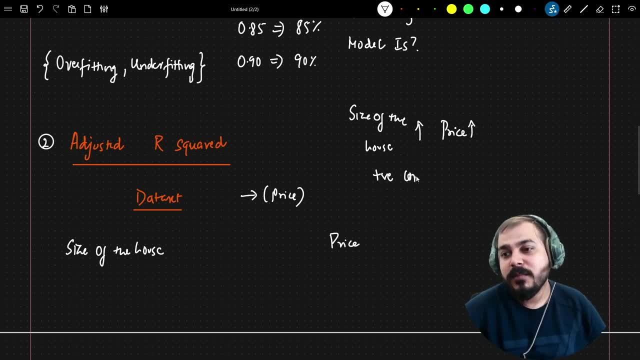 the price also decreases. so here we can definitely find something called as a positive correlation. right, positive correlation, a good positive correlation. so when we have, in this particular case, a good positive correlation, uh, then what happens? my r? squared value probably increases, right, let's say, this value basically increases. now let's say in this: 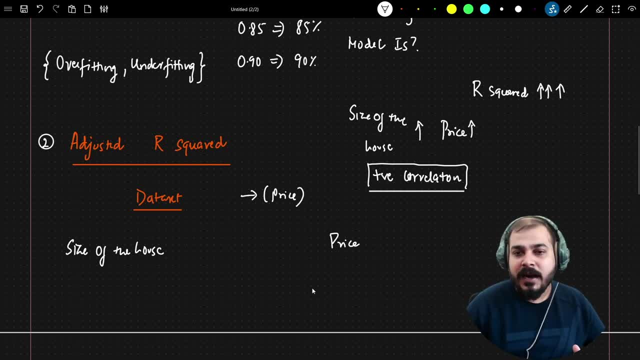 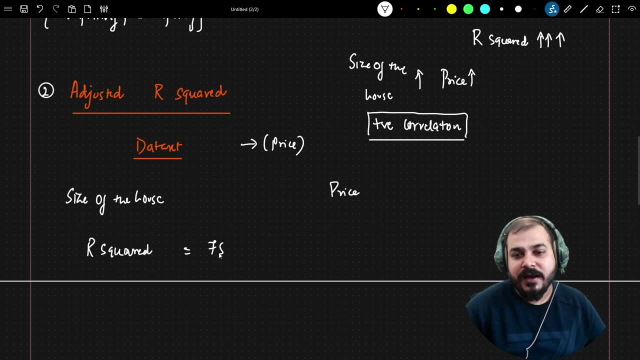 particular case, when i'm using these two features, my uh- and let's say that i have actually computed my r squared- my r squared value that was coming was somewhere around- uh, you know, 75 percent. let's say 75 percent is nothing but 0.75 with the help of the same formula. okay, let's say with the help. 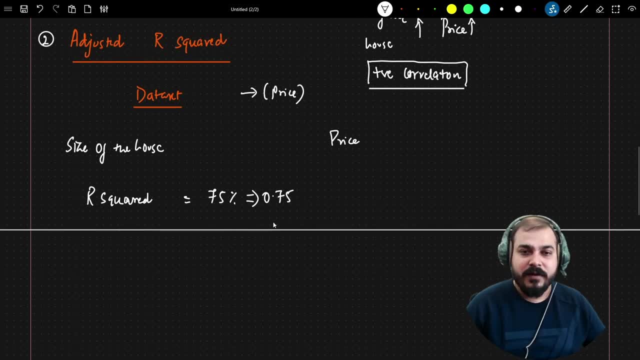 of this same formula that we have used over here, we got 0.75. now what happened is that, let's say, i included one more feature after i have included one more feature after i have included one more feature. the size of the house. i said number of bedrooms. now you know that as the number of bedrooms 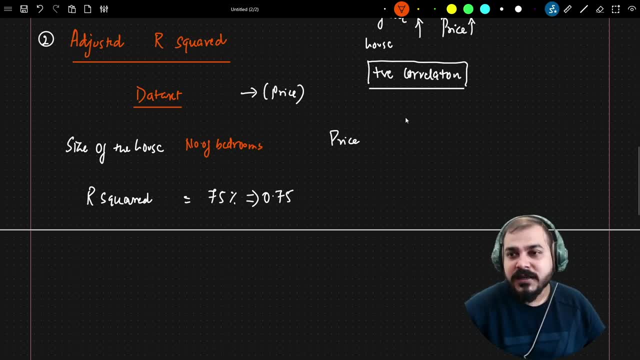 increases, right, the price is also going to increase. so from this i can definitely say, as my number of bedroom- and this is just a domain knowledge- right, when the number of bedroom increases, my price also is going to increase. so here also i can definitely see something called as: 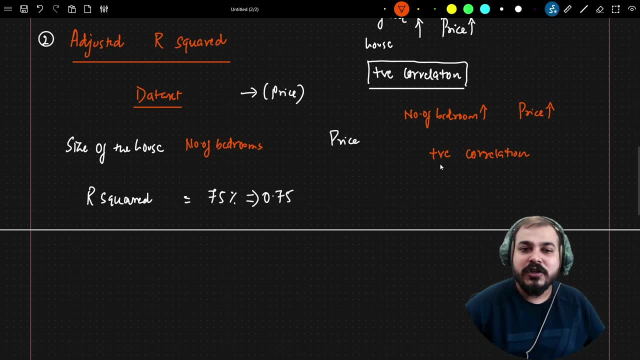 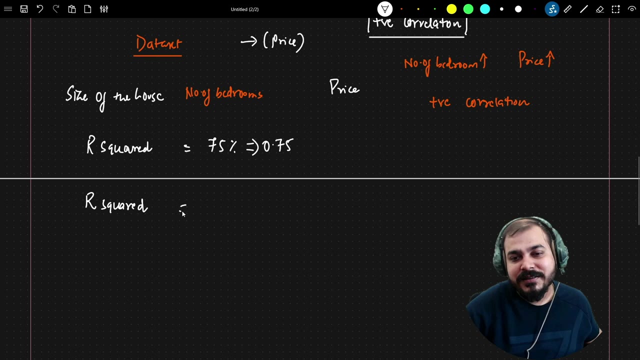 positive correlation, right. so when i'm actually seeing this positive correlation now, if i go and probably find out my r squared value again after i create my model and probably plot or get my best fit line and then apply this entire formula, okay, i am definitely going to see some increase. let's say here i'm just assuming that. 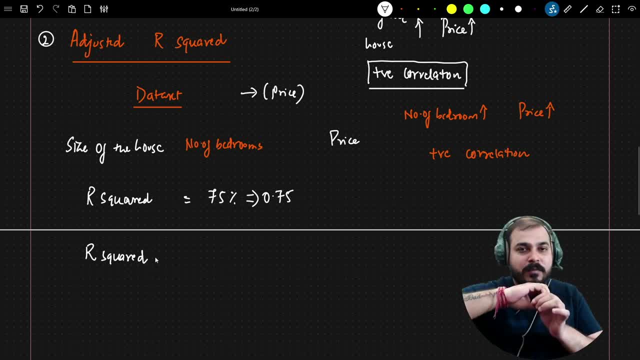 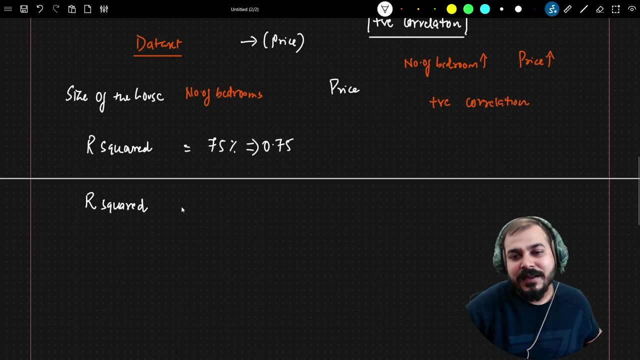 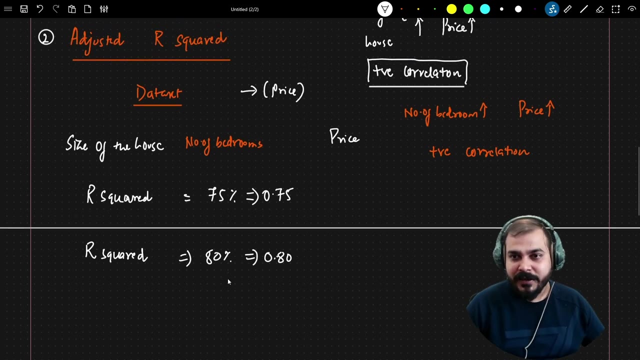 r squared value again, after i create my model and probably plot or get my best fit line and then apply this entire formula, okay, i am definitely going to see some increase. let's say here i'm just assuming that i got 80 percent, so this is nothing but 0.80. this is also perfectly fine now. similarly, when i try to add: 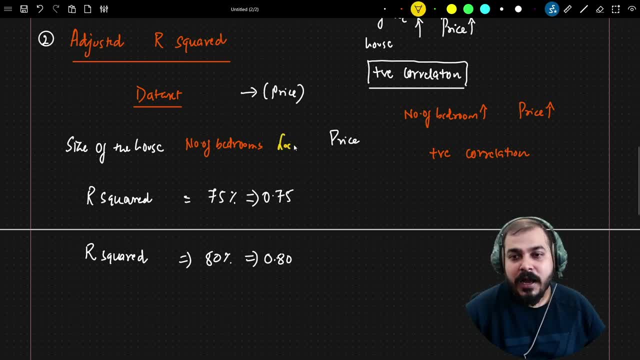 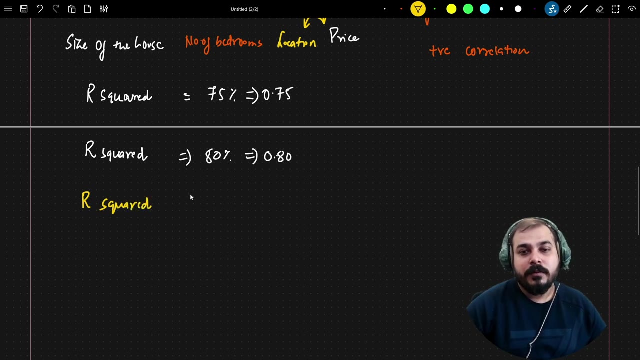 one more feature with, let's say, this particular feature is location, and we know that with respect to location also, it is more positively correlated with respect to price. okay, these two are more positively correlated, so there are again chances that my r squared value will definitely increase. okay, my r square value will become 85 percent. let's say i'm just assuming it has now increased. 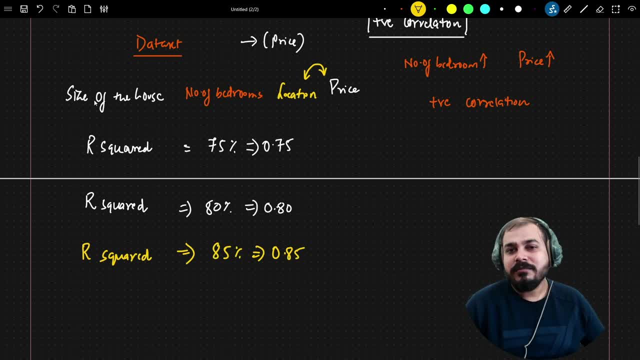 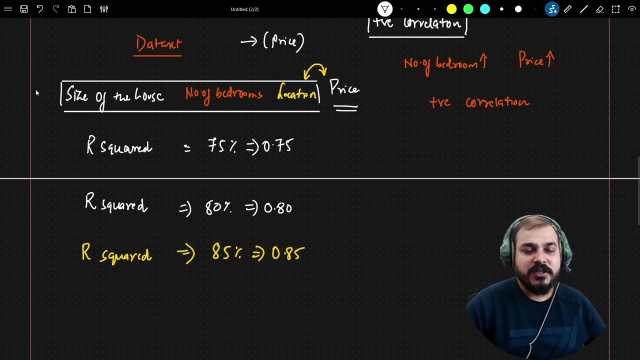 to 85 percent. now let's say that, okay, this many features i have, okay, this many perfect, so many independent features i have, and, uh, and this is my all my independent features and this is my dependent feature right now, let's say that i have added one more feature now, this specific feature, basically. 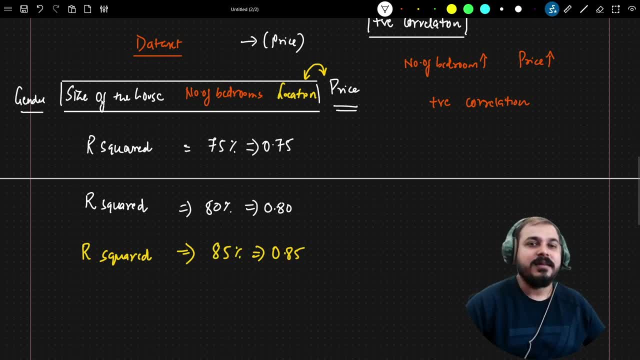 says that which gender are going to stay in this house? okay, whether they're, i'm just adding one feature. okay, that does not make any sense. okay, and obviously you know that if i consider gender with price, obviously just by common sense, there will be no correlation with respect to price right. 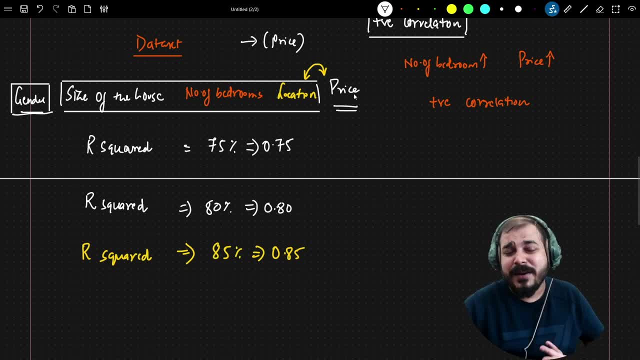 anyhow, no correlation. whoever gender stays over there, obviously price is not going to get affected, right? but if we add this particular feature which is not at all correlated with price, and again, if we try to probably solve this problem, which again in the future, i'll be showing you in, 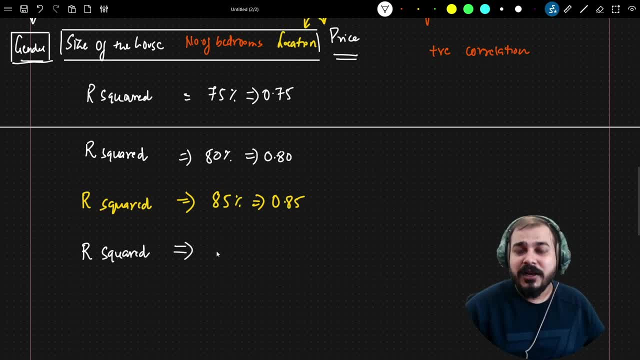 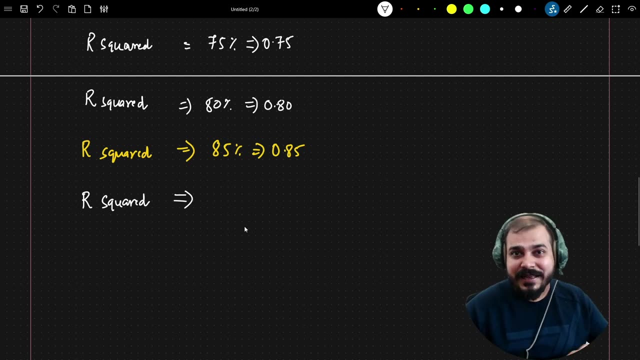 with the help of practical example. if i try to see the r squared value, even though these two variables, this input feature and this output feature, are not at all correlated, then also, since we are applying this particular r squared formula, there will be chances that this particular value will still increase, but it will not increase by a bigger value. so here you. 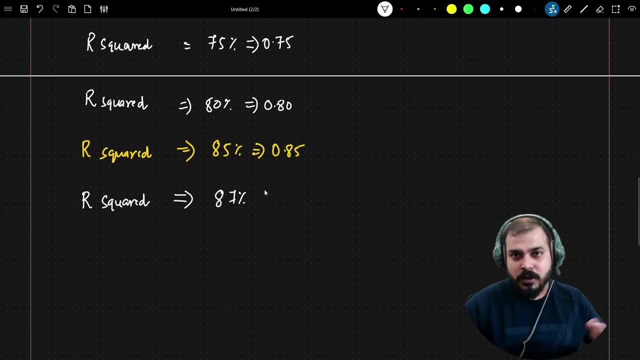 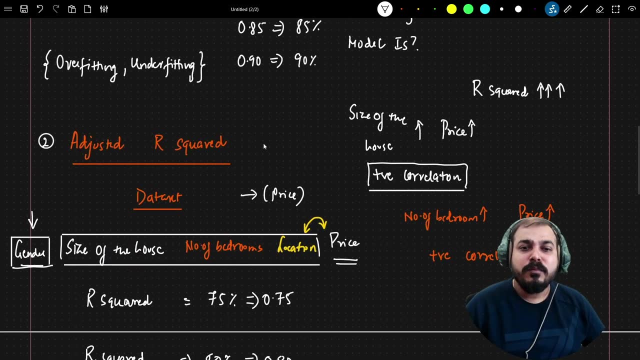 can see that i'm actually getting somewhere around 87 percent. let's say, okay, i'm just assuming two more percent. it got increased because the formula- it works in that specific way of r squared is that as more number of features you keep on adding, somehow the r squared value is going to increase. 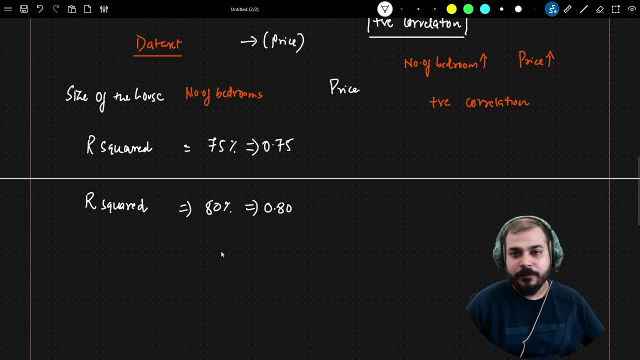 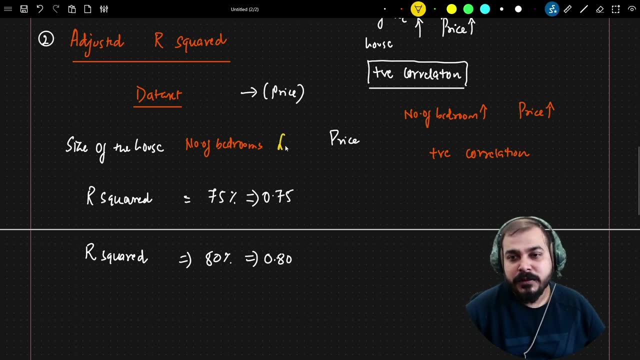 i got 80 accuracy, so this is nothing but 0.80. this is also perfectly fine now. similarly, when i try to add one more feature with, let's say, this particular feature is location and we know that with respect to location also, it is more positively correlated with respect to price. okay, this two up. 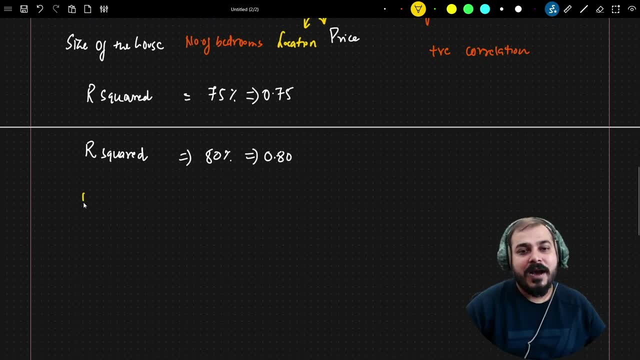 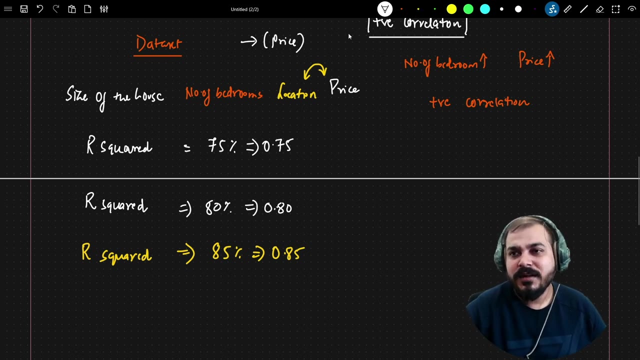 positively correlated. so there are again chances that my r squared value will definitely increase. okay, my r square value will become 85 percent. let's say i'm just assuming it has now increased to 85 percent. now let's say that, okay, this many features i have. okay, this many perfect, so many. 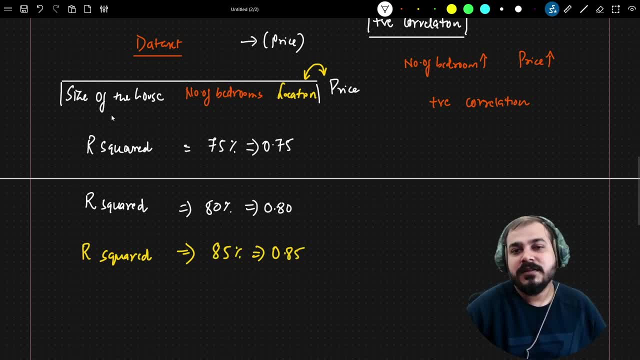 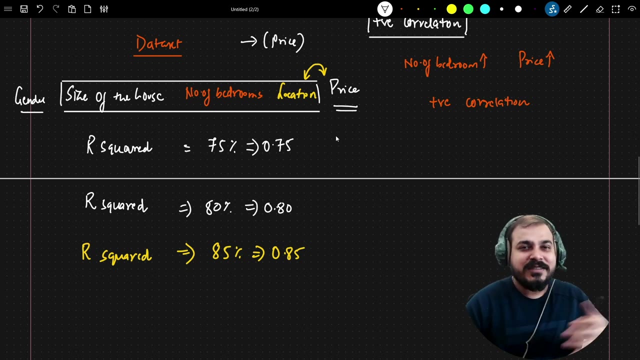 independent features. i have and, uh, and this is my all my independent features and this is my dependent feature right now. let's say that i have added one more feature. now, this specific feature basically says that which gender are going to stay in this house. okay, whether they're, i'm just adding. 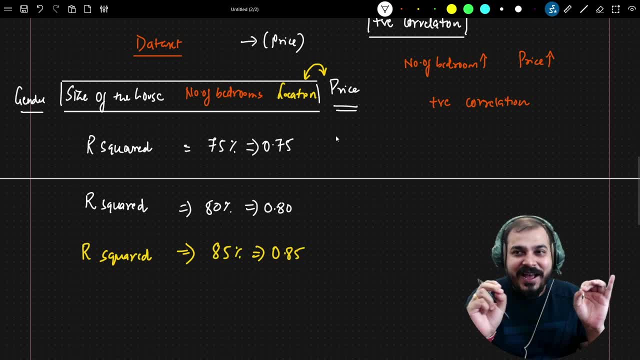 one feature. okay, that does not make any sense. okay, and obviously you know that if i consider gender with price, obviously, just by common sense, there will be no correlation with respect to price, right, anyhow, no correlation. whoever gender stays over there, obviously price is not going to get affected. 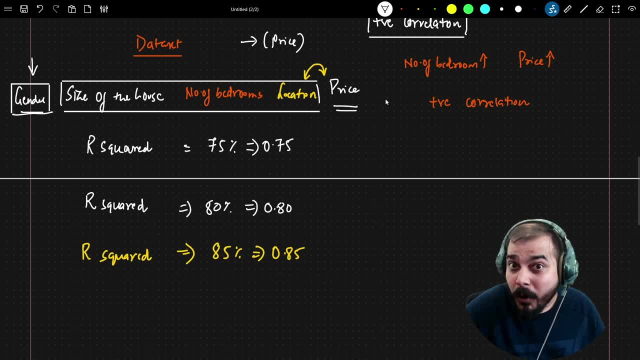 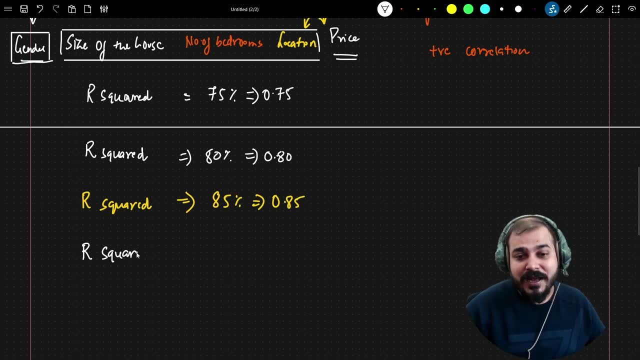 right. but if we add this particular feature which is not at all correlated with price, and again, if, if we try to probably solve this problem which, again in the future, i'll be showing you in with the help of practical example- if i try to see the r squared value, even though these two variables 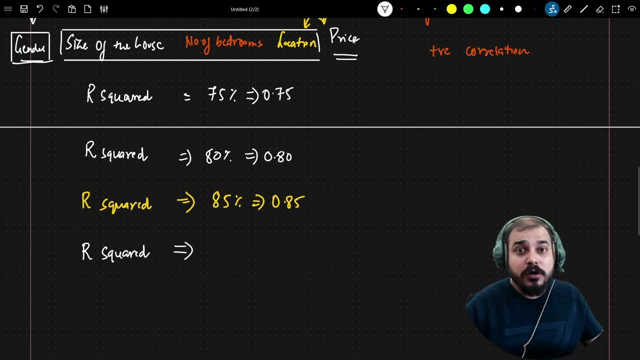 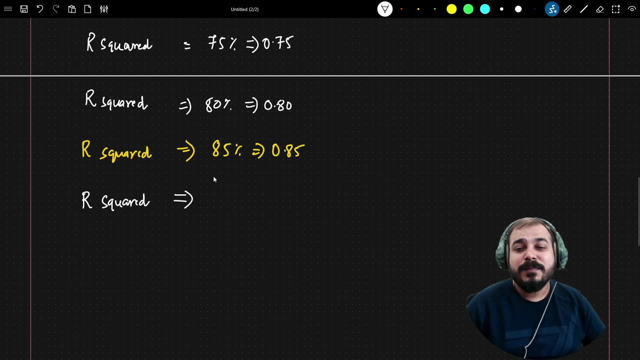 this input feature and this output feature are not at all correlated. then also, since we are applying this particular r squared formula, there will be chances that this particular value will still increase, but it will not increase by a bigger value. so here you can see that i'm actually 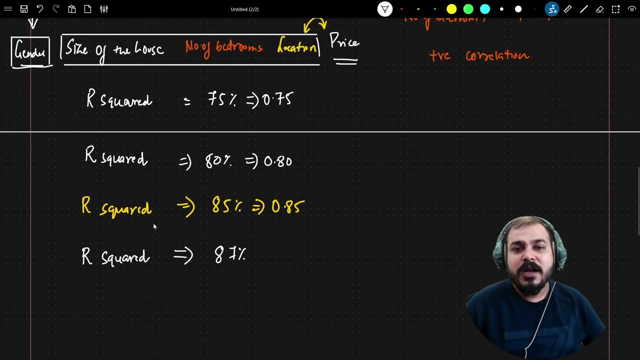 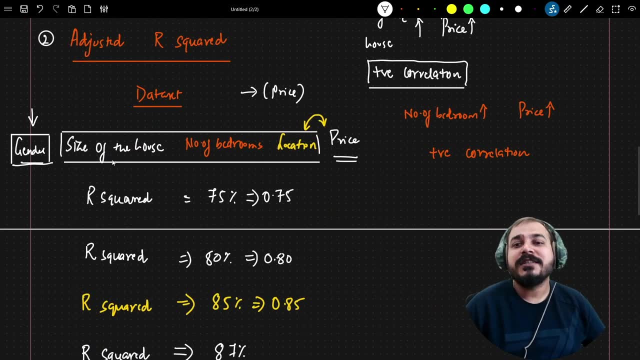 getting somewhere around 87 percent. let's say, okay, i'm just assuming two more percent. it got increased because the formula- it works in that specific way- of r squared is that as more number of features you keep on adding, somehow the r squared value is going to increase. okay, and 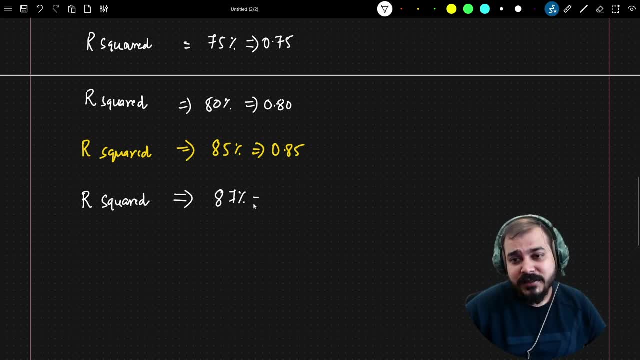 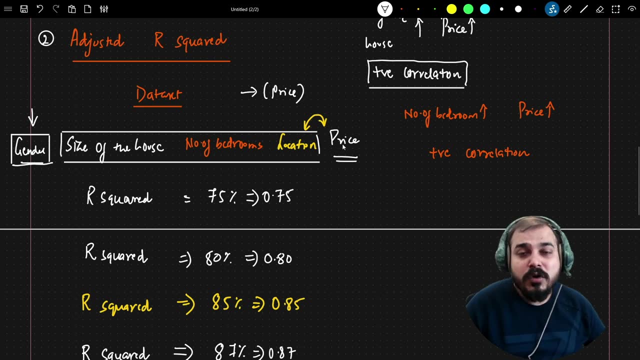 okay, and these all things i'll show you in practical also, guys. so let's say this become 0.87. but now there is some kind of problem. even though this particular feature is not at all correlated with price, here you can definitely see that my r squared value is increasing. okay, i did not prove 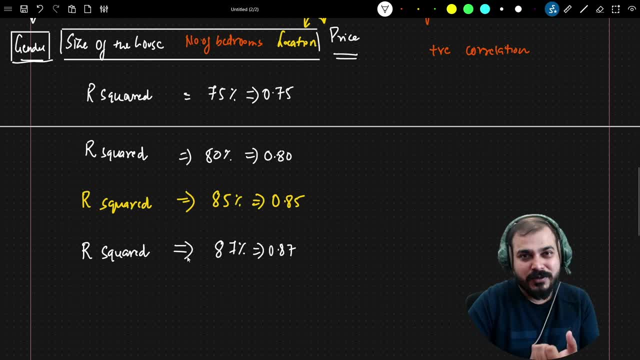 it practically yet, because i'll do the practical and show you. uh, with respect to this particular problem statement also: right. so in this case, the r squared, you can see that, even though this and this feature are not at all correlated, still it is basically increasing, right? so this is the problem with respect to r squared, right? so this is the problem. 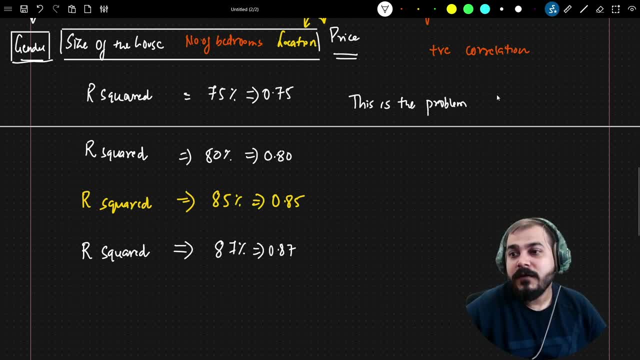 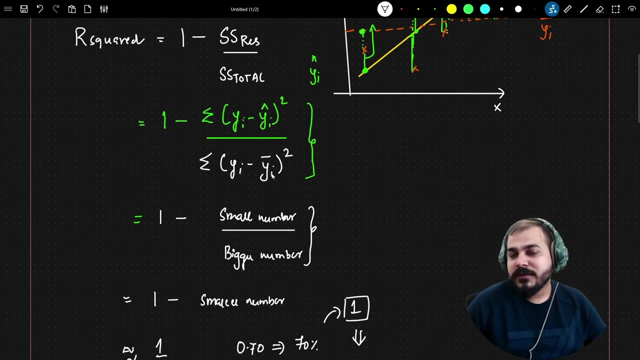 with respect to r squared problem of r squared, even though you don't have a feature that is directly correlated with the output feature, then also this particular value increases, since the formula is in that specific way. we are just trying to find out the difference between residual and difference between the mean of which we basically say it as ss of total. now, in order, 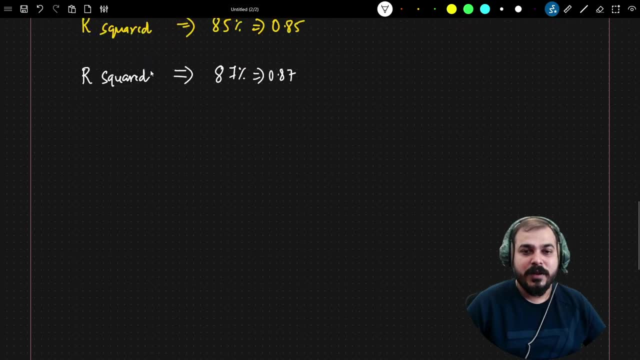 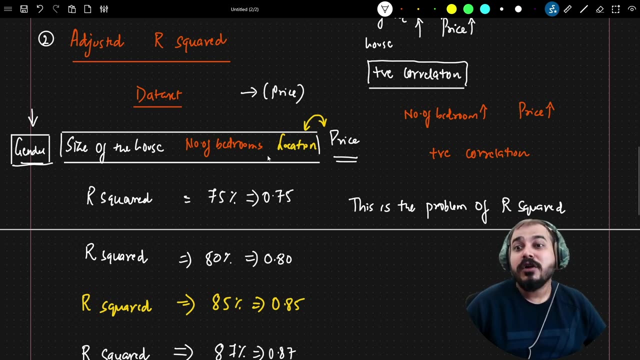 to prevent this, we basically use something called as adjusted r squared. now, in adjusted r squared, what it does is that it penalizes with respect to every feature that are not correlated with the output feature. okay, so this is what amazing thing basically happens with the existed r squared. now, in order to define, uh, the adjusted r squared, we 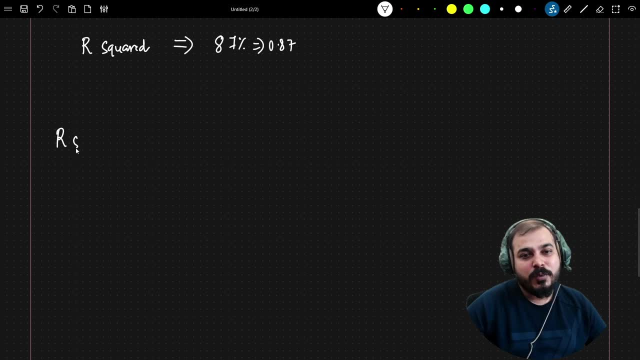 basically use a very simple formula. so i am basically using r squared or the adjusted r squared. so let me write down the formula over here and again. uh, you do not know how. the formula is not at all important, but instead we should directly use this kind of performance matrix. 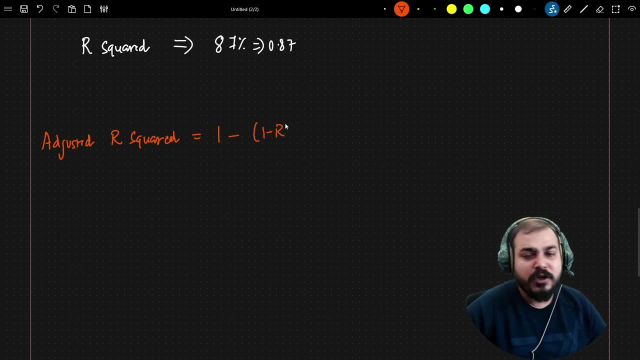 so it is nothing but one minus one minus r, squared, and i'll talk about each and every term multiplied by n minus one, divided by n minus p minus one. okay, now let me talk about what is this n, what is this p? and all right, so n is nothing, but we basically say number of data points. 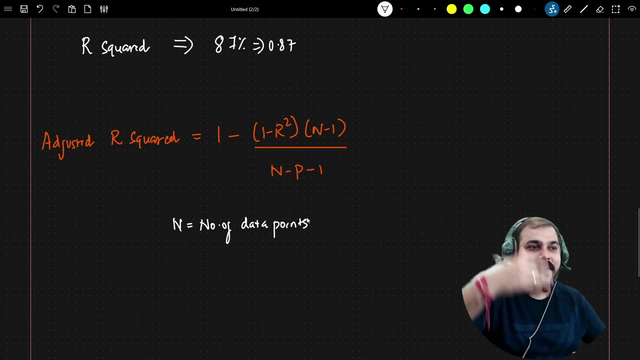 okay, number of data points. so that's the number of data points. that's the number of data points basically means in our data set: how many data points are actually there. okay, and p basically indicates number of independent features: number of independent features that we are using now, guys. 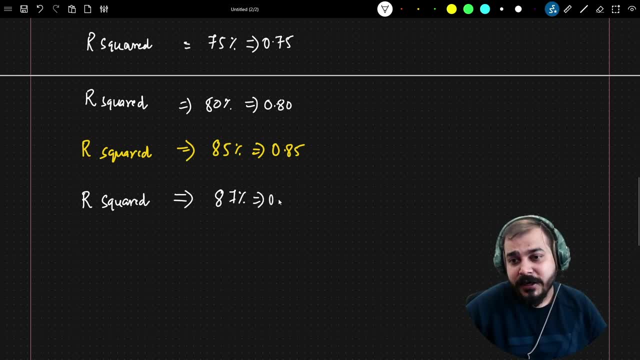 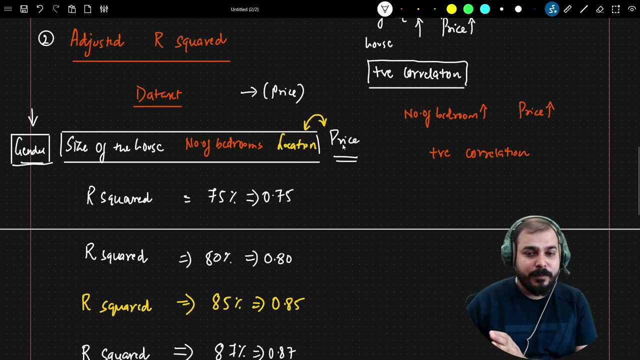 these all things i'll show you in practical also, guys. so let's say, this become 0.87. but now there is some kind of problem. even though this particular feature is not at all correlated with price here you can definitely see that my r squared value is increasing. okay. 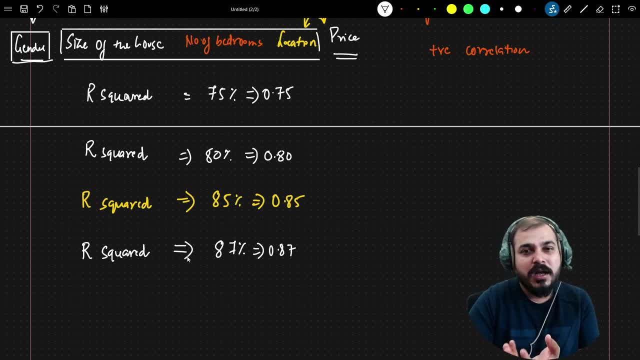 i just want to show you that i'm actually getting somewhere around 87 percent. let's say, not prove it practically yet, because i'll do the practical and show you. uh, with respect to this particular problem statement also: right, so in this case the r squared. you can see that even. 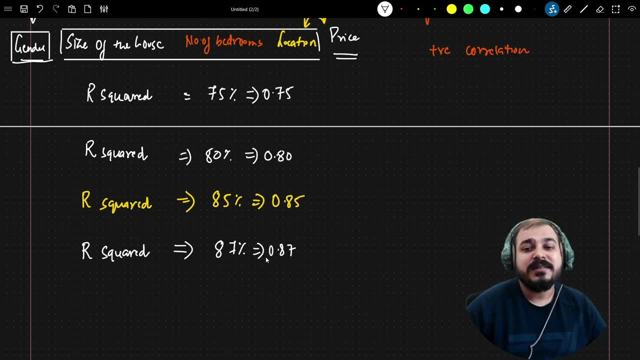 though this and this feature are not at all correlated. still, it is basically increasing, right? so this is the problem with respect to r squared, right? so this is the problem with respect to r squared, problem of r squared even though you don't have a feature that is. 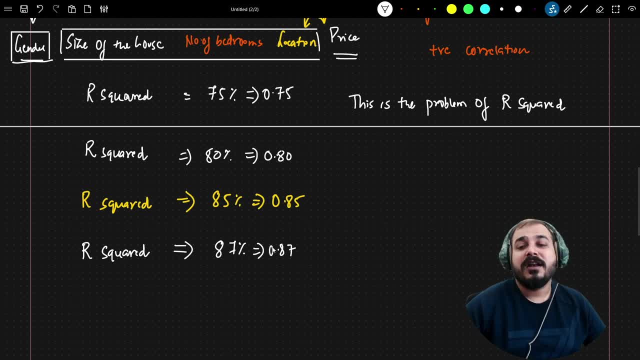 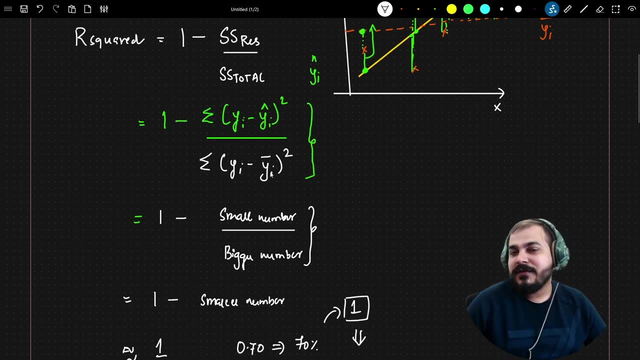 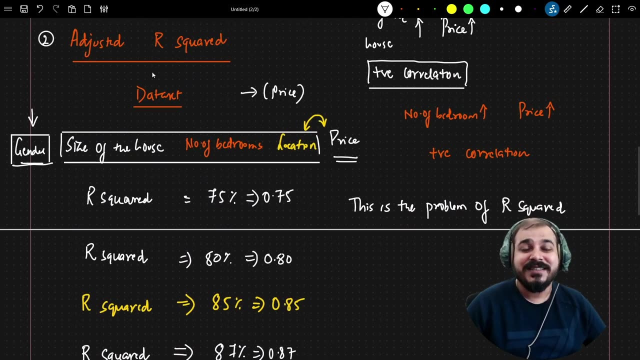 directly correlated with the output feature, then also this particular value increases since, uh, the formula is in that specific way, we are just trying to find out the difference between residual and difference between the mean, of which we basically say it as ss of total. now, in order to prevent this, we basically use something called as adjusted r square. now, in adjusted r. 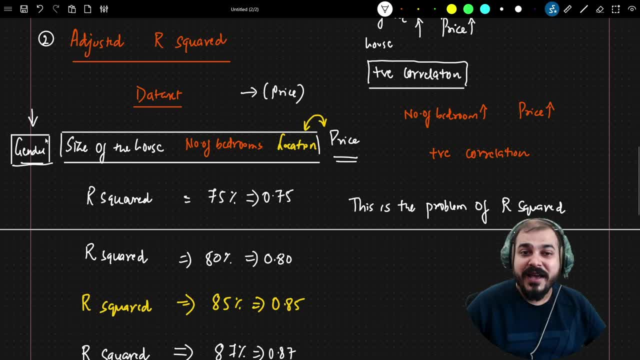 square. what it does is that it penalizes with respect to every feature that are not correlated with the output feature. okay, so this is what amazing thing basically happens with the existed r square. now, in order to define, uh, the existing r squared, we basically use something called the. 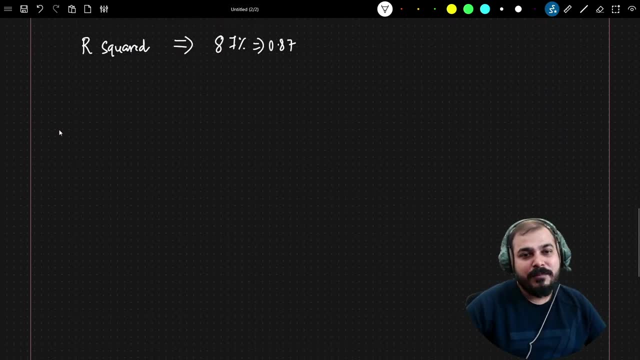 adjusted r square. we basically use a very simple formula. so i am basically using r squared or the adjusted r squared. so let me write down the formula over here and again. uh, you do not know how the formula is getting derived, guys. that is not at all important, but instead we should directly. 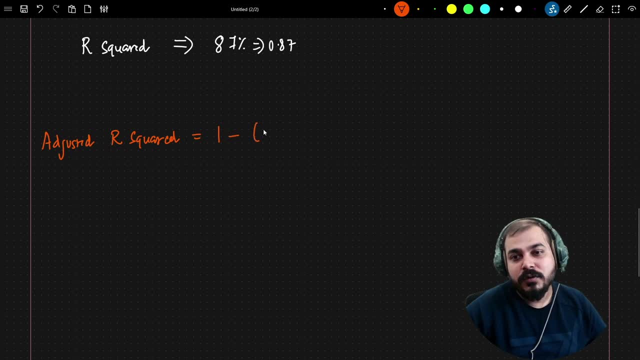 use this kind of performance matrix. so it is nothing but one minus one minus r squared, and i'll talk about each and every term multiplied by n minus one, divided by n minus p minus one. okay, now let me talk about what is this n, what is this p? and all right. so n is nothing but. 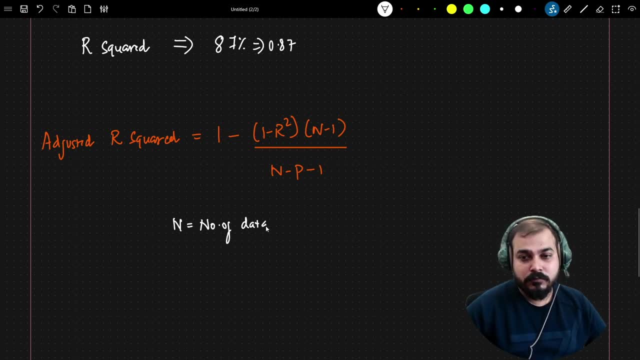 we basically say number of data points: okay, number of data points. so that basically means, in our data set, how many data points are actually there? okay, and p basically indicates number of independent features. number of independent features that we are using. now, guys, whatever formula that we have written over here with respect to the adjusted r square one- amazing. 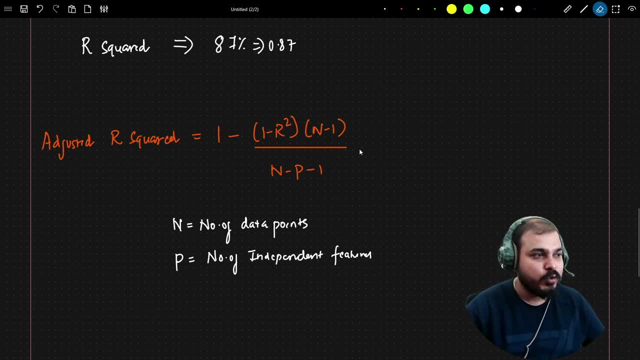 whatever formula that we have written away with respect to the adjusted r squared, one amazing thing that you will be finding in this and later on, when we do the practical implementation. that thing will be clearly visible to you. so let me just note it down over here and in the later. 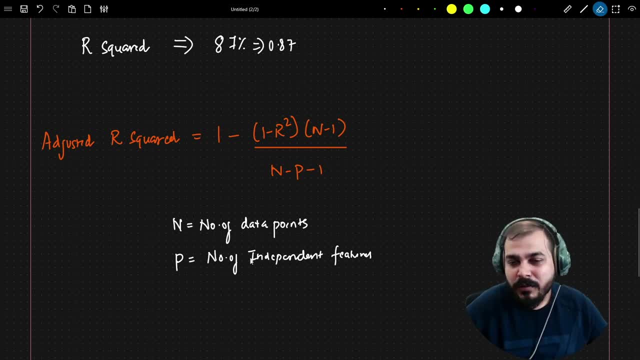 stages in the practical part. i will try to show it to you now. n basically means number of data points. p basically means number of independent feature. let's say, initially my p value is something like two. so this basically indicates that, let's say my number of independent features. 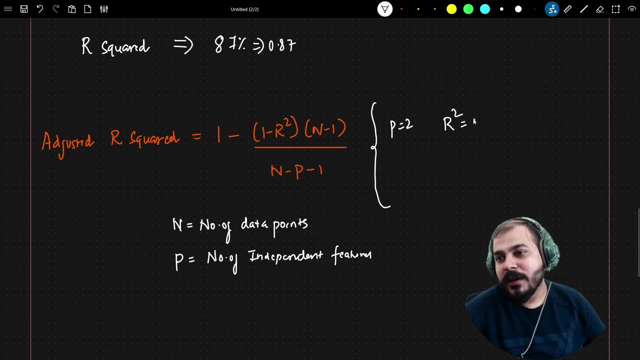 are two in this case. let's say my r squared is 90- i'm just assuming, i'm just giving you a hypothetical scenario- right? if my r square value is 90, then if i try to apply the same formula with respect to r square adjusted, then here you'll be, seeing that i will be getting less than this particular r square value. so here, 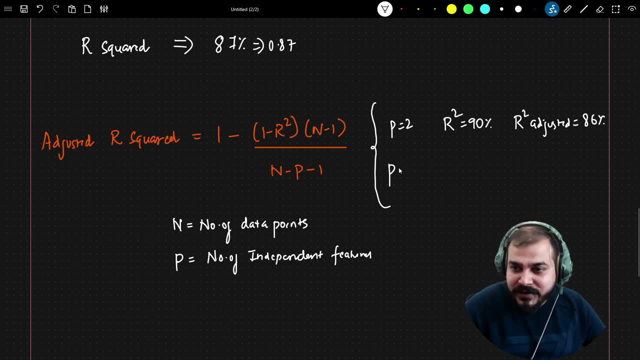 let's say i'm getting 86. okay, now, as soon as i increase p value, then obviously you know that we have seen that the r square value will increase. okay, let's say the r square value has got 92 and let's say that additional one feature that we have added, the independent feature, is not at all. 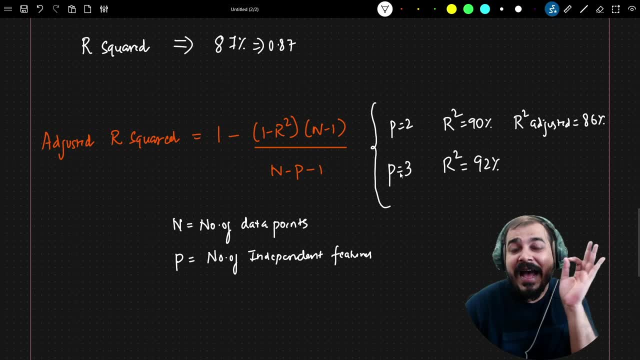 correlated- okay, not at all correlated- or it does not have a direct impact on that specific output feature. at that point of time, you will be seeing that the r square adjusted value will get reduced. it will be somewhere around 82- 83. it will be less than the previous one, that is, less than the 86 percent. 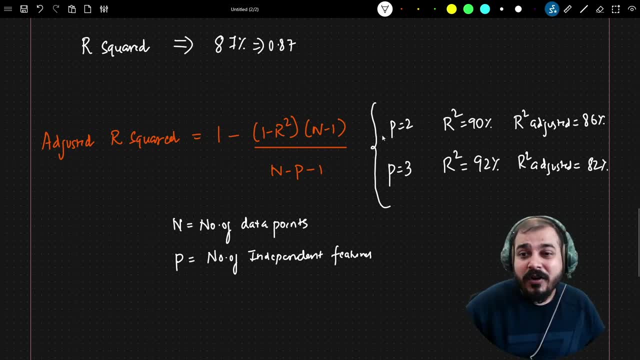 here. i'm just giving you a hypothetical number. okay, this kind of scenarios you will be able to see with the help of adjusted r square. suppose, if the additional independent feature that i have added is directly proportional to the output feature, one thing that you will be able to. 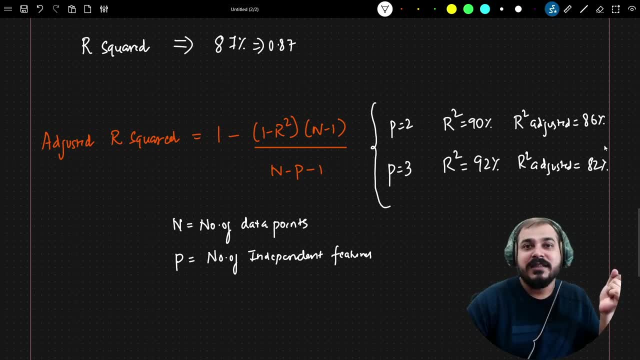 find out that it will increase and it will be greater than this 86 percent. if it is not at all correlated, then it is going to decrease. this is the assumptions i'm making it right now. okay, later on, when i try to show you with respect to the practical, uh, you know you will be able to. 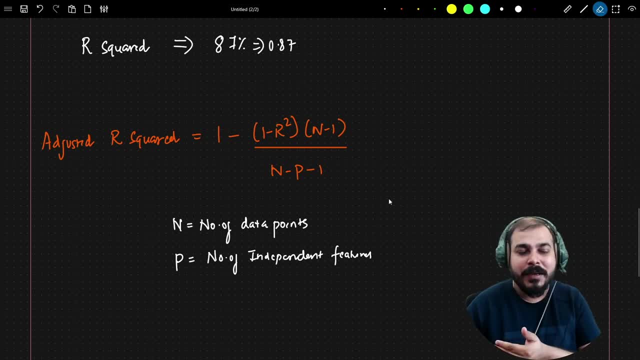 thing that you will be finding in this and later on, when we do the practical implementation, that thing will be clearly visible to you. so let me just note it down over here and in the later stages, in the practical part, i will try to show it to you now. n basically means number of data points. 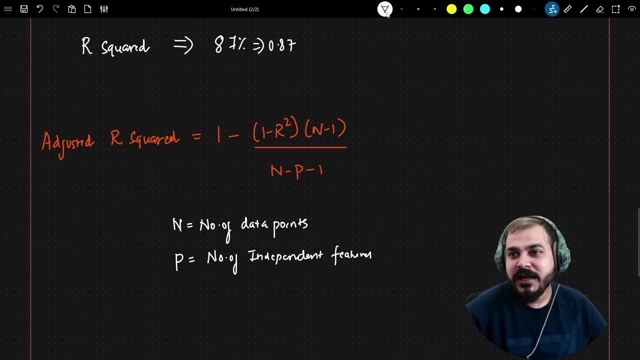 p basically means number of independent feature. let's say, initially my p value is something like two. so this basically indicates that let's say, my number of independent features are two in this case. let's say my r squared is 90%. i'm just assuming, i'm just giving you a. 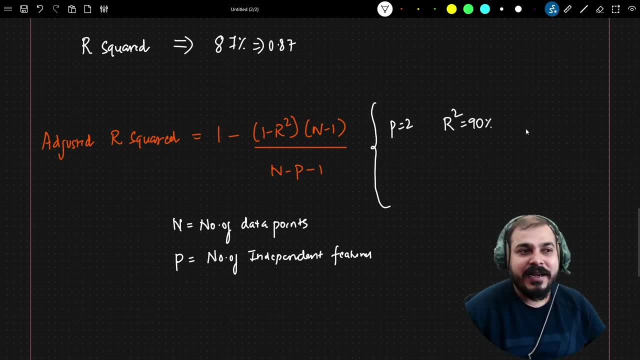 hypothetical scenario. right, if my r square value is 90, then if i try to apply the same formula with respect to r square adjusted, then here you will be seeing that i will be getting less than this particular r square value. so here, let's say, i'm getting 86%. okay, now, as soon as i increase p value, 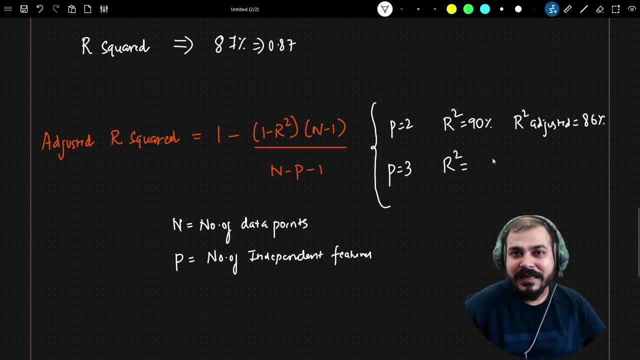 then obviously you know that we have seen that the r square value will increase. okay, let's say the r square value has became 90, so that's very important. let's say that the r square value is increasing, got 92 percent. and let's say that additional one feature that we have added, the independent 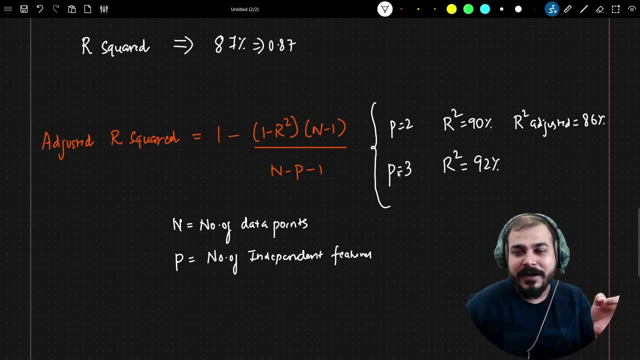 feature is not at all correlated. okay, not at all correlated, or it does not have a direct impact on that specific output feature. at that point of time, you will be seeing that the r square adjusted value will get reduced. it will be somewhere around 82- 83. it will be less than. 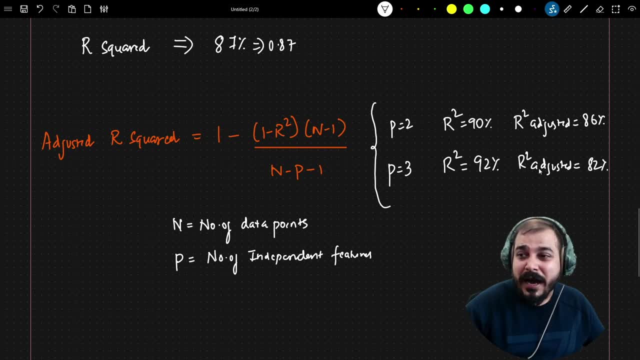 the previous one, that is, less than the 86 percent here i'm just giving you a hypothetical number. okay, this kind of scenarios you will be able to see with the help of adjusted r square. suppose if the additional independent feature that i have added is directly proportional to the output. 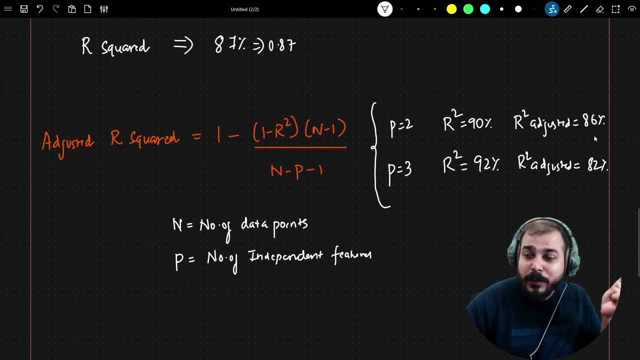 feature one thing that you will be able to find out: that it will increase and it will be greater than this 86 percent. if it is not at all correlated, then it is going to decrease. this is the assumptions i'm making it right now. okay, later on, when i try to show you with respect to the practical, 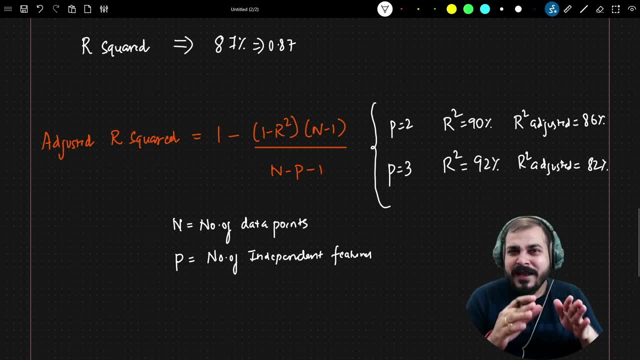 you know you will be able to find it out. you know i may you know you will be able to find it out. you know i may. you know you will be able to find it out. you know i may. i guess, like you may be thinking: okay, krish, how did this specific thing happen? just understand.